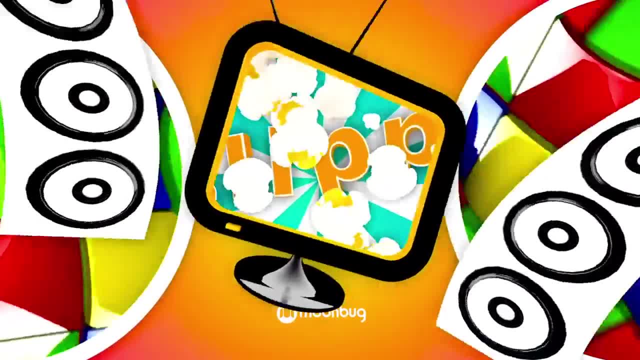 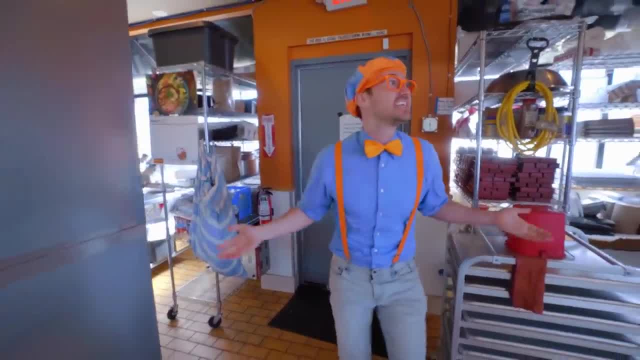 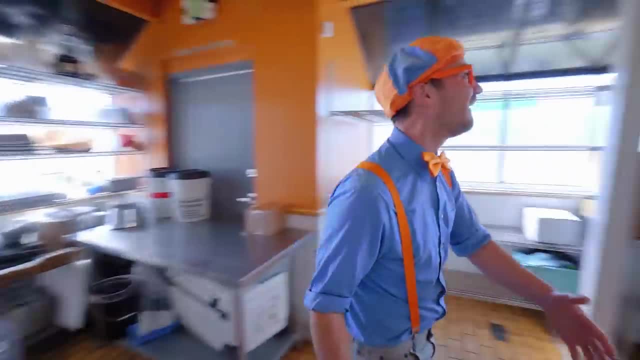 So much to learn about. it'll make you want to shout: Blippi, Hello, It's me Blippi, and today I'm at Petey Bakery in Seattle, Washington. Whoa, look at this place. Oh, it's so cool. 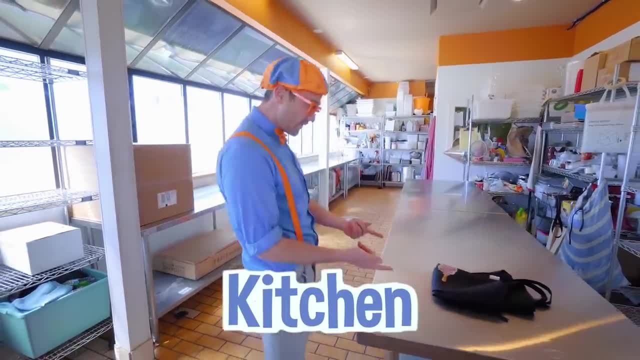 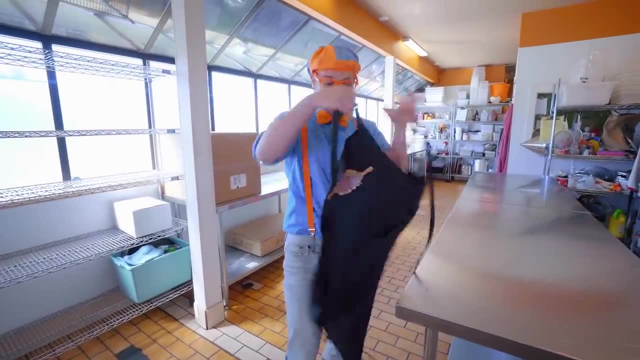 Yeah, we're in the back. Yeah, this is called a kitchen. Oh, and look at what it is. Wow, Look at it. Oh, wow, This is an apron. Ooh, check it out. Look at those flowers. 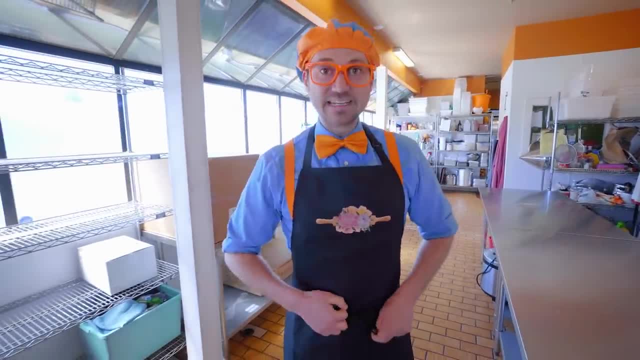 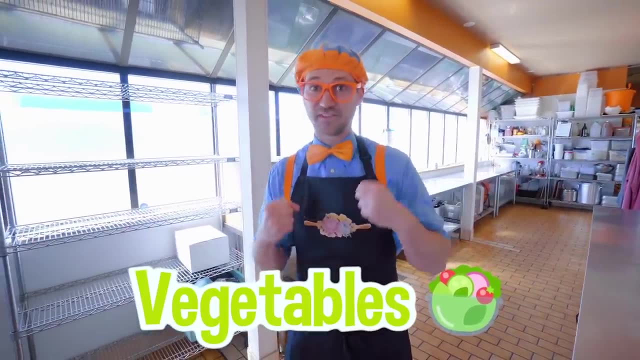 Yeah, this apron is going to help keep me nice and clean when I bake. Yep, I sure ate a lot of vegetables today. Yep, and now that I ate a bunch of healthy food, we can have something yummy and sweet. I am so excited. Let's go. 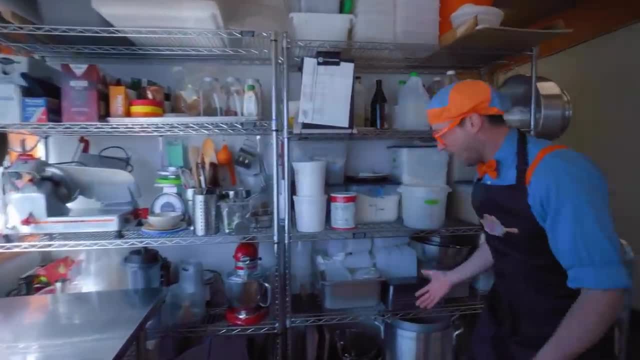 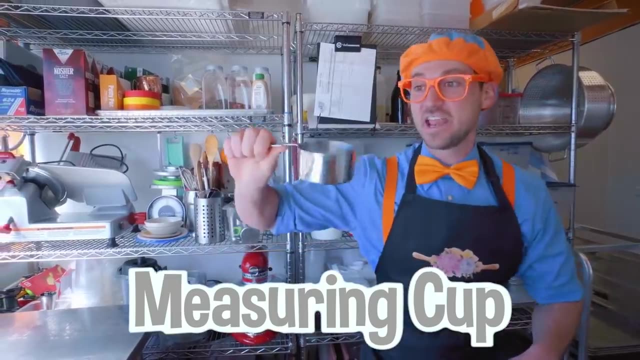 Wow, Wow. Look at this place- Whoa, there's so many cool things. Yeah, like a measuring cup. Yeah, you can put things in there and then know how much of an ingredient you have exactly in this measuring cup- Whoa. 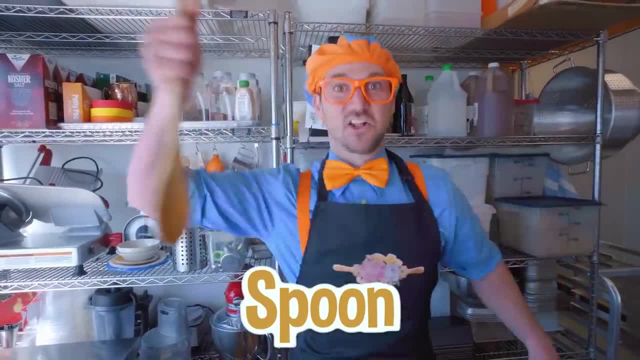 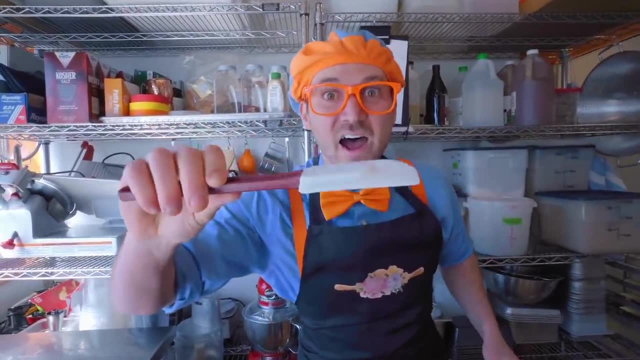 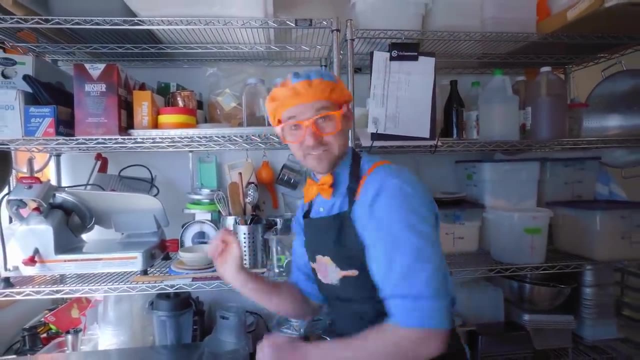 Or a giant spoon, Whoa. You can stir a lot of stuff with that Whoa, Whoa. And look at this: Yeah, a spatula Boing. That's so cool. Okay, let's set it right there for now. 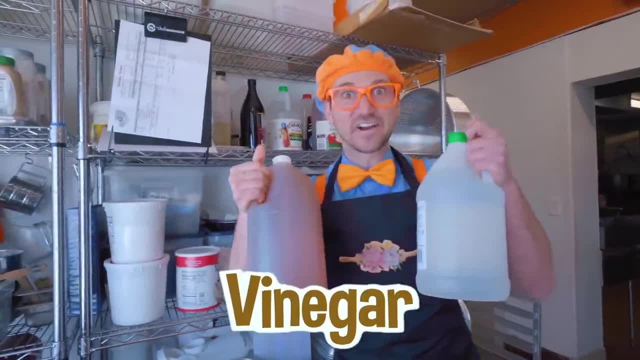 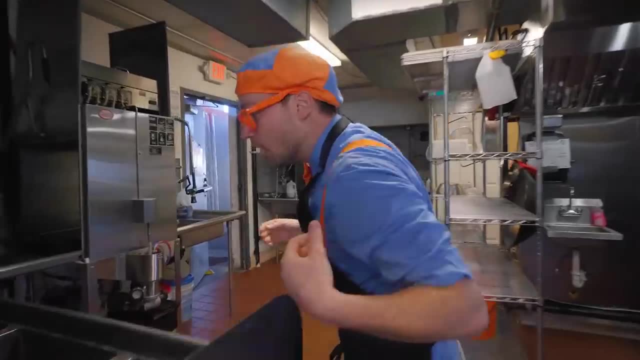 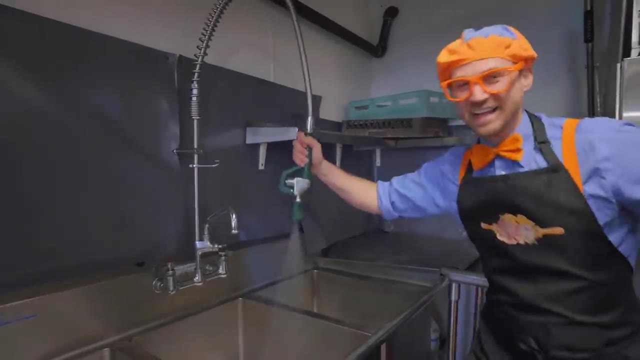 Whoa, Looks like we have some vinegar. Yum, Okay, there we go. Wow, come on. Whoa, A giant sink. Woohoo, Yeah, This is where I clean a lot of dishes, Woohoo. 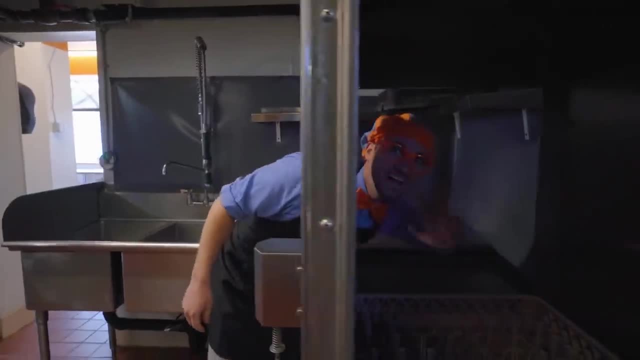 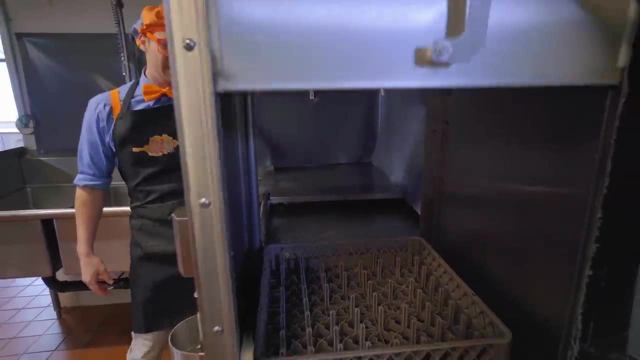 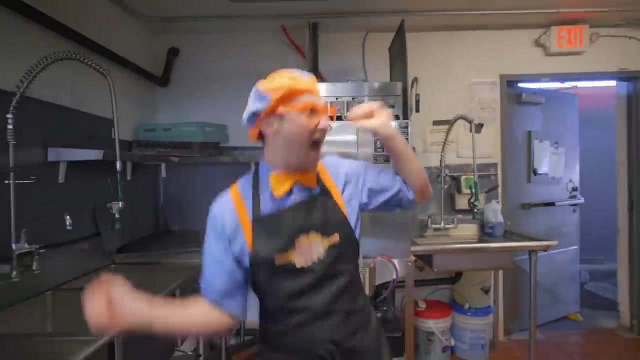 Oh, speaking of cleaning dishes, Whoa, Hello, Look, this is a dishwasher. You put a lot of dirty dishes right here and then you close it down. Yeah, That is awesome. Woohoo, Whoa, check it out. 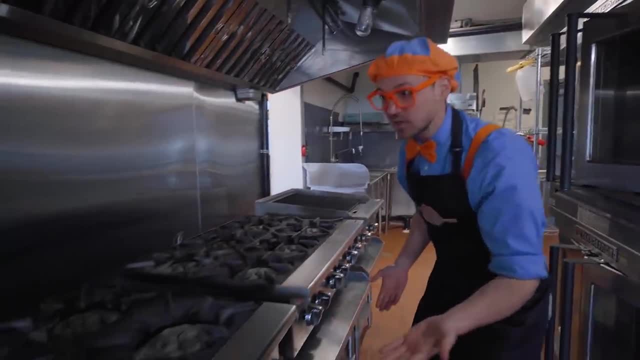 This is a stove top. Whoa, you can cook so much food right here. Whoa, there's so many stove tops. Whoa, do you see the little frying pan behind that? Whoa, this is a large frying pan. 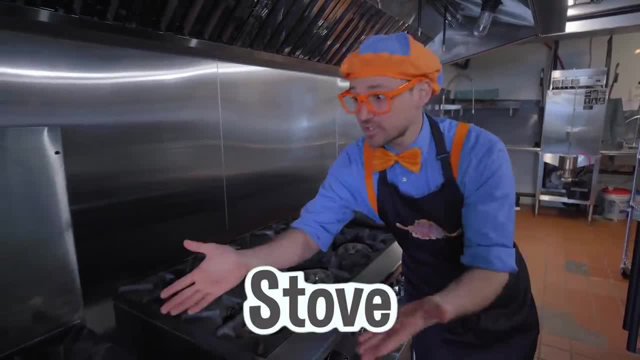 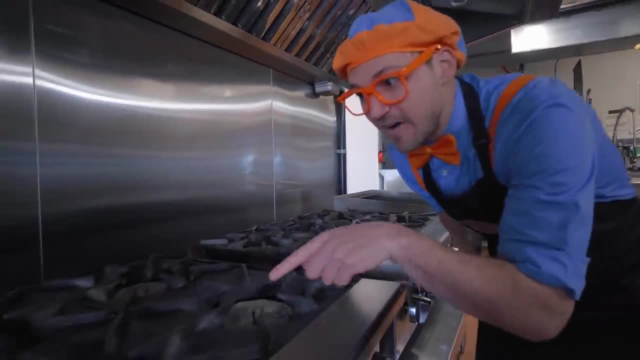 I love that. It's a lot of food. It's a lot of stuff. Wow, Whoa. Now let's see the kitchen. Whoa, look at that, Whoa, Look at that. Wow, little fire right there. Yeah, this is not a toy. You need to be very careful when you're cooking. 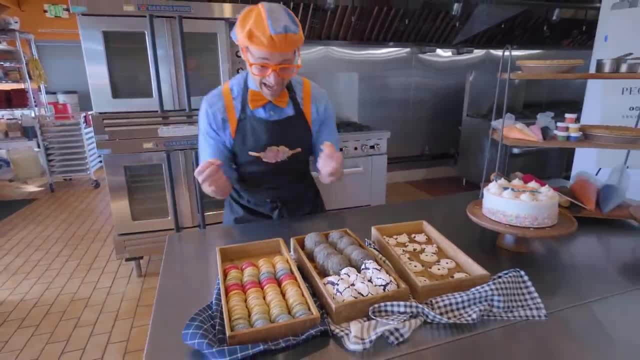 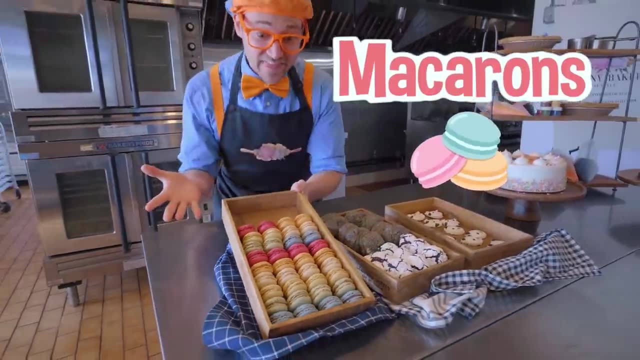 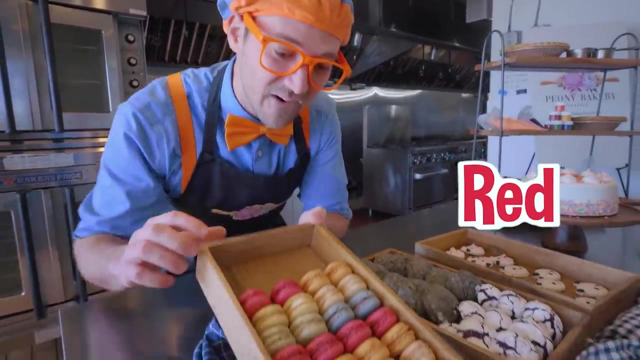 Whoa, Yum. Yeah. Look at these sweet treats. Wow, These are macarons and they look so yummy. Look at this one. This one is the color red Whoa. Looks like we have some green and some blue. 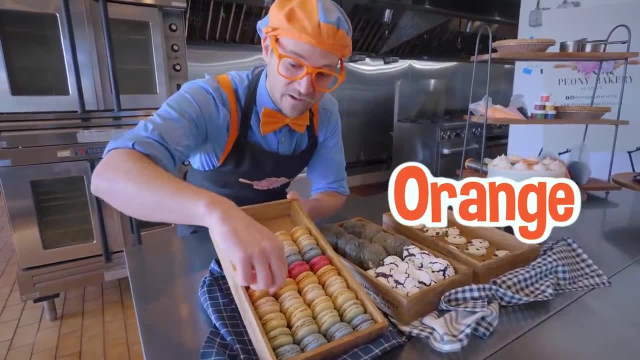 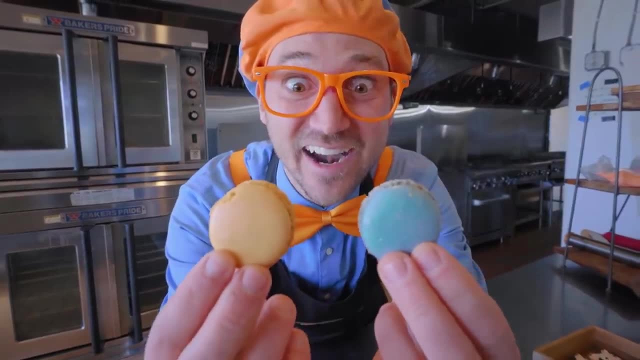 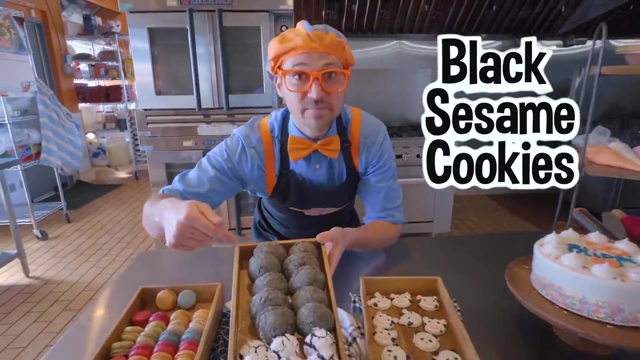 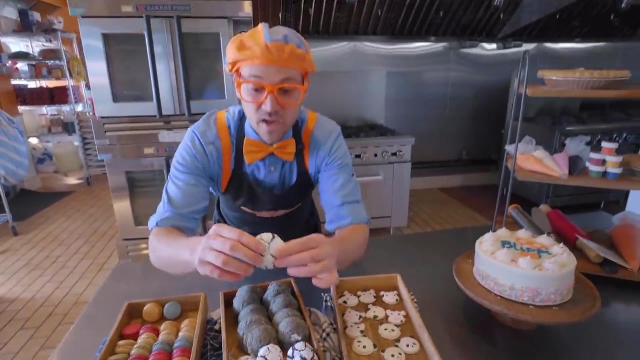 and some orange: Whoa. Look, I'll grab an orange and a blue, My two favorite colors. Ah, I'll eat these later. Whoa, We have some black sesame cookies- Yum. Whoa. And some ube cookies: Yum, Check these out. Open these up. Wow, What color is that? 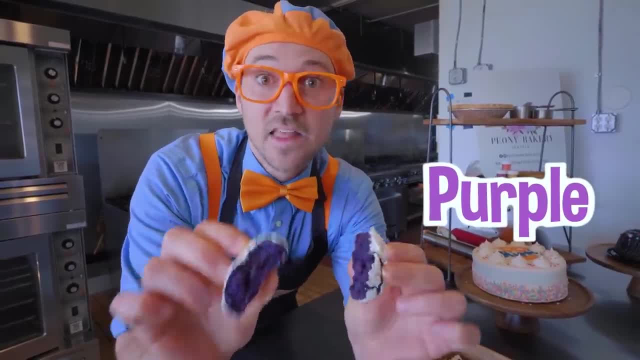 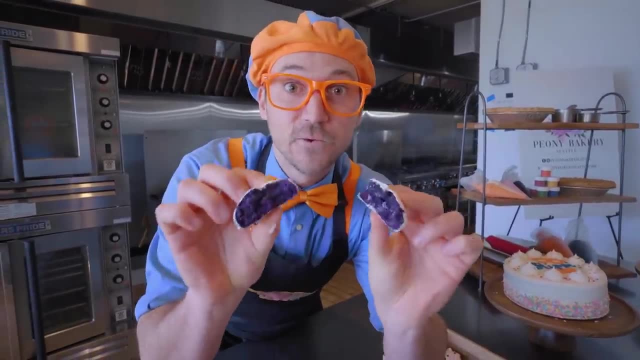 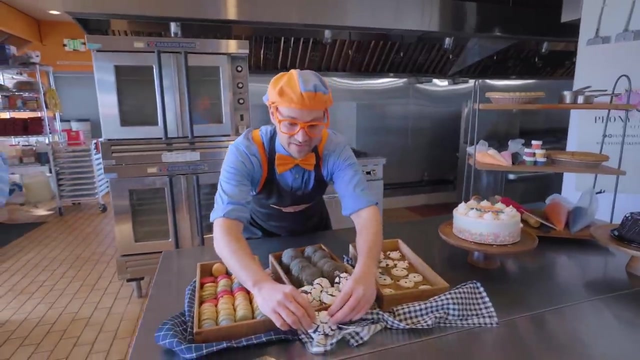 Yeah, the color purple. Yeah, there's no food coloring in this. That, yeah, that is the color of the food that was added into this cookie. That's so cool. Okay, we'll put that right there for me to eat later. 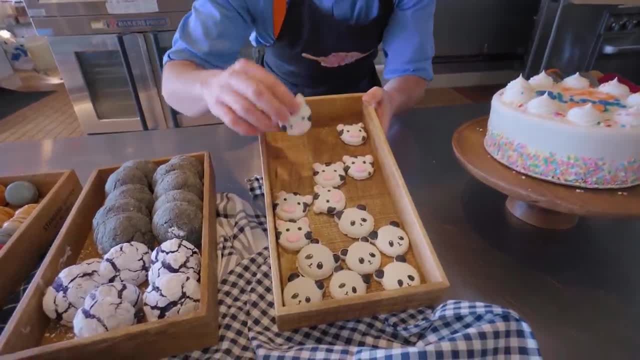 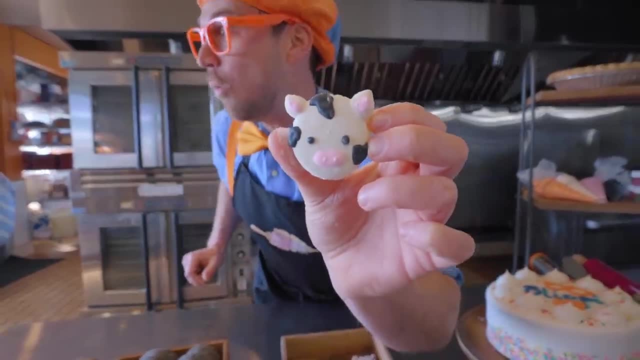 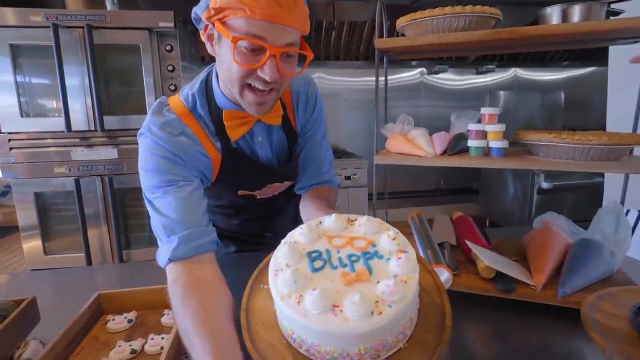 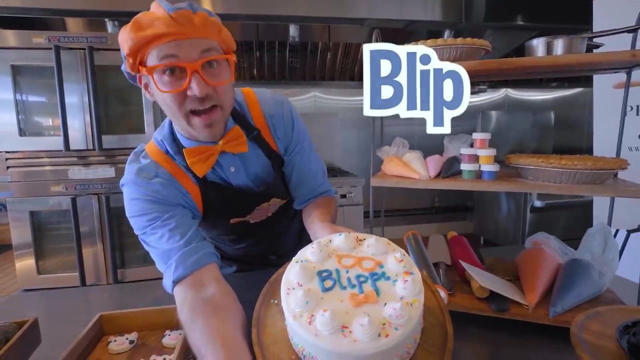 Whoa, Look at these cute things. Looks like. What animal is that? Yeah, Moo Moo. Yeah, A cow. Ooh, A vanilla cake. Yeah, Blippi, Party Cake. Will you spell my name with me? B-L-I-P-P-I. 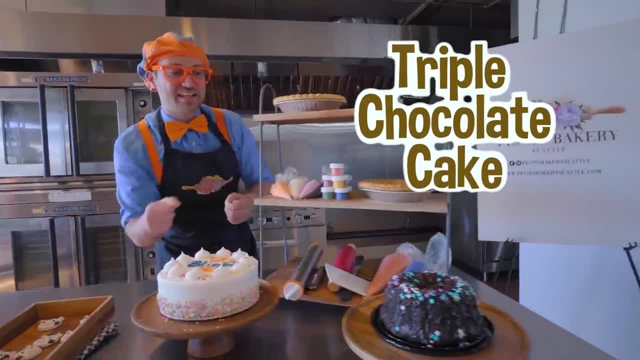 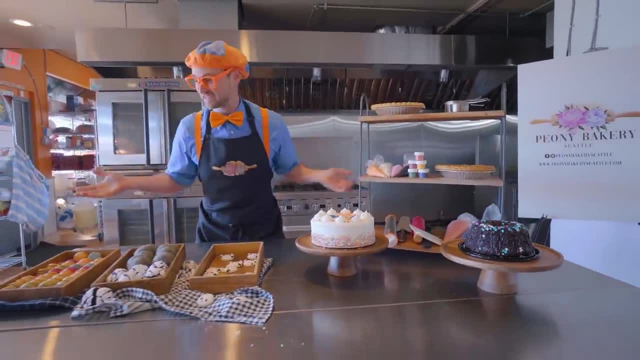 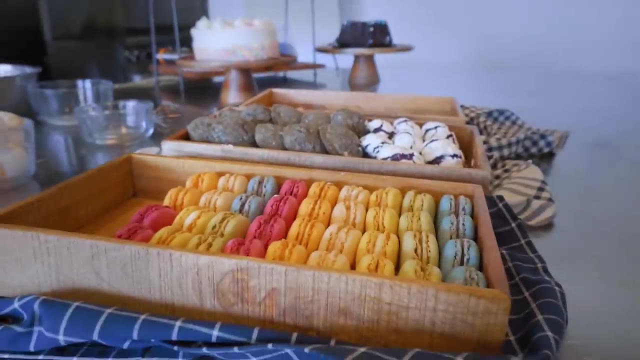 Blippi, Yeah, And a triple chocolate cake. Yeah, That looks so yummy. Well, hey, maybe you and I can cook and bake some of this. Yeah, how about today we make some macarons? Yeah, Whoa, check it out. 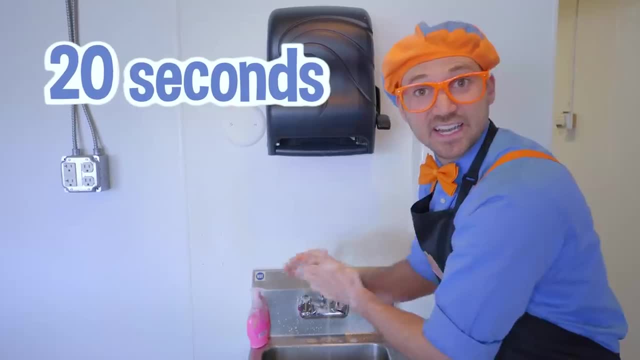 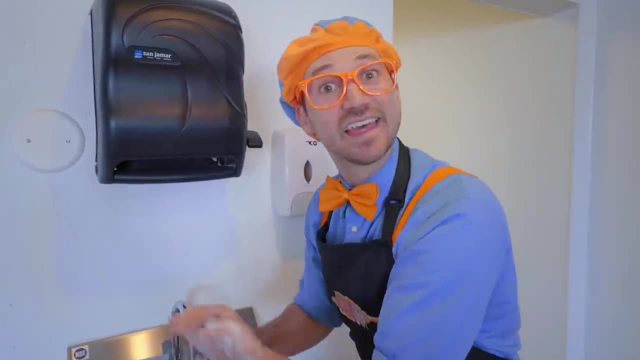 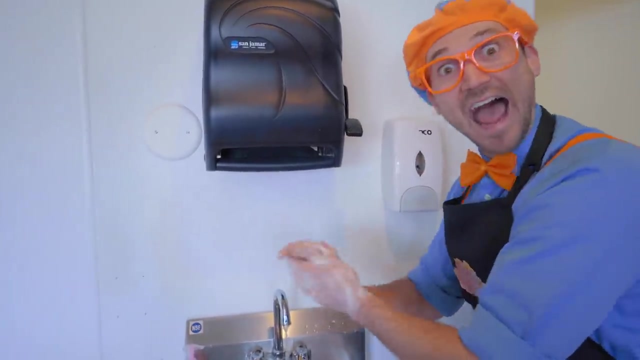 I'm washing my hands and I'm scrubbing them for 20 seconds. Yeah, do you know how long 20 seconds is? Yeah, it's about the same length as when you sing the ABCs. Will you sing with me A, B, C, D, E, F, G. 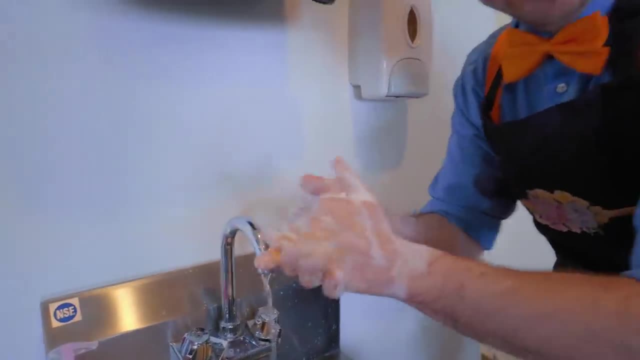 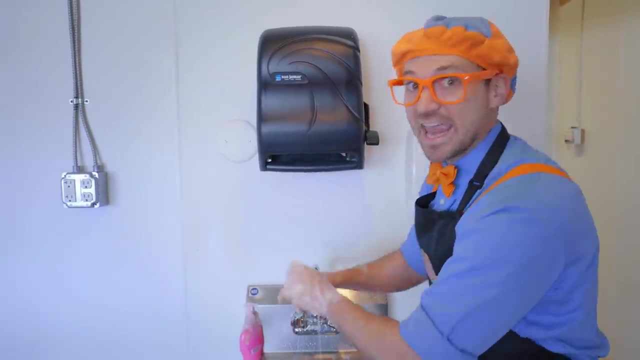 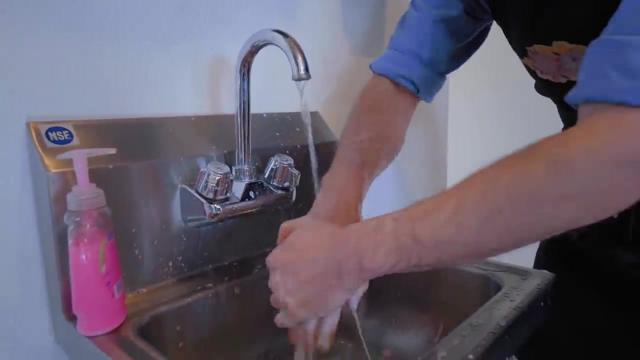 H, I, J, K, L, M, N, O, P, Q, R, S, T, U, V, W, X, Y and Z. Hey, there we go. Okay, rinse them all off. 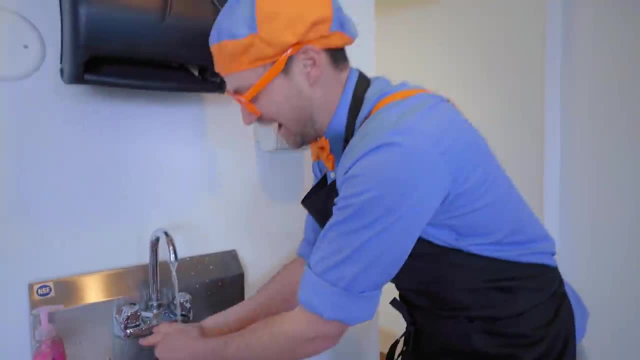 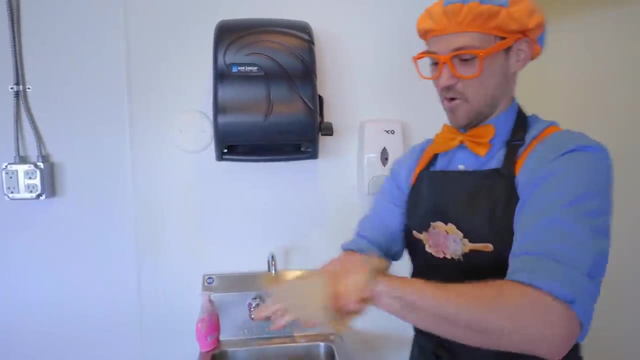 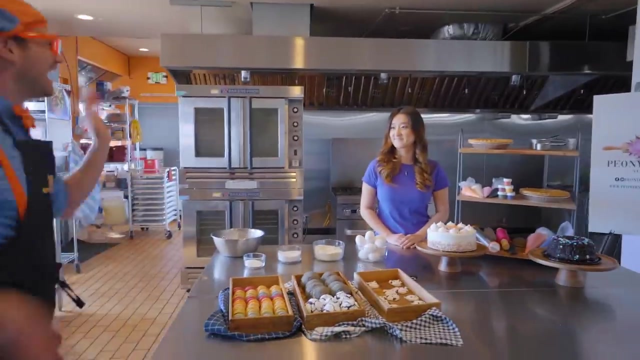 Whoa, Nice and clean now, Okay, perfect, Shut off the water. Wow, And now I'm ready to make some delicious treats. Oh hey, who are you? Hi, I'm Jennifer. I'm the baker for Candy Bakery. 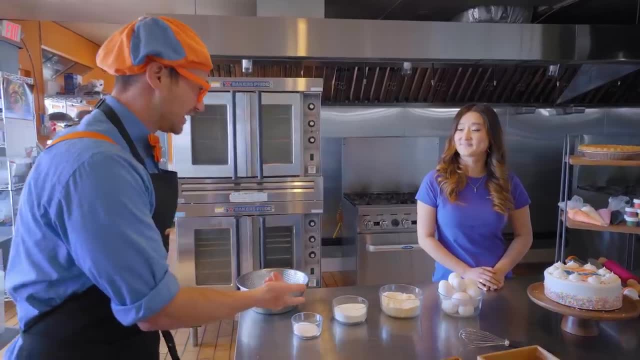 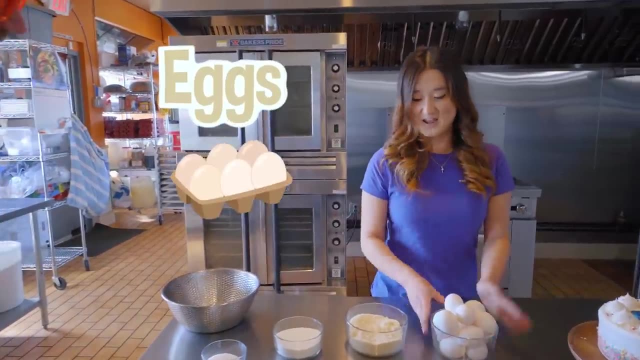 Whoa nice to meet you. I'm Blippi. Are these the ingredients? Yeah, these are some ingredients for some macarons. Ooh well, what do we have here? Well, first, we have eggs And we have almond flour, we have sugar. 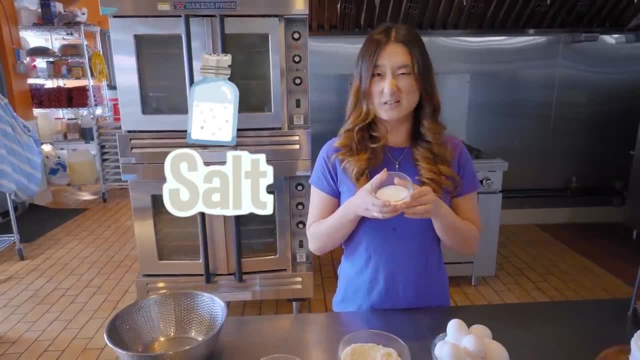 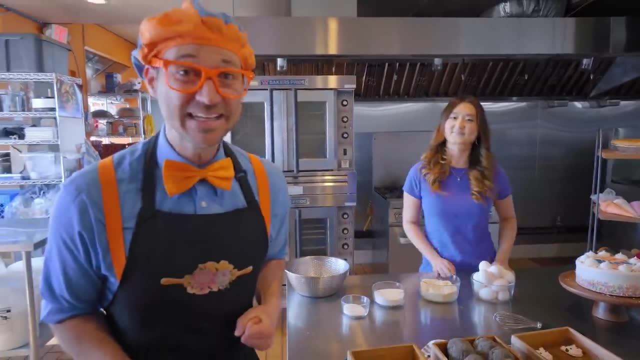 and we have an important ingredient called salt And when you eat it it's really salty, but when you put it in desserts it actually makes it sweeter and tastier. Ooh, that sounds so yummy. And you said almond flour. 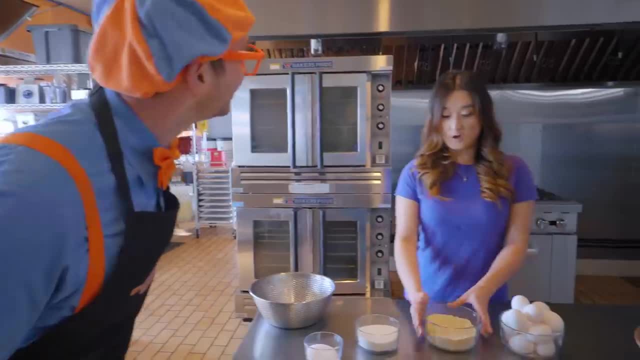 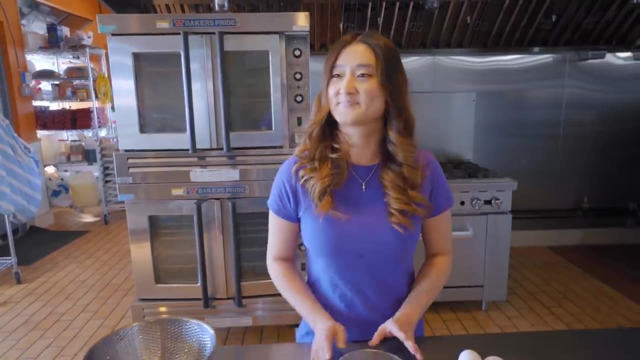 Why are we using that rather than all-purpose flour? So almond flour is special because when you put it in macarons it makes it less sticky than flour and makes it really light. Wow, that is so cool. Well, hey, do you mind? 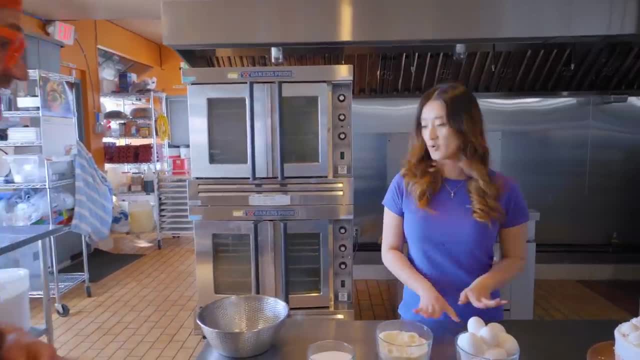 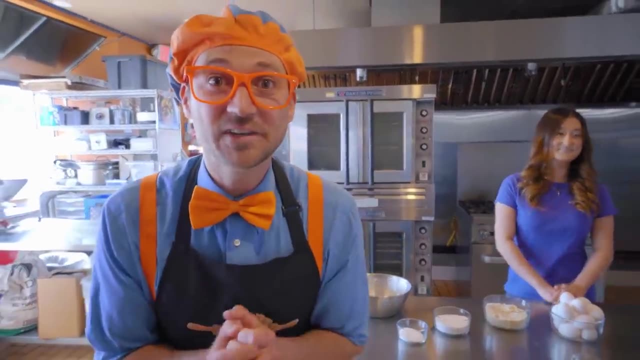 if I mix all these ingredients? Yeah, how about you throw all the ingredients into a bowl and throw it into the mixer and I'll go get the oven ready? Okay, woo-hoo-hoo, All right, let's mix all the ingredients together. 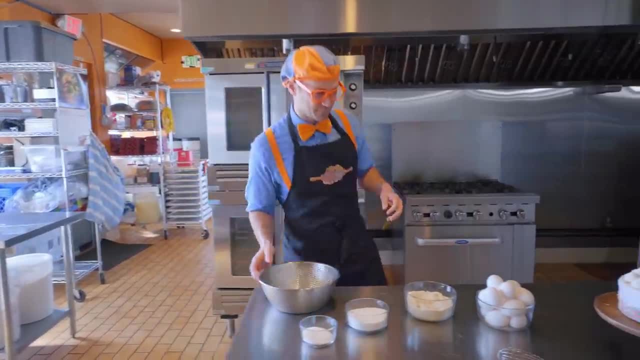 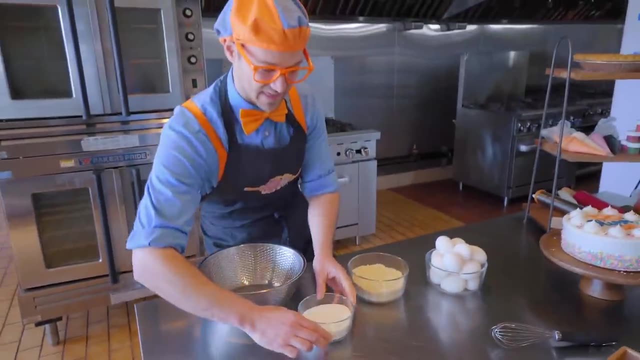 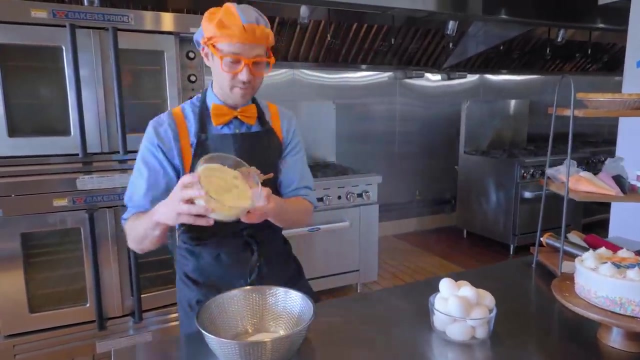 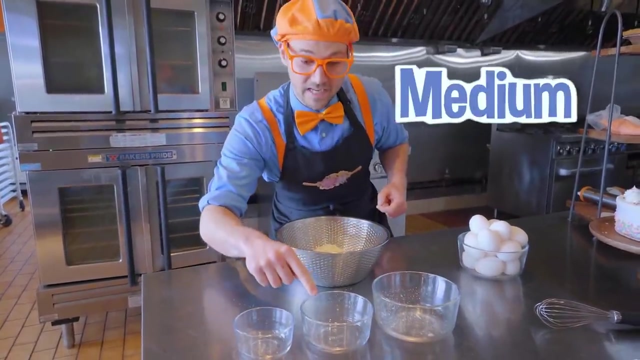 and then we'll put it in the mixer. All right, first let's add the salt, Perfect. Then we'll add the sugar, Then the almond flour, Whoa-ho-ho-ho. Hey, check it out. A small bowl, medium and large. 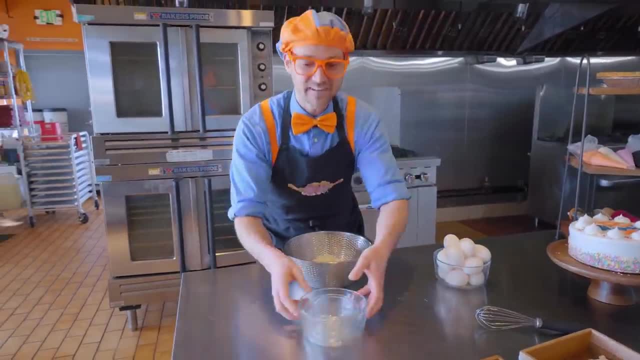 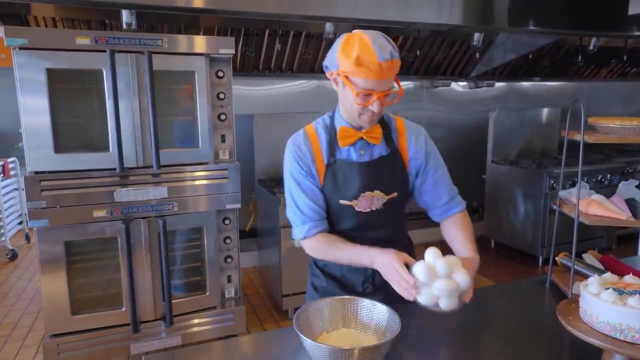 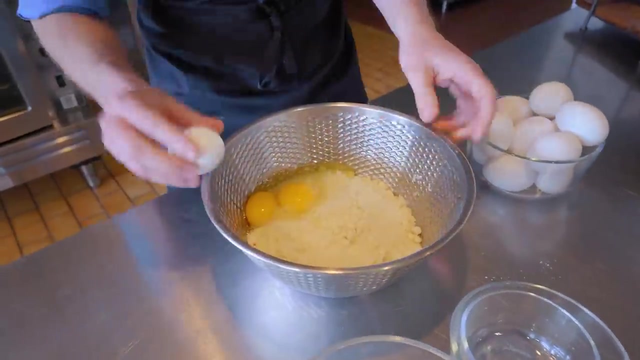 Ha-ha, there we go. Perfect. And for the eggs? Oh wait a second, I probably have to break them open. All right, here we go. Ha-ha, Now I'm gonna go put it in the mixer. 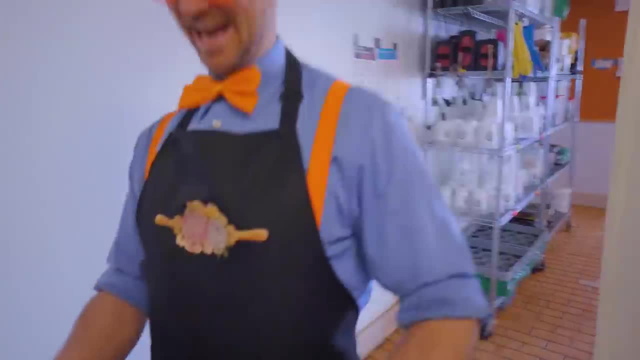 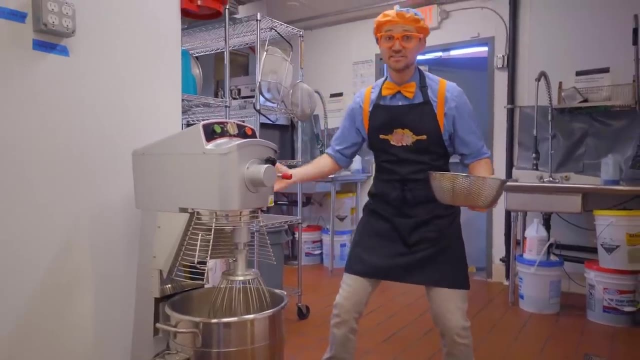 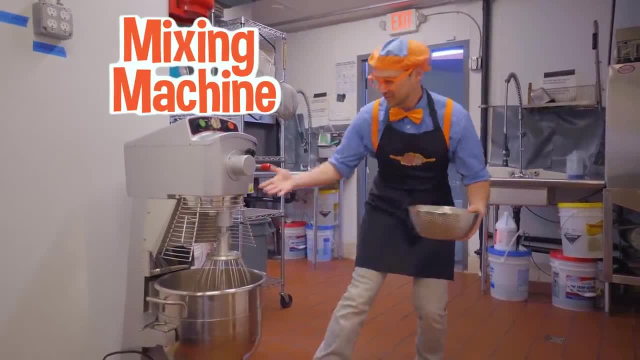 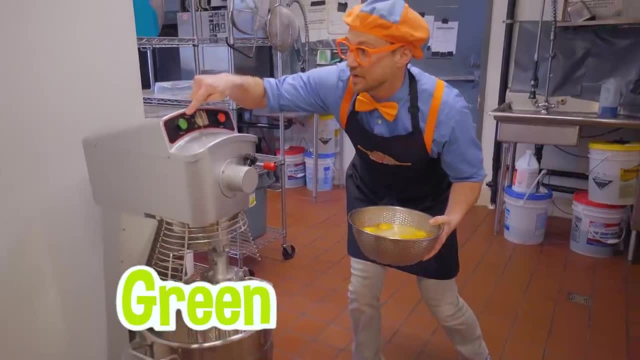 Whoa-ho-ho-ho, Look how big it is. There's a giant whisk right here. Wow, Looks like there's a green on button, a red stop button and a big bowl for me to add all the ingredients. 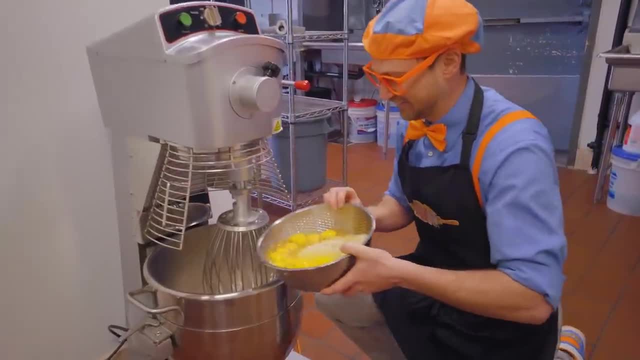 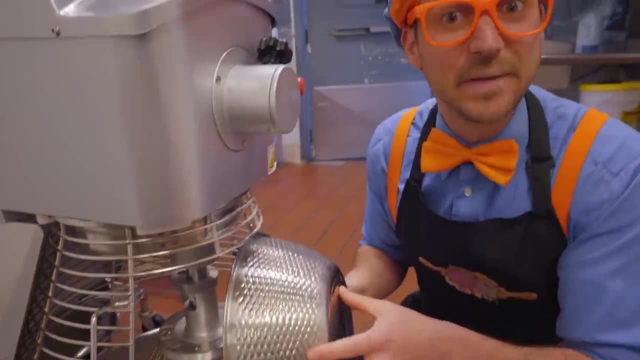 All right, let's go. All right, here we go. All right, Here we go, Pour it in. Looks like we already made some earlier. Yeah, this is gonna be a big batch Whoa-ho-ho-ho. 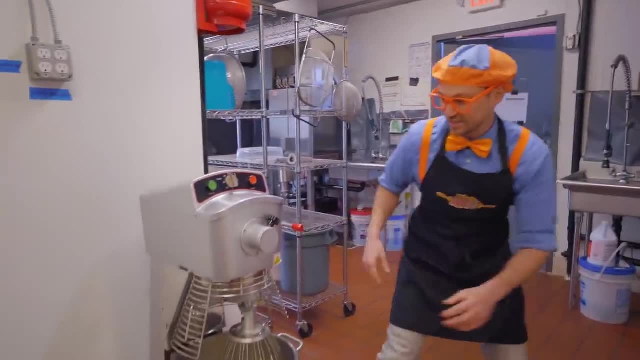 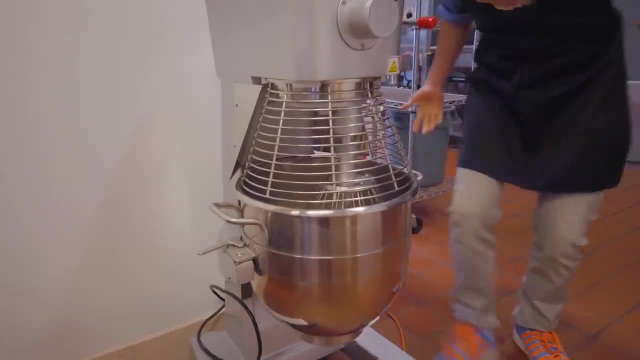 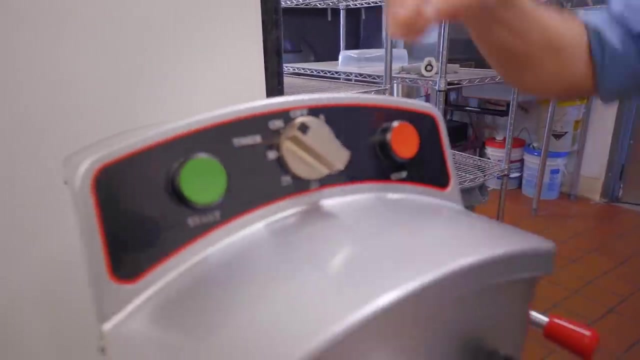 All right, now that all the ingredients are in there, we need to make sure that the cover is closed. We need to raise up the bowl. There we go. And now we need to turn this to the on position. There we go. 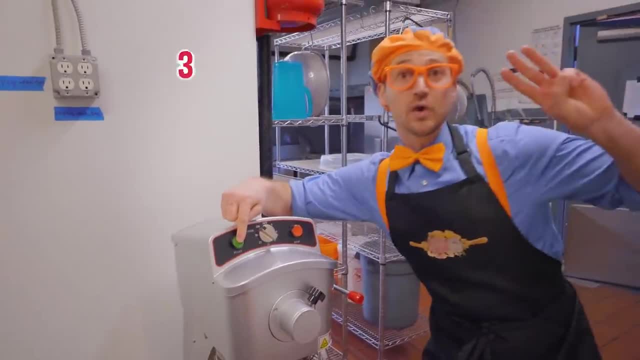 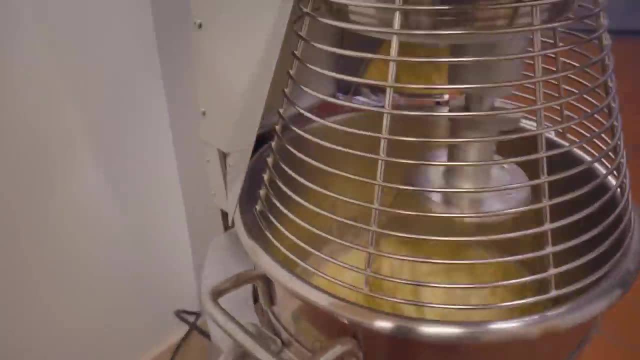 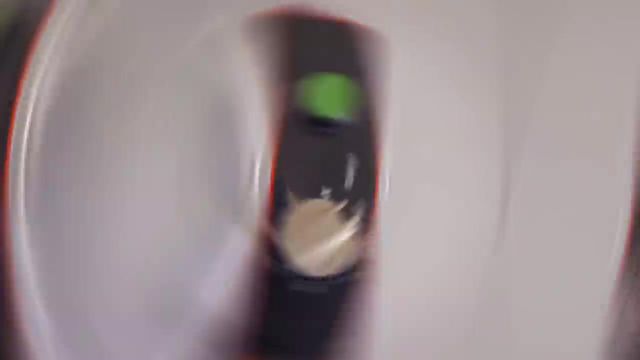 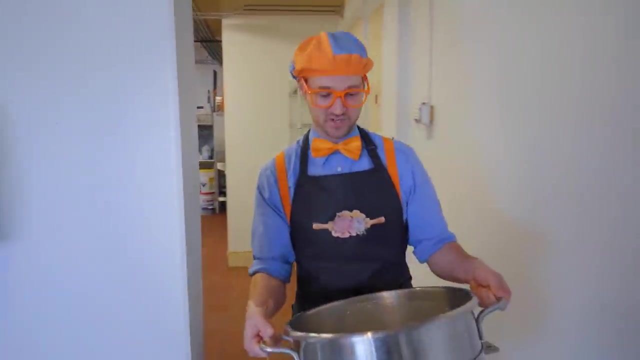 And we'll push the green start button in three, two, one. Yeah, Look at it. mix, Whoa. Yeah, The batter is finished. Whoa-ho-ho-ho, This is a big bowl, Pfft. 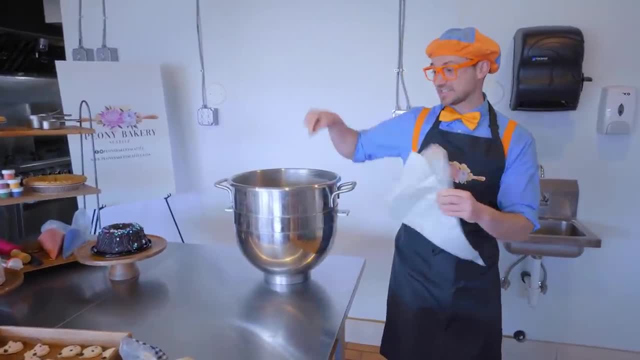 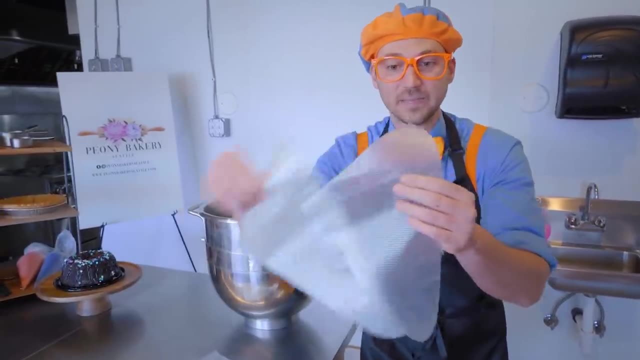 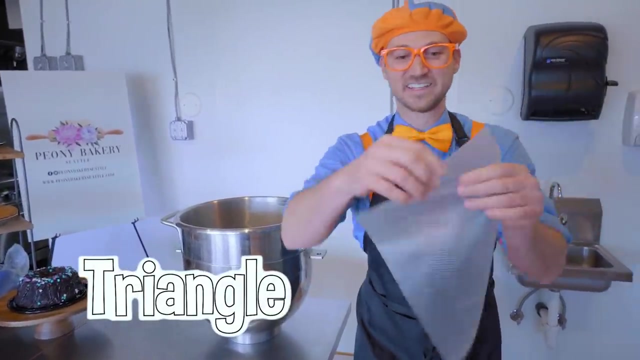 Okay, Okay, Okay, Here's what we need to do. Yeah, let's take some of this batter and put it inside these piping bags. Yeah, What shape is this piping bag? Oh Yeah, Looks like a triangle, Perfect. 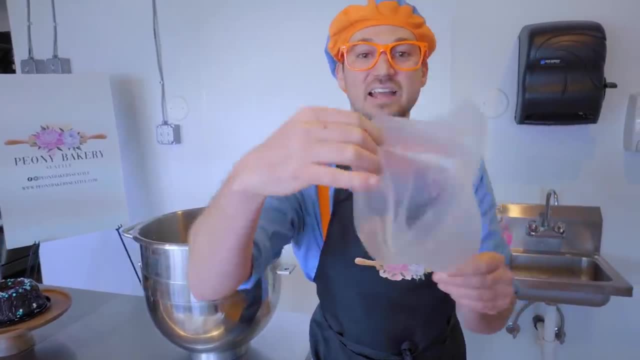 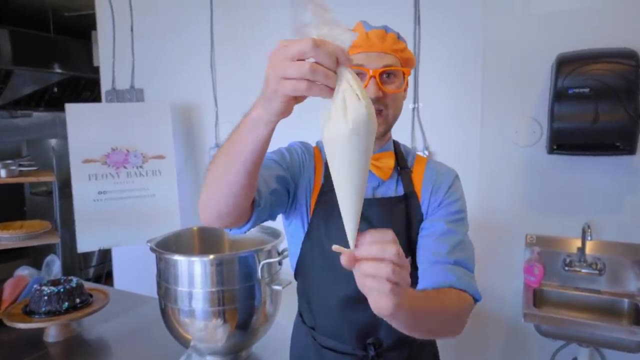 And do you see how you open it up? Yeah, And that's where you put all the batter. But hey, check it out. Yeah, we have some batter already in a piping bag. Whoo-hoo-hoo, Ha-ha-ha. 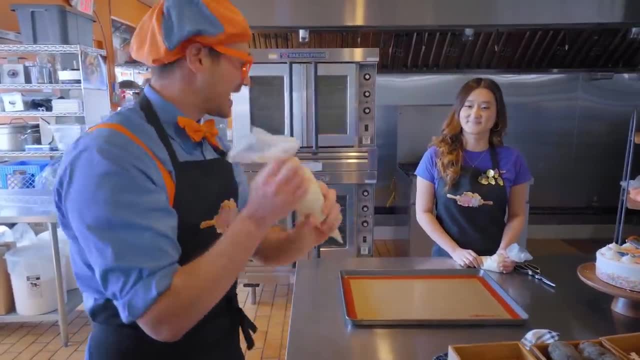 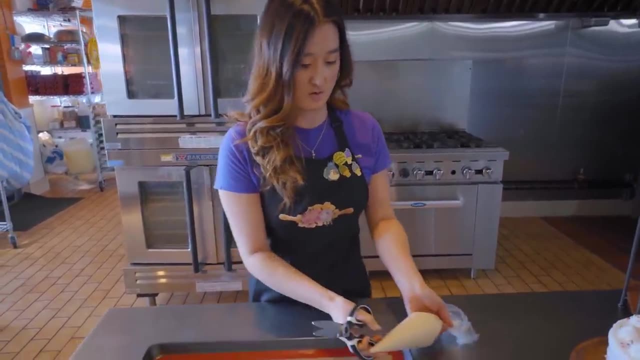 Okay, Jennifer, Now that we have the batter in the piping bags, what do we do now? Well, first we need to cut the bag. Okay, Cut mine, Okay, Okay, And we're gonna make some cow macarons. 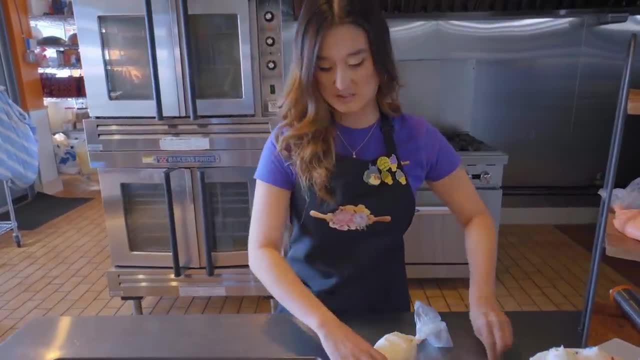 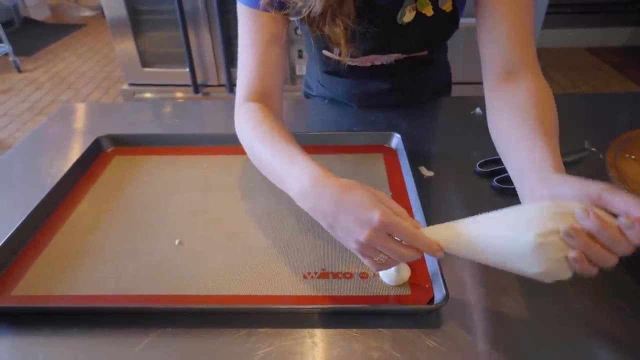 Ooh, To do that first, you're going to need one big circle. Okay, I'm gonna make cow macarons And we need a big circle, For is that the head? That's gonna be the head, yeah. 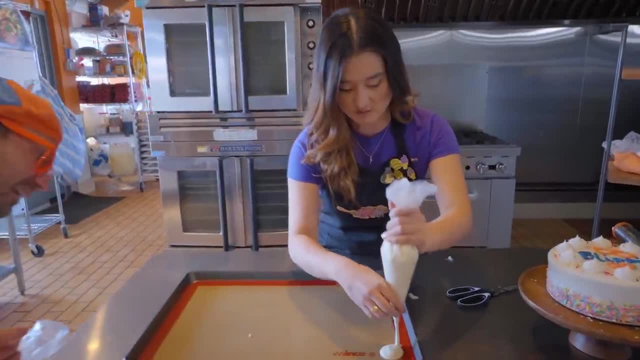 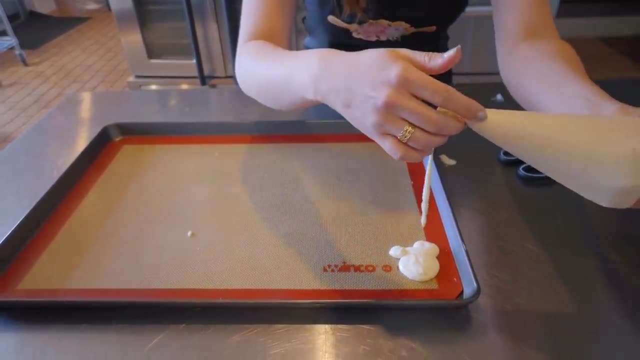 Okay, Then we need two small circles on the top for its ears. Okay, That is not how I want it. That's funny. That's okay. Okay, I see it. Yeah, the head and then two ears Here, let me try. 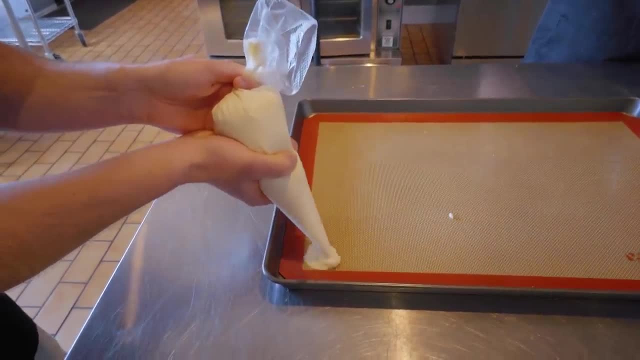 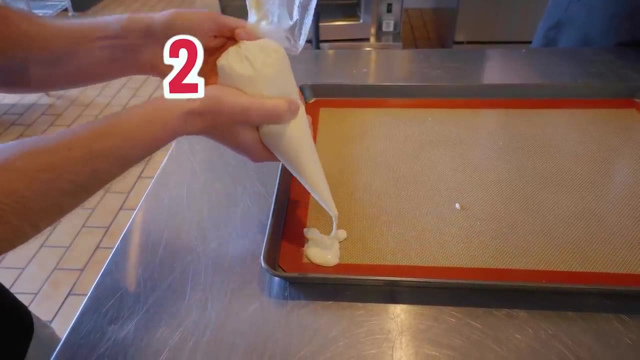 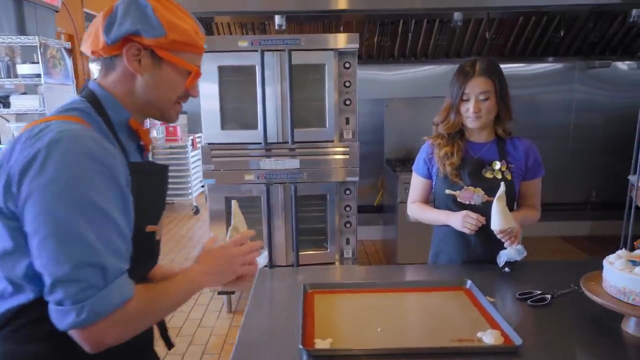 All right, There we go. Yeah, looks just like that. And then one ear, two ears, Perfect, That's gonna be one great cow. Okay, do we fill it up now? Yeah, let's fill up the whole pan. 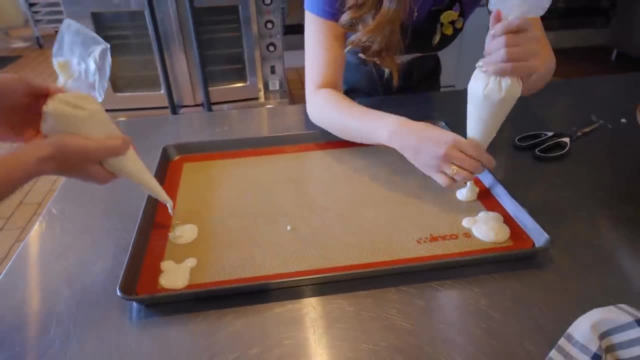 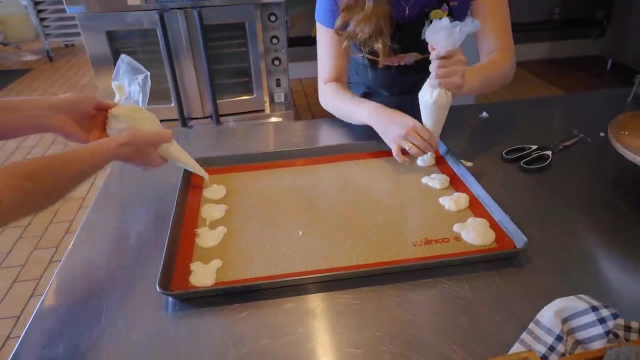 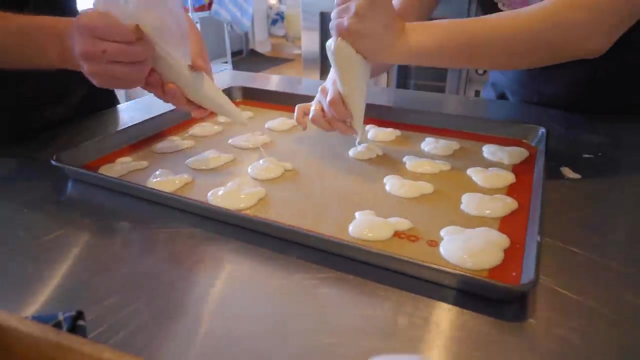 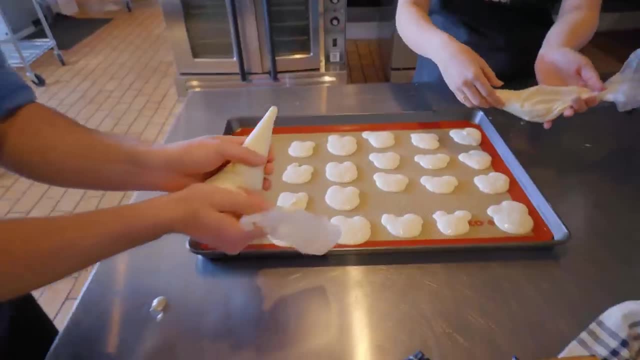 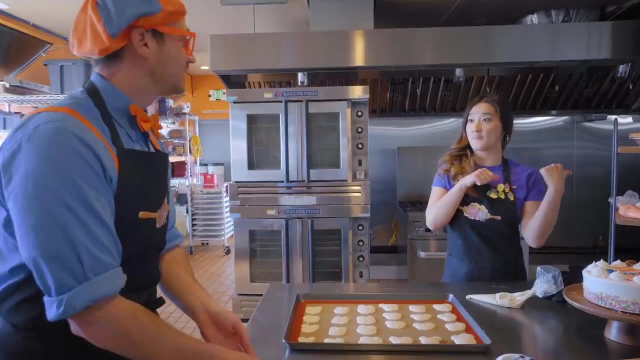 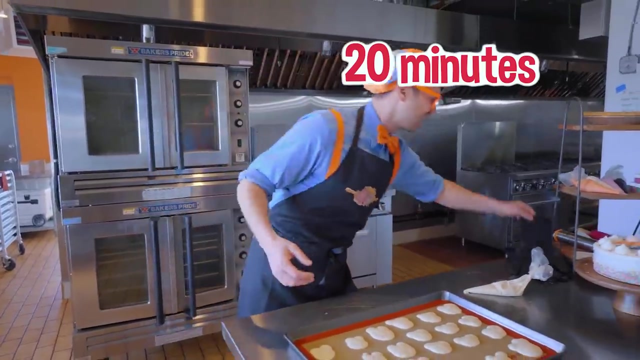 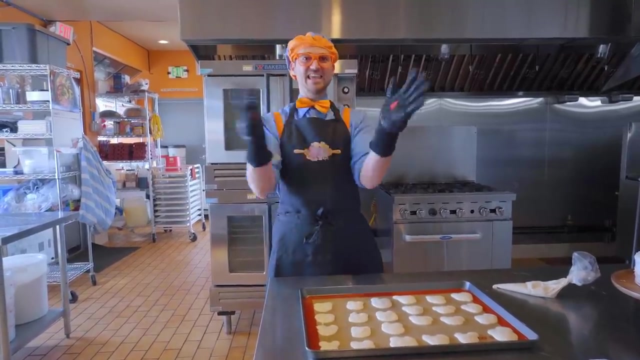 Yeah, Yeah, Yeah, Yeah, Yeah. Whoa, That was so much fun. Yeah, now that we're done, why don't you throw them into the oven for 20 minutes and I'll get the butter cream ready, Okay. 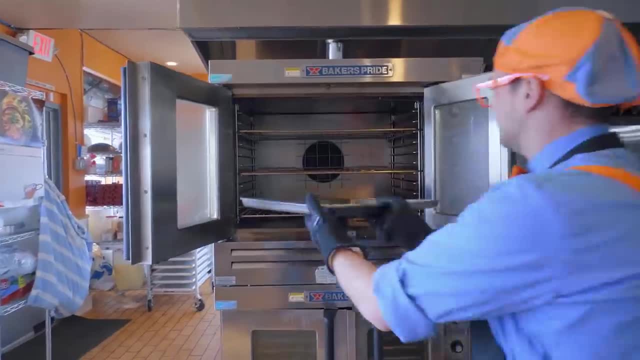 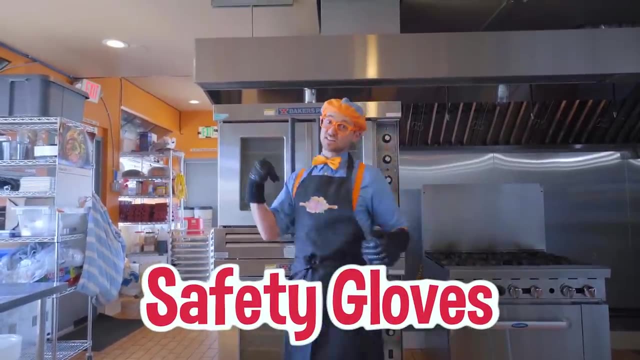 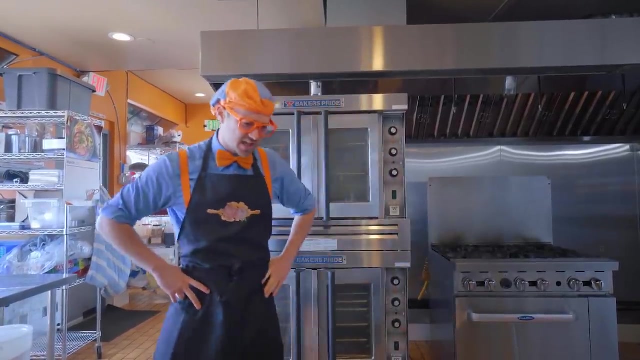 All right, so I need to throw these in the oven for 20 minutes. Whoa, Wow, I used my safety gloves, because ovens are not a toy. You need to be very careful. Okay, what did Jennifer say? She said 20 minutes. 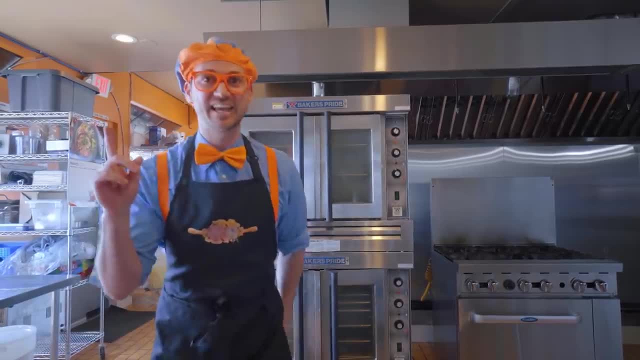 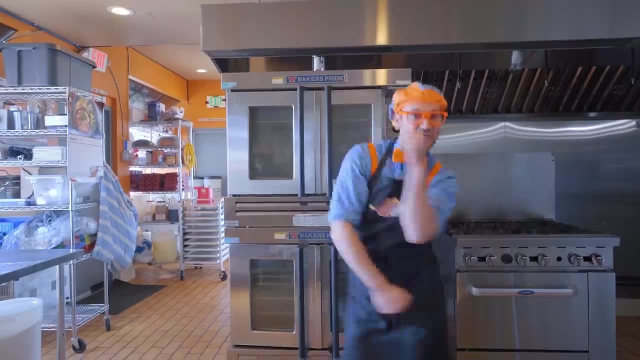 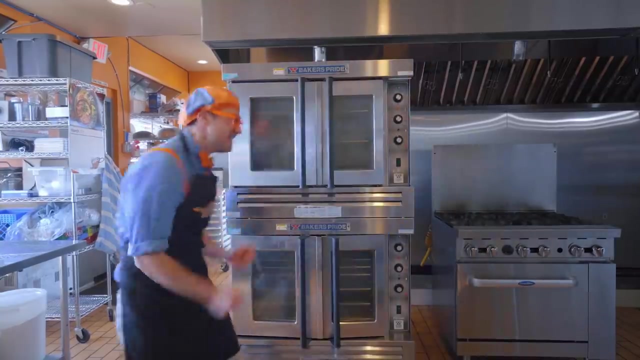 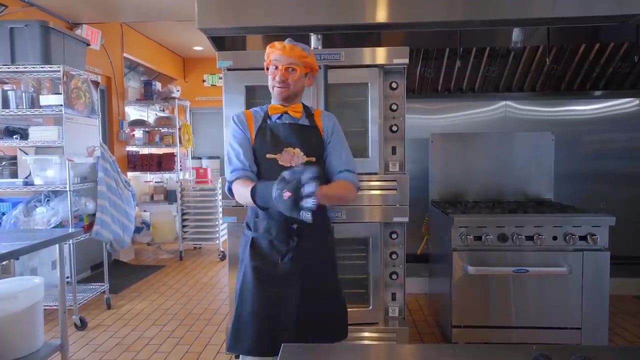 Oh, that's a long time to wait, But wait a second. You know what I like to do when I wait? Yeah, I like to dance. Woohoo, Did you hear that? Yeah, That buzzer means that they're probably done. 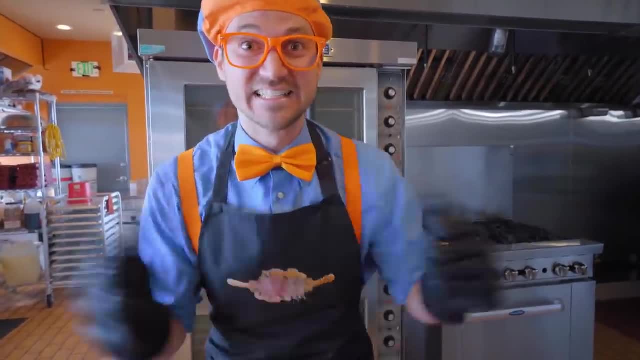 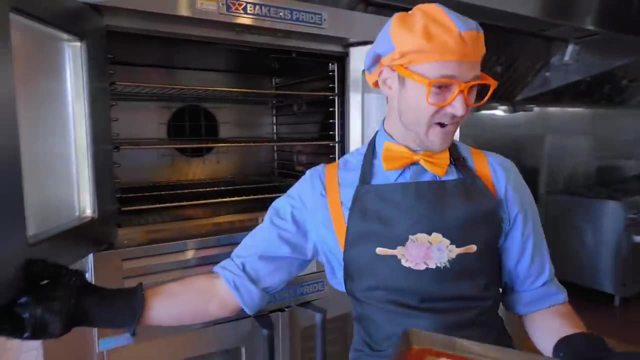 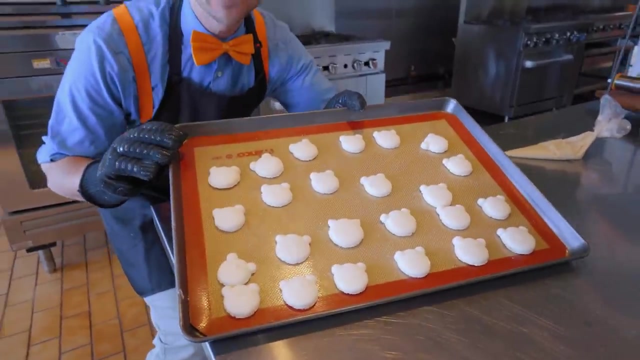 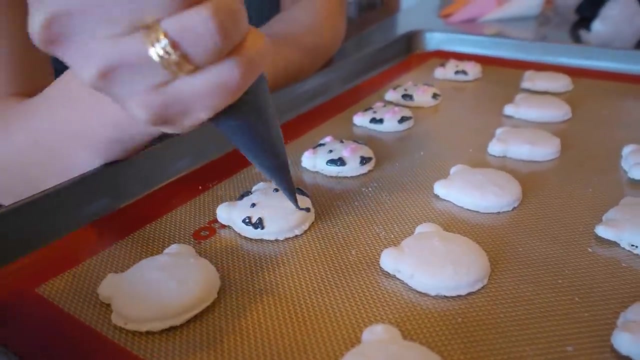 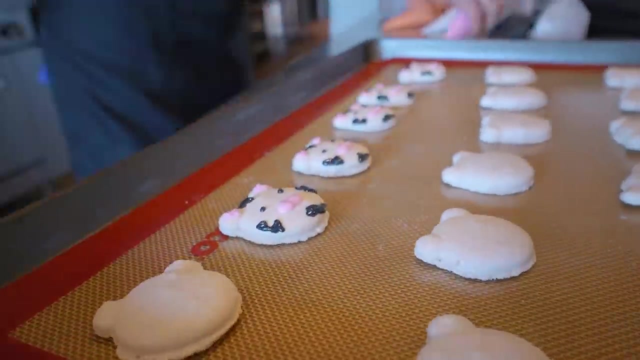 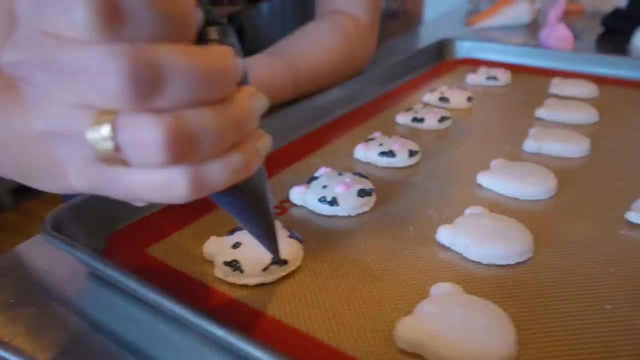 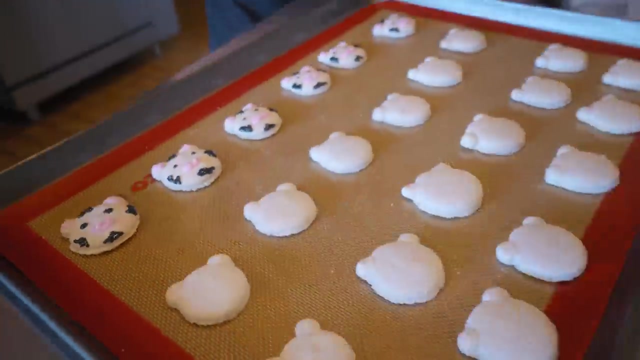 Yeah, Let's open it up and then see the macarons. Whoa, Woohoo, That is hot And they look so yummy. Wow, Check it out. Now it's time to decorate. Ha ha, Wow, That looks like so much fun. 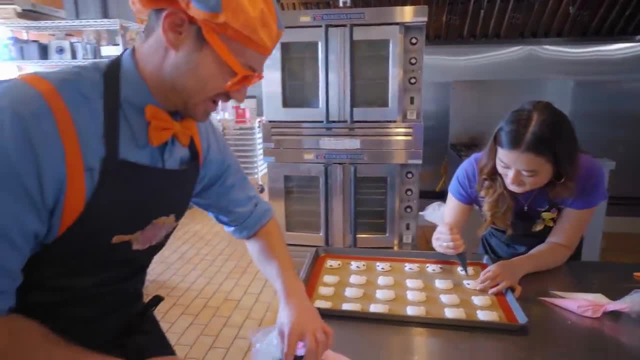 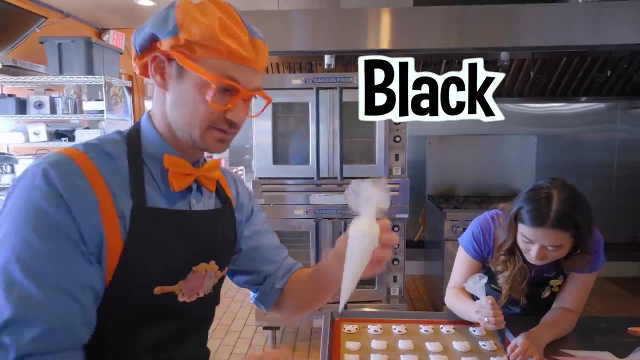 Hey, can I try? Sure Blippi. Go ahead and give it a try. Sure, Okay. Uh well, looks like we have three colors here. We have black And then, uh, looks like we have white And then looks like we have the color pink. 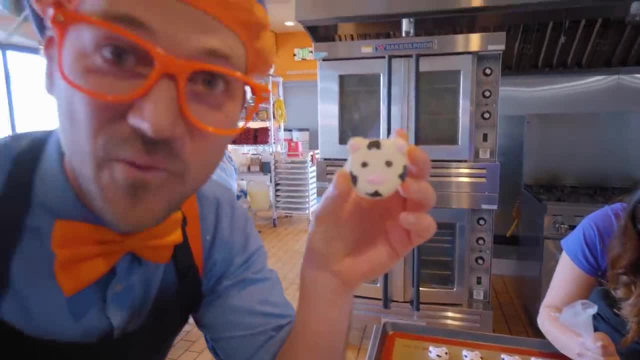 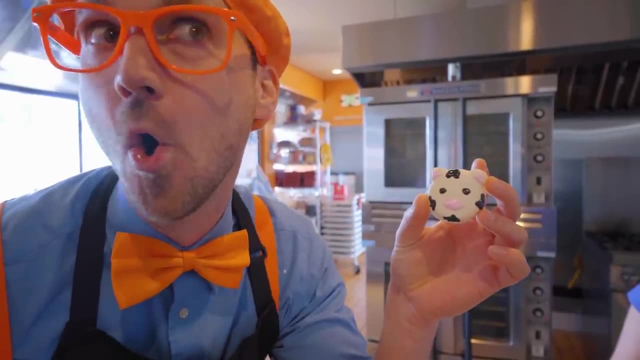 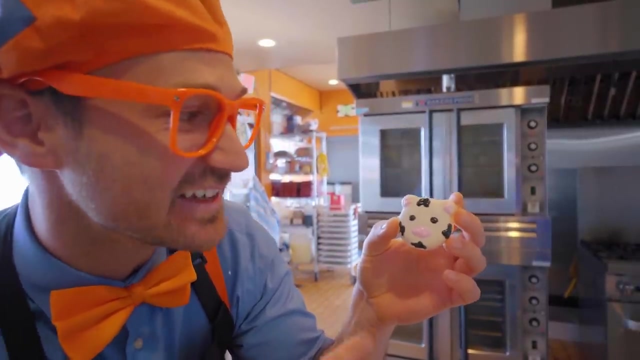 Let's see What are we making. Oh yeah, Remember these from earlier. Yeah, a cow, A cute cow, Moo Ha ha ha. Yeah, Has two eyes, Has two ears, Has some spots And a really cute nose. 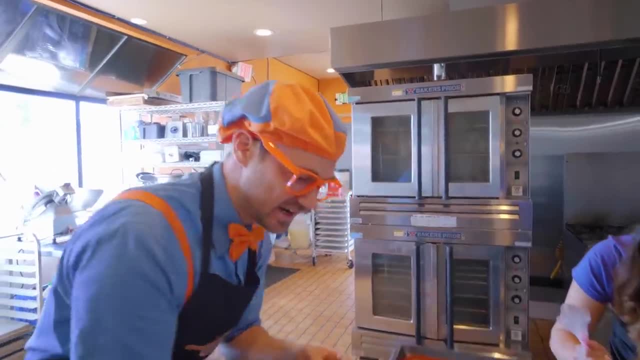 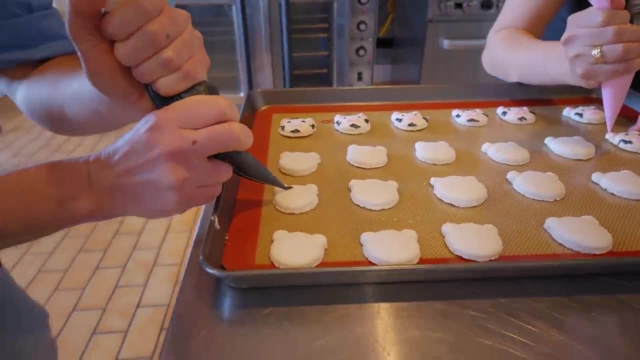 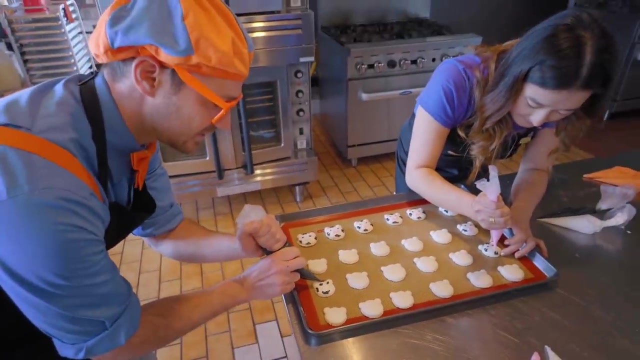 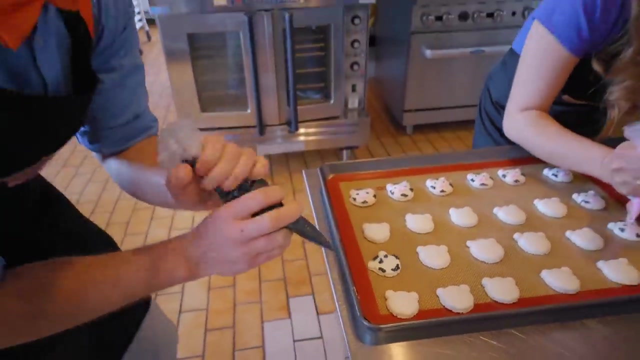 Ha ha. Okay, Let's put that down right here And I'm gonna start with the black. All right, Looks like we'll do two eyes And we need to do the spots. Cute little hair thing on top, Ha ha. 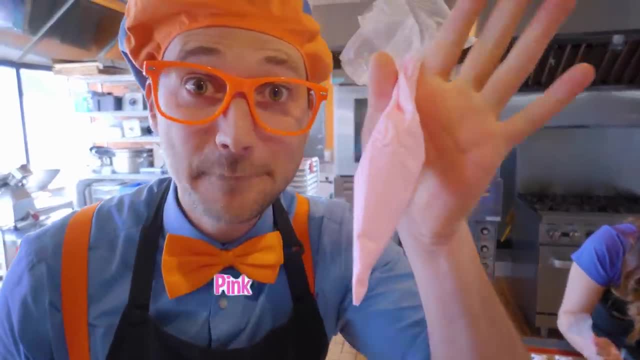 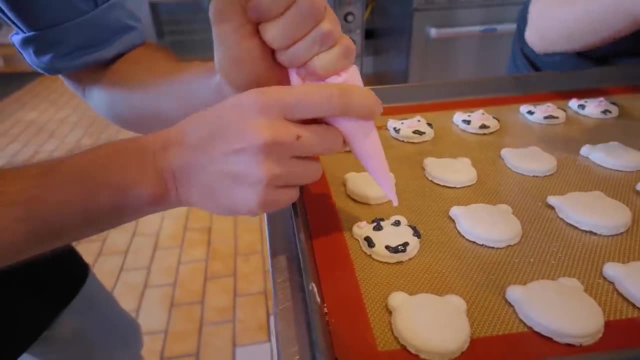 Okay, So now let me move to the color pink. Ha ha, All right, Looks like pink And put it on the ears And it's the base for the nose. Last but not least, the color white. Ha ha. 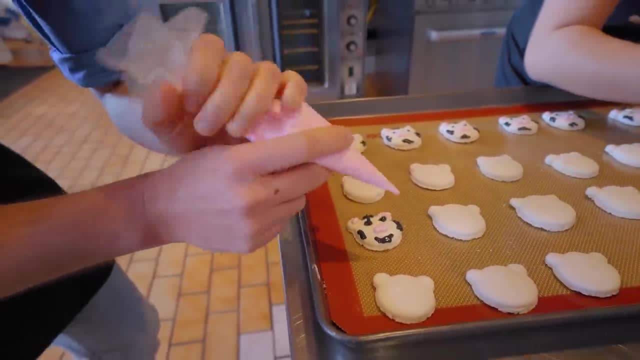 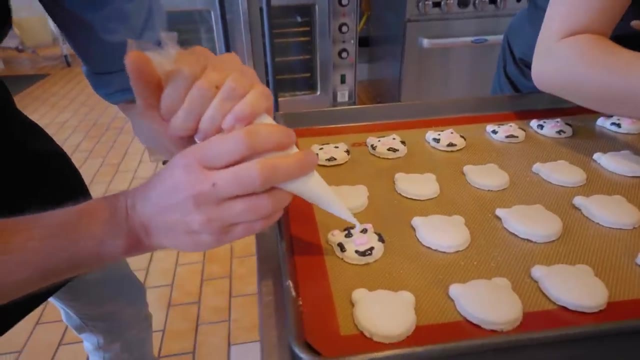 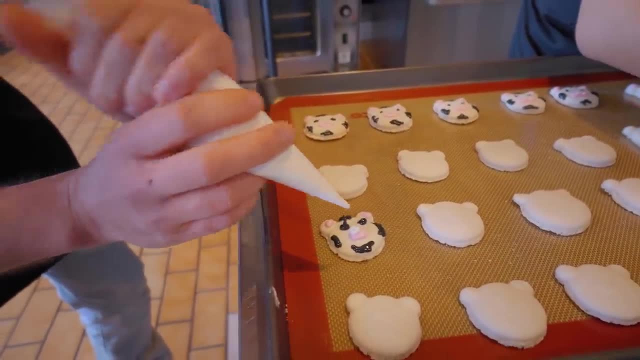 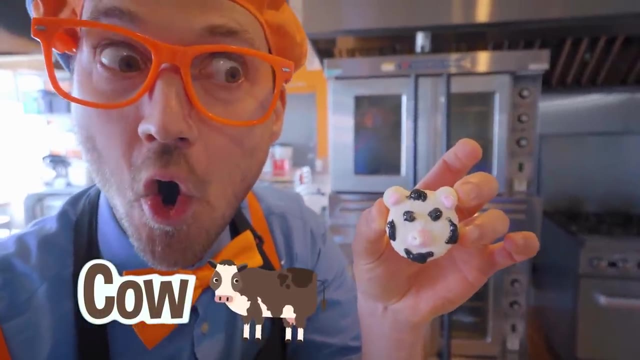 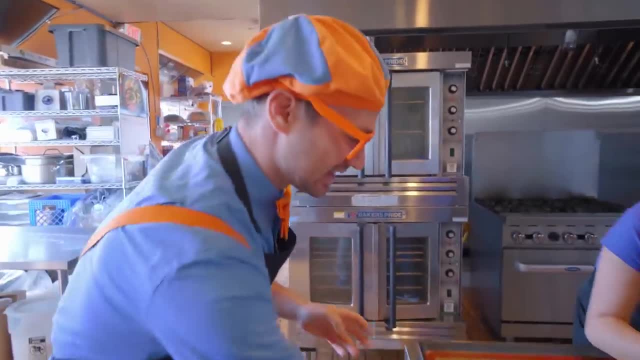 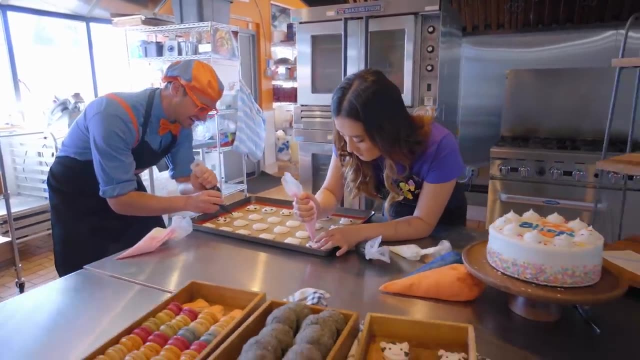 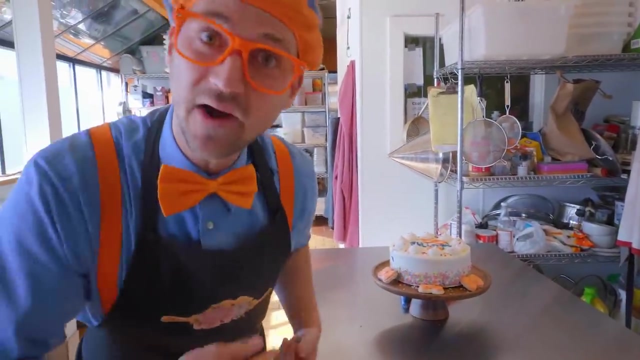 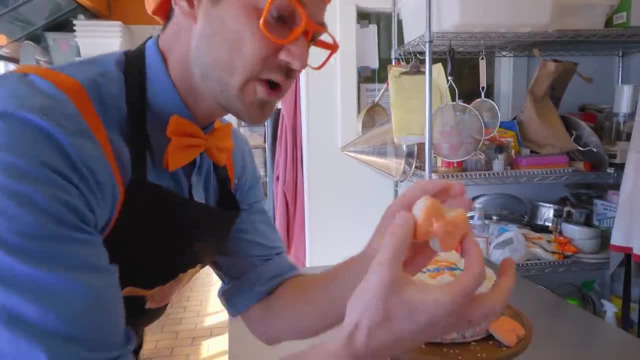 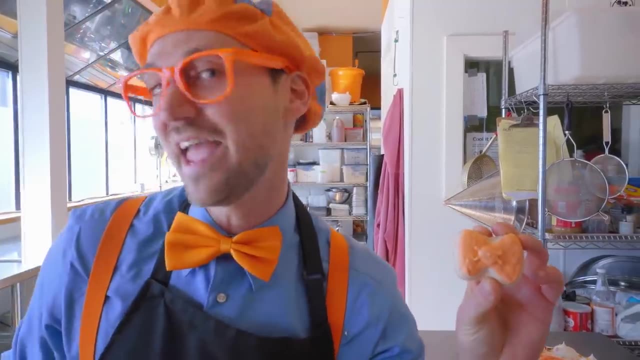 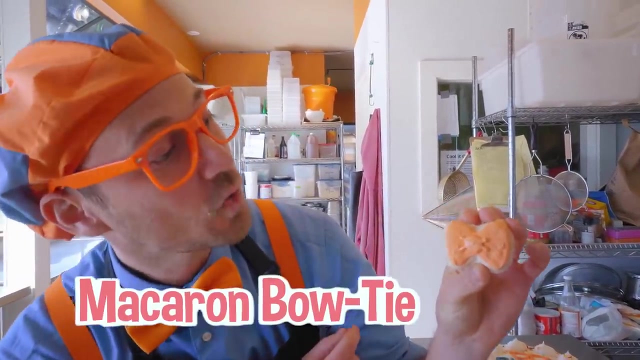 Oh, Oh, Oh, Oh, Wow. What are these? Yeah, Macarons, Yum, They're so tasty. What is this, though? Yeah, Does it look like my bowtie? Yeah, It's an orange Blippi Macaron Bow Tie. 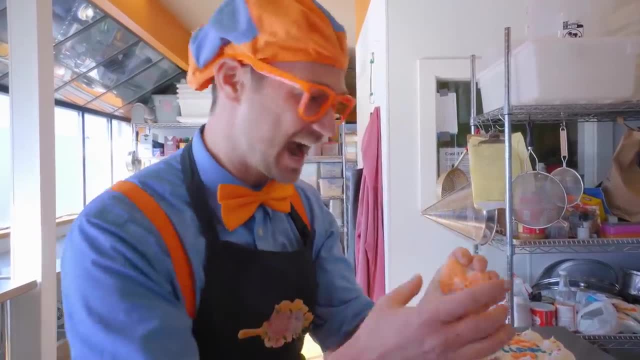 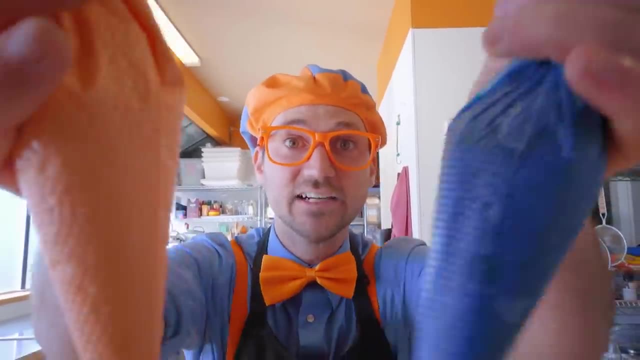 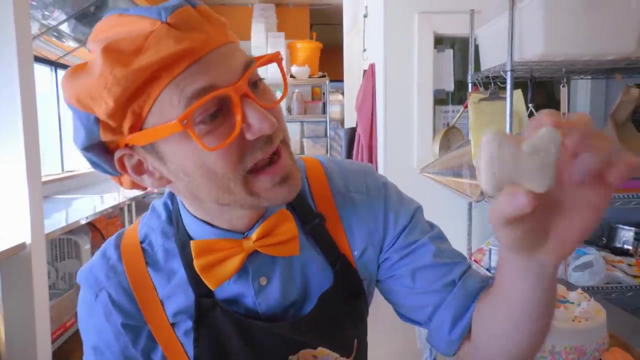 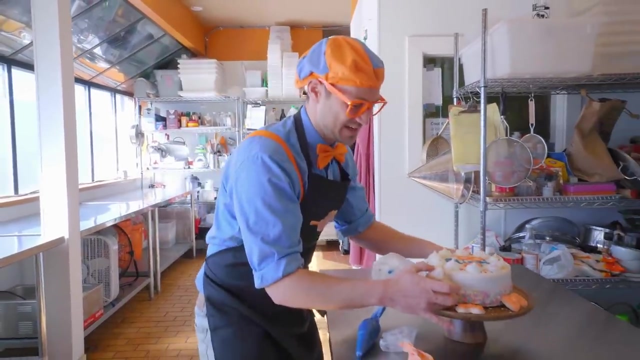 It looks so tasty, doesn't it? Yeah, Hey, Check this out. I have two things of Icee- My two favorite colors, Blue and orange- and check it out. I have a flippy macaroon that's empty- no colors at all. so maybe, just maybe, we can. 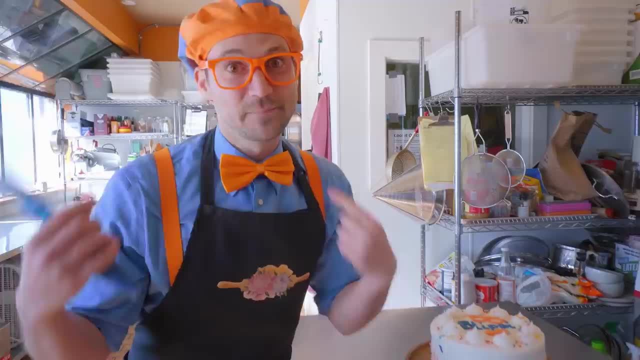 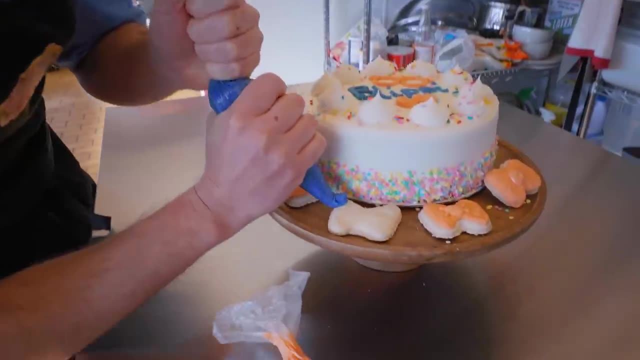 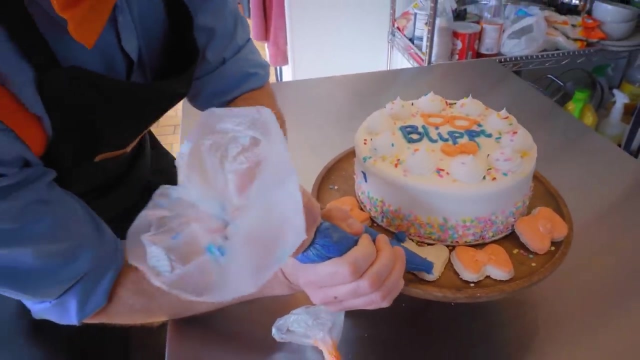 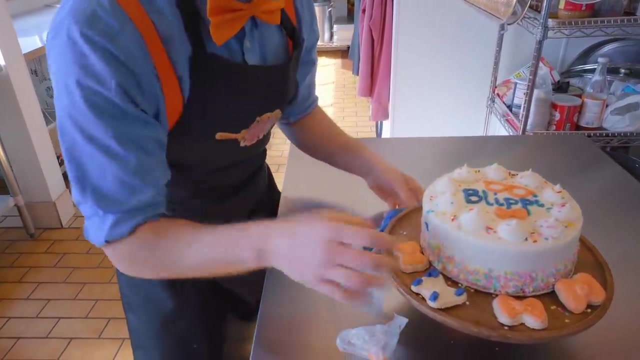 use some of this icing to decorate it. so my normal bow tie is orange, but I'm actually gonna use some blue too, so let's just squirt some out. oh, that looks cool. do a big dot there. do a big dot there, about one right there. oh, and one way over there. oh, that doesn't look like my bow tie, does it no? 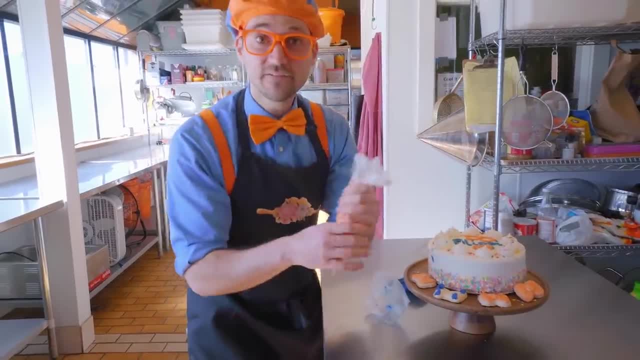 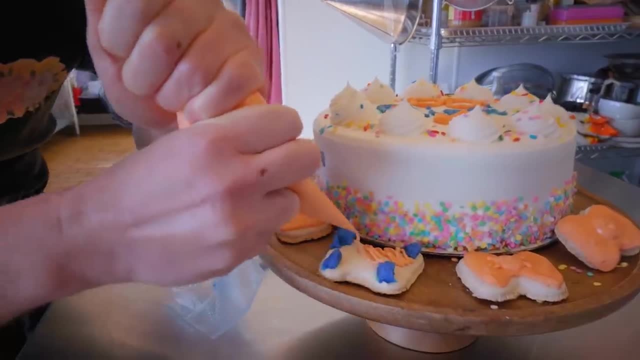 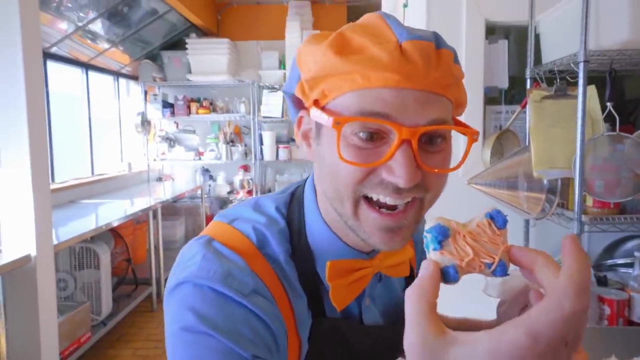 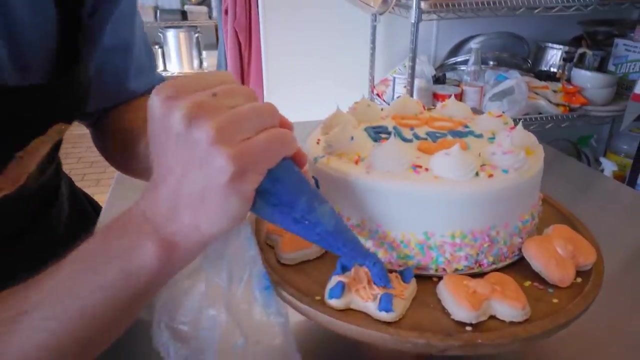 that's okay, though sometimes, when you're being creative- yeah, actually all the times when you're being creative- you could do whatever you want. yeah, like this: whoa, check it out. whoa, yum, doesn't that look tasty? and hey, watch this, I'm gonna do another big blob. yeah, a blue. oh, I will just finish that all the way. 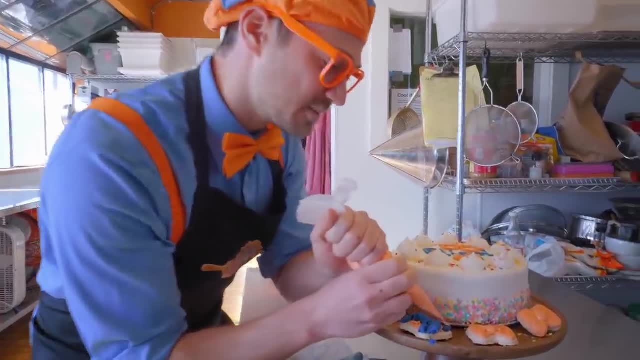 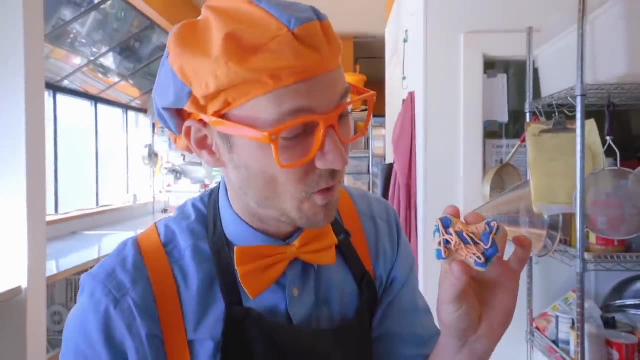 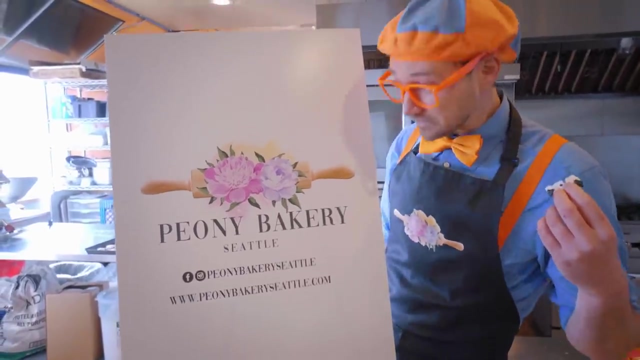 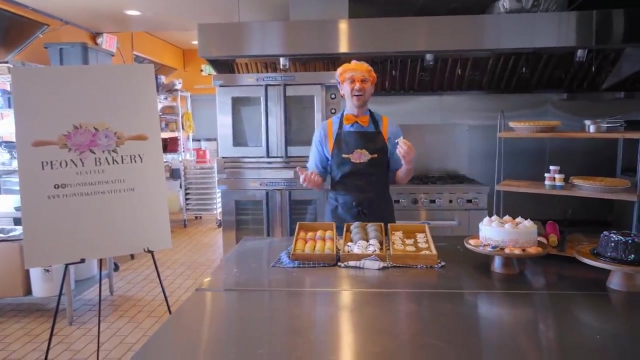 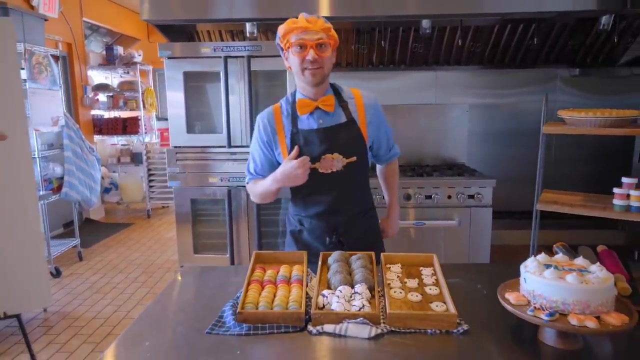 across there, and then I'll put some orange on top of that. wow, now does that look tasty, or does that look tasty? yum, these are so tasty. that has been so much fun making all these sweet treats with you, hasn't it? yeah, I want to give a special thanks to Jennifer atpenny. 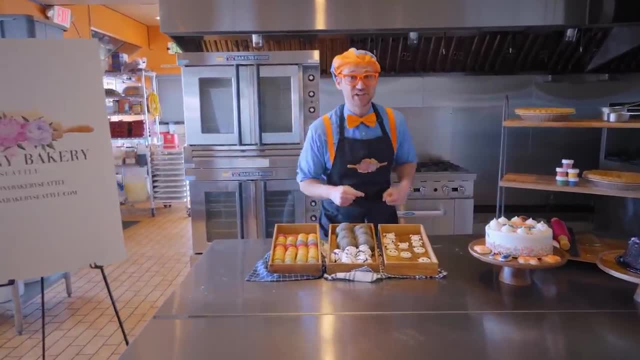 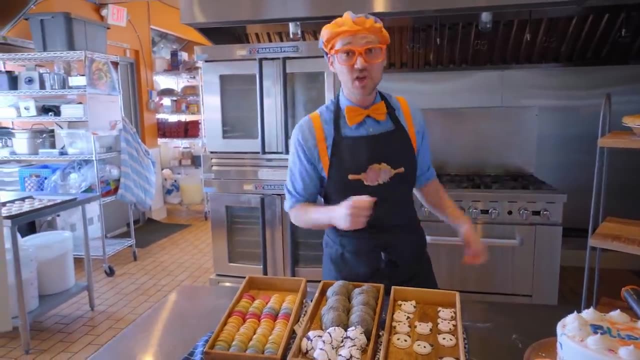 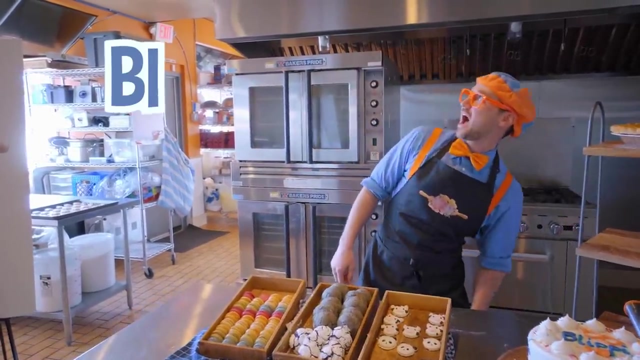 Bakery in Seattle Washington. wow, she did such a good job and they are so yummy. well, this is the end of this video, but if you want to watch more of my videos, all you have to do is search for fragment name. Will you spell my name with me? Ready B-L-I-P-P-I, Blippi, Good job, Alright, see. 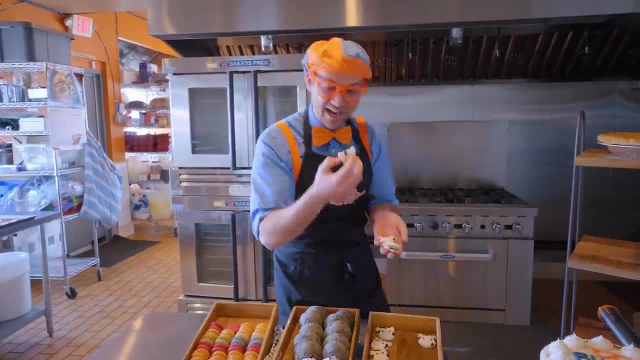 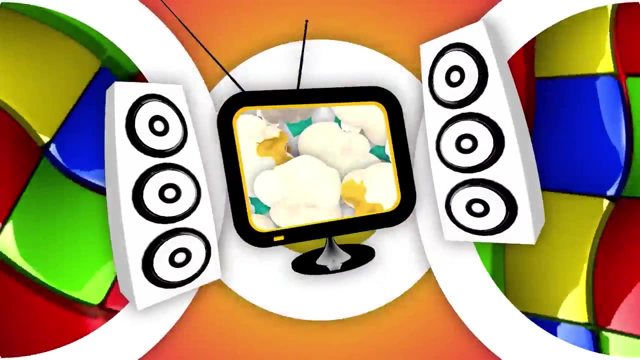 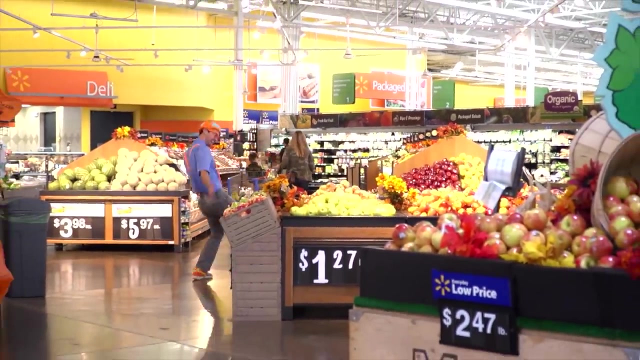 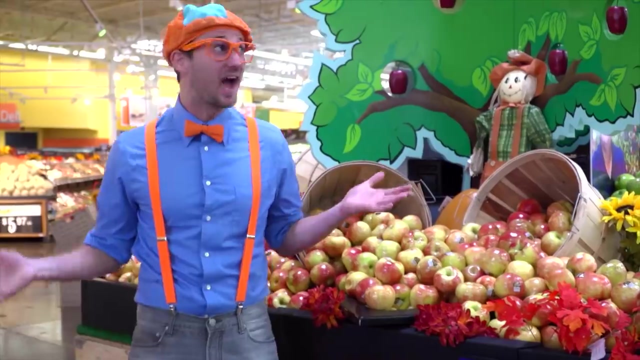 you again, Bye, bye. So much to learn about. It'll make you want to shout: Blippi. Hey, it's me, Blippi, And look at where I'm at. I'm at a super center, But look at what. 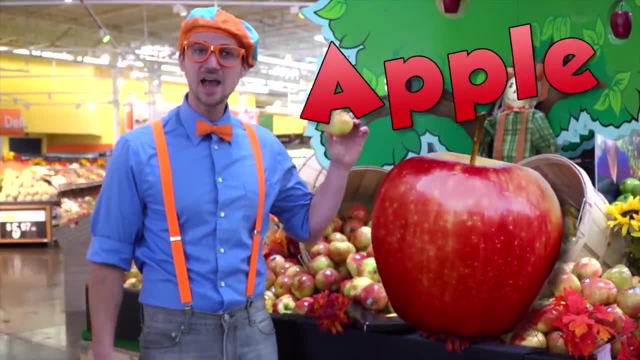 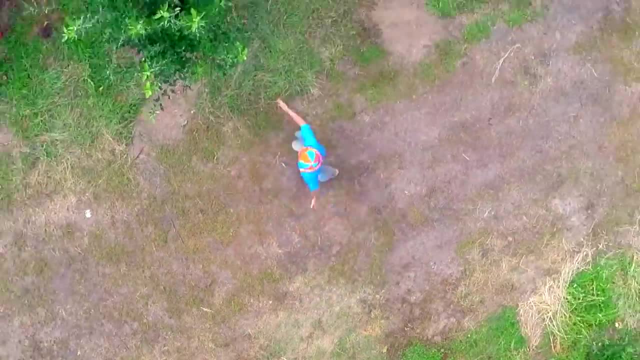 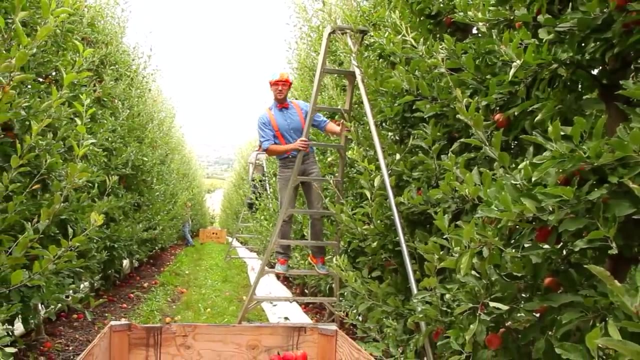 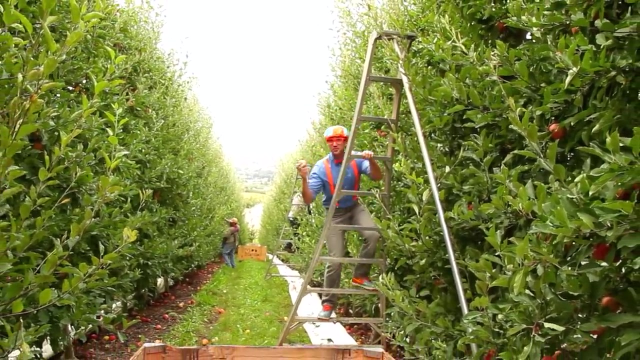 it is. It's a delicious apple. I wonder how this apple got here. Every apple at the grocery store came from an apple field. First you gotta pick the perfect fruit Like this one. This one looks really tasty, And after you pick it you put it inside the. 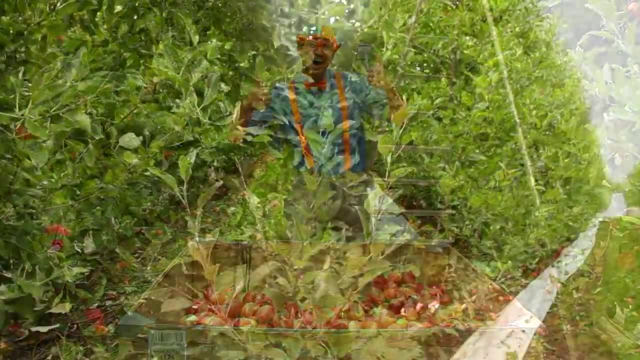 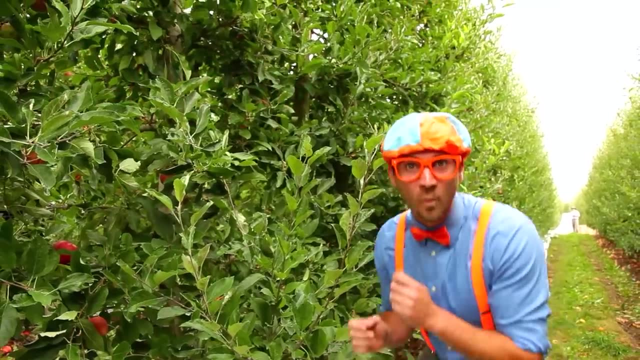 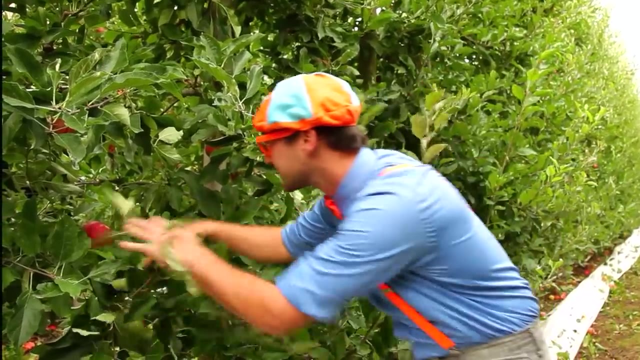 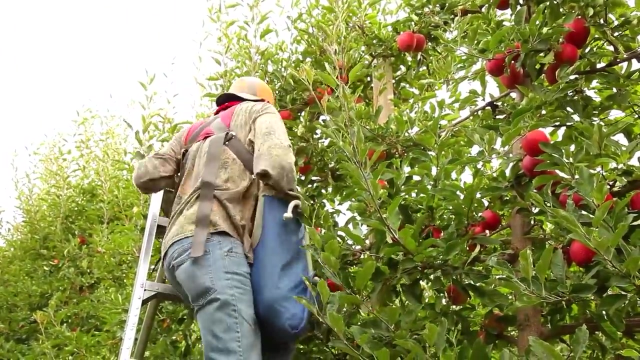 bin with all the other apples. Let's try and find an apple together. Do you see an apple? I see one. Yeah, look, Yum. It all starts by a worker handpicking every single apple, And then they dump their. 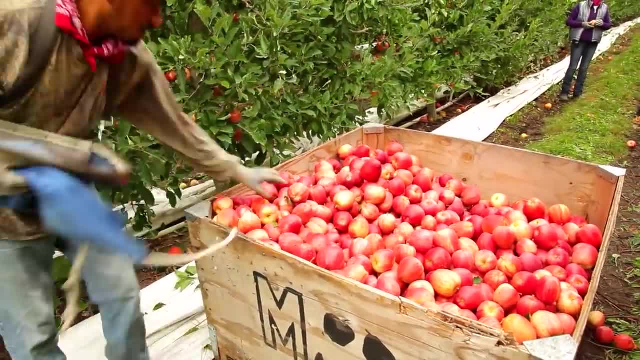 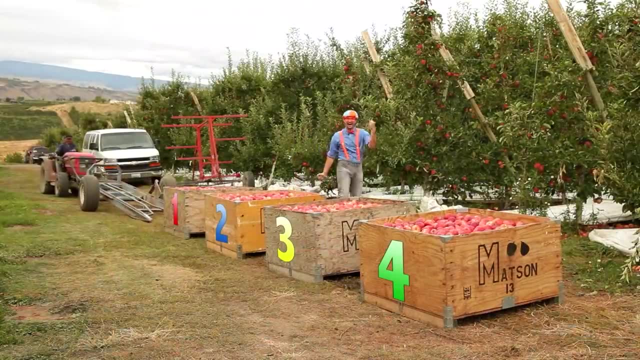 sack into the bins And when the bin gets full, a tractor picks it up and takes it away. Now that the apples are all out of the fields and into the bins, and the bins are full, now we need to transport them to the bin. 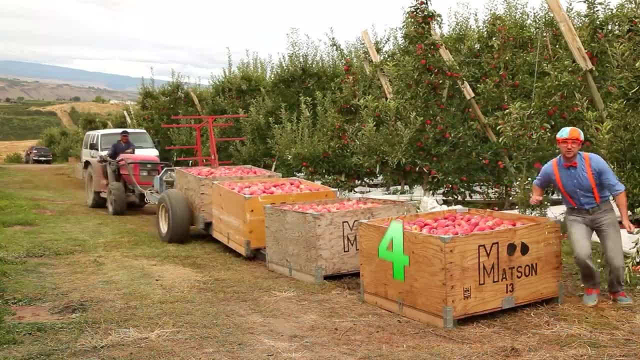 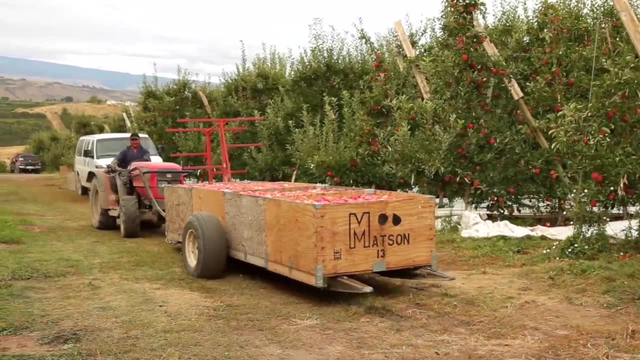 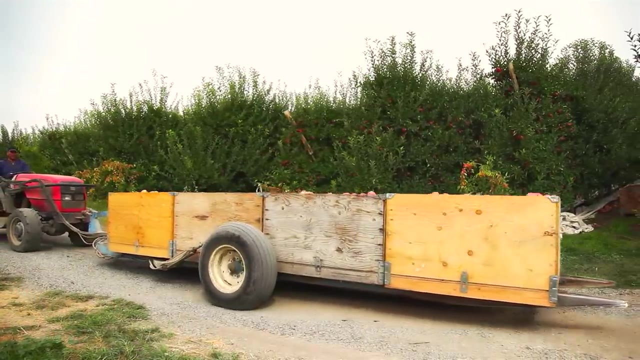 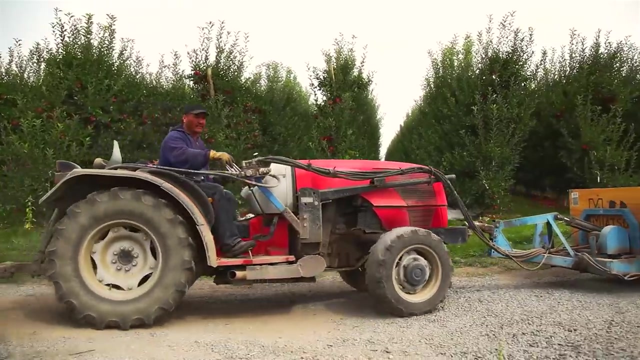 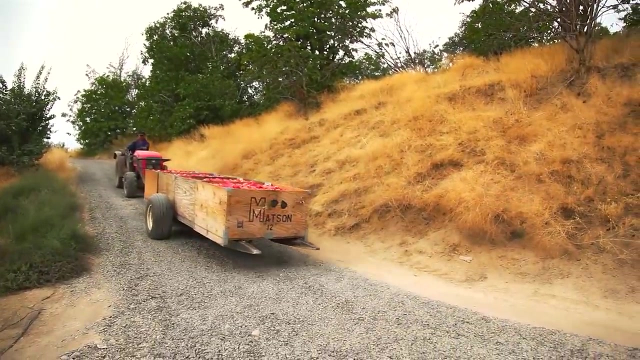 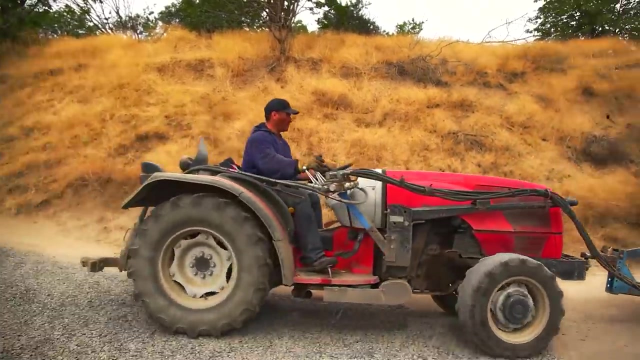 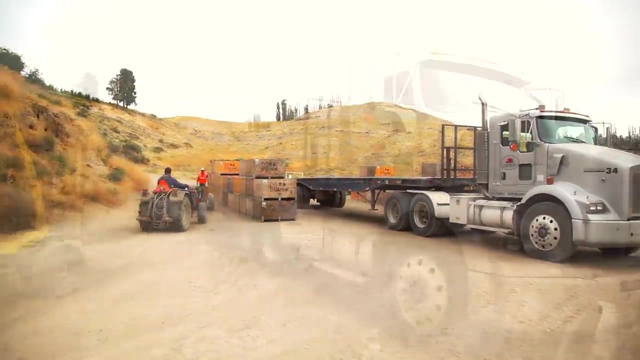 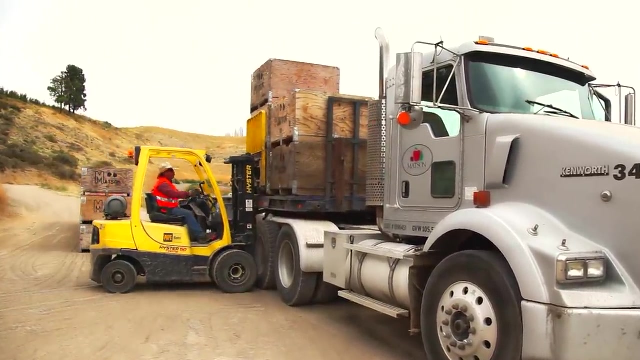 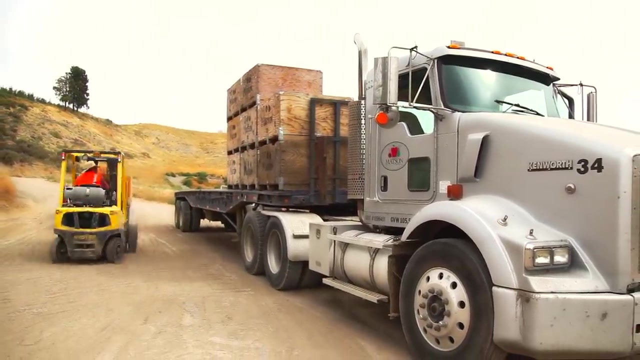 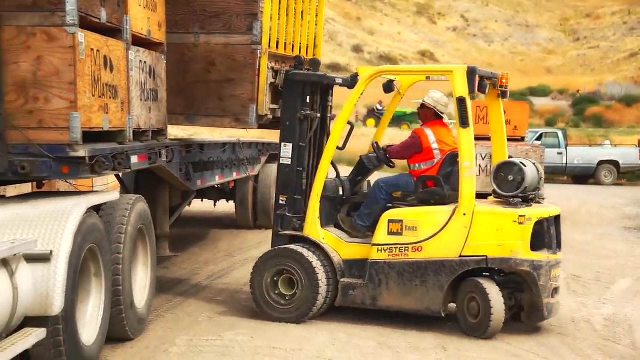 Oh yeah, Oh yeah, Oh yeah. Let's go back up to the trucks. Wow, Four giant bins full of apples And one red tractor. Okay, the apples are now here at the semi-truck. Now we gotta load up all the bins on top of the back of the semi-truck with a forklift. 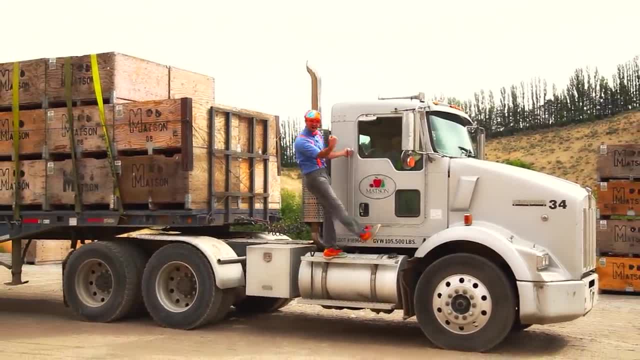 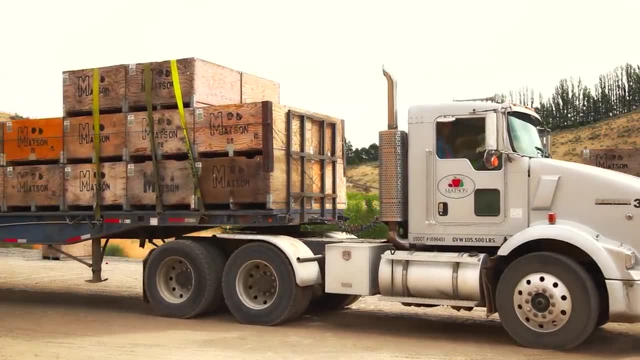 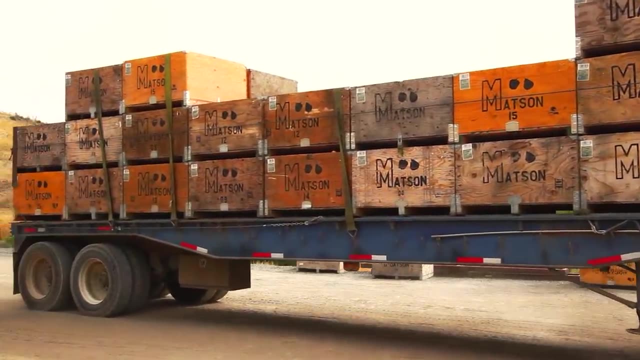 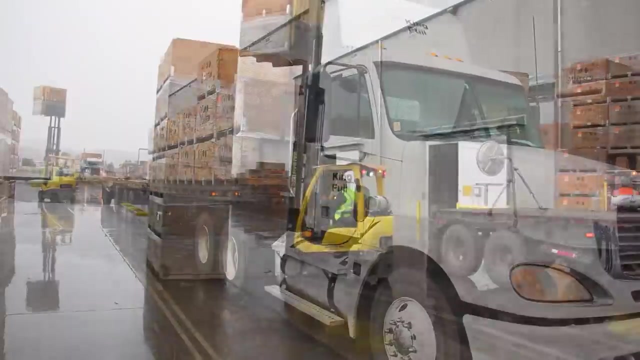 The bins are loaded on the back of the truck, so let's go Off to the factory we go. We've arrived at the factory, so now we need to take a forklift and get every single bin off the back of the semi-truck. 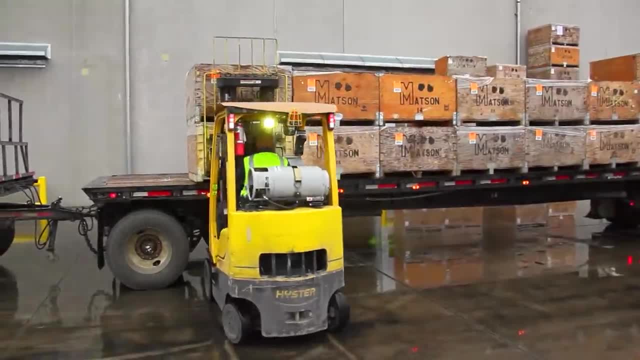 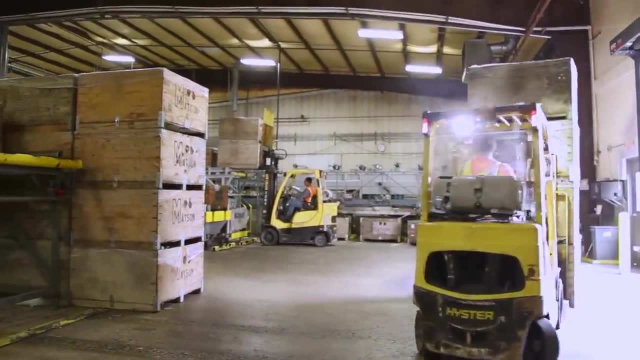 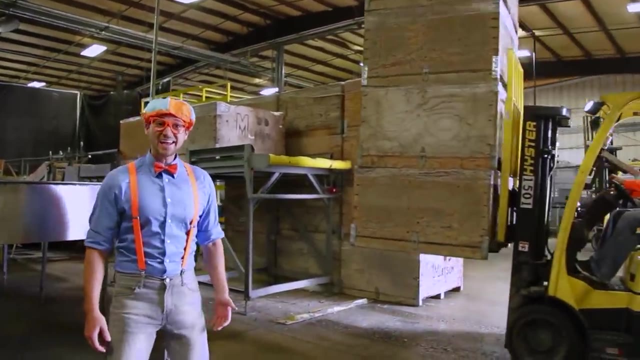 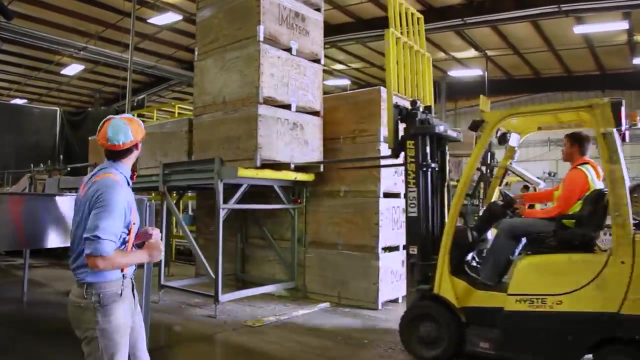 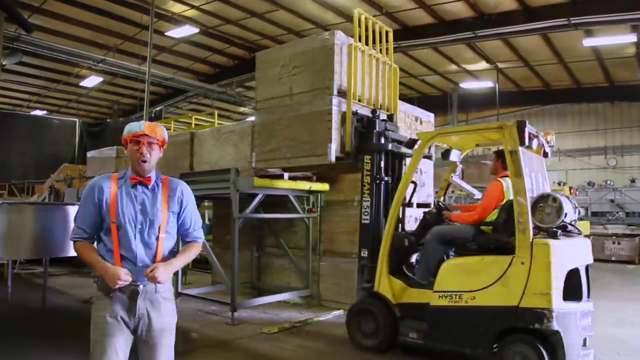 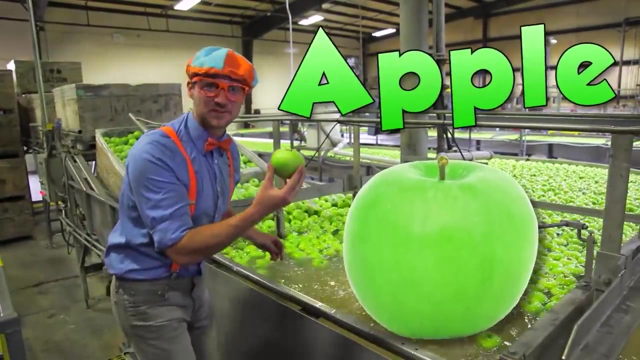 Let's go. Okay, now it is time to clean and package all of the apples. Okay, now we're ready, Let's go. Let's go. Green apples: now we need to empty the bins of all of the apples so we can clean them. 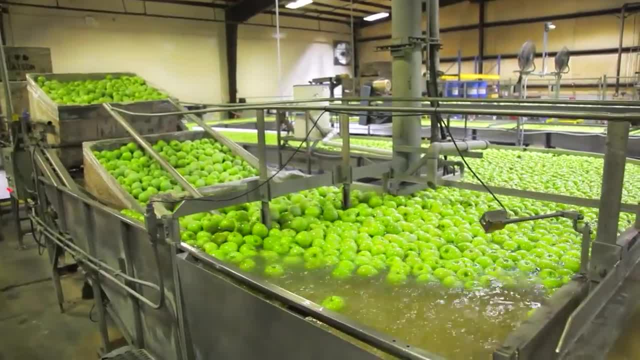 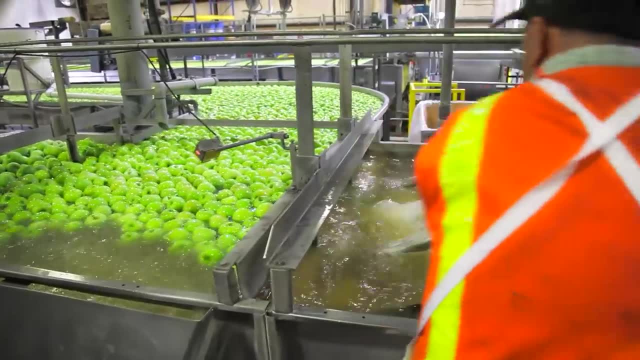 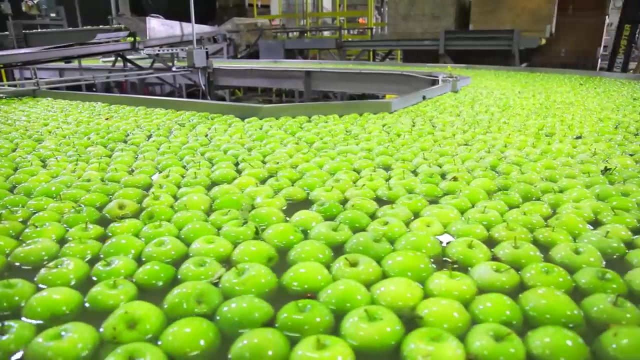 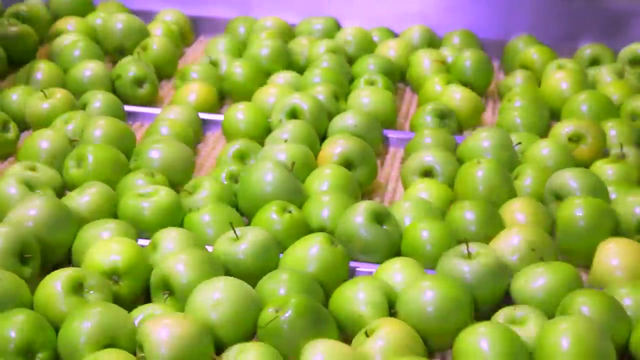 and package them. The apples start their floating journey while the bins get emptied out. Look, the bins are empty. Whoa, that's a lot of floating apples. Then they get taken out of the water and scrubby-dub-dub: nice and clean and cleaned some more. 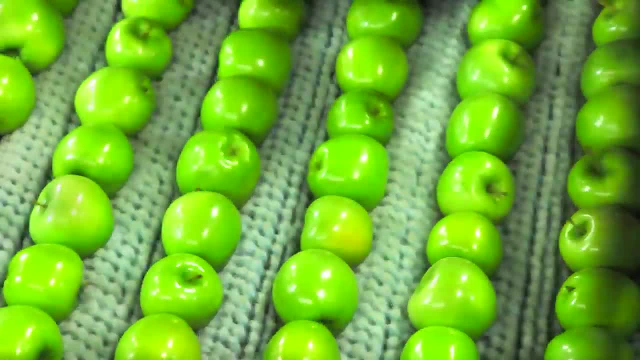 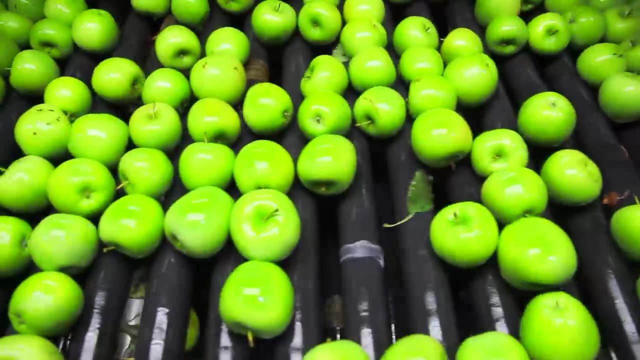 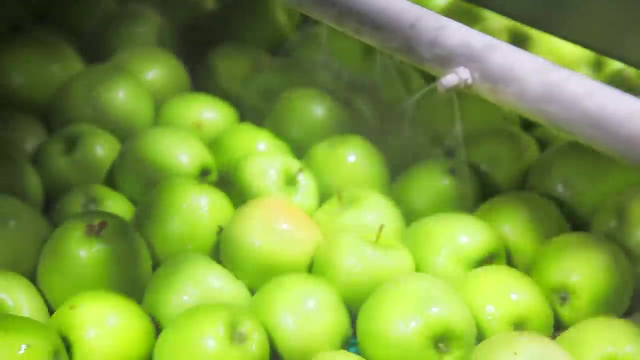 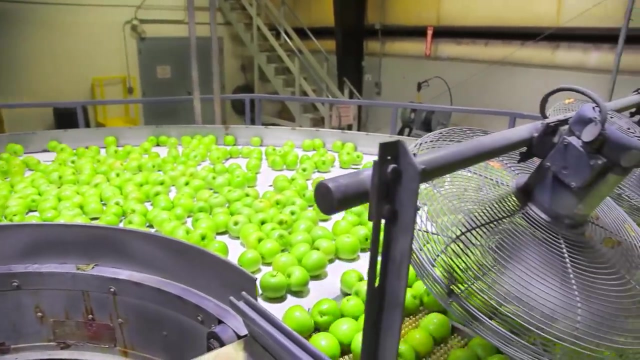 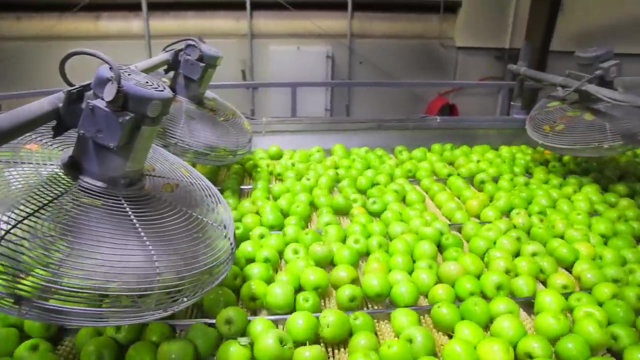 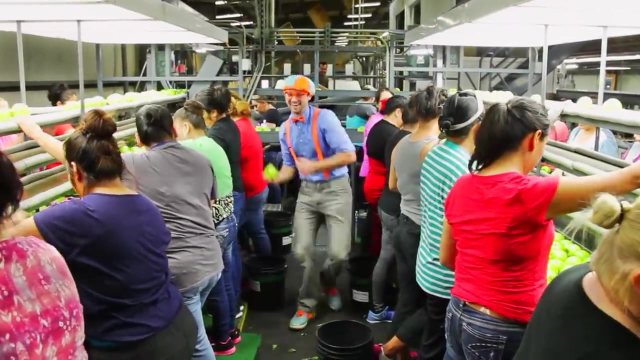 Look at all those bristles, Whee, Those apples look like they're happy, They're having fun. And then all the apples get sprayed with some water, Nice and clean, And then they go through giant fans. Once the apples are all dry, they get sorted. 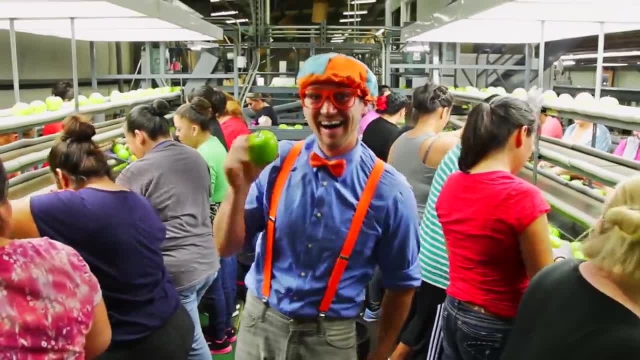 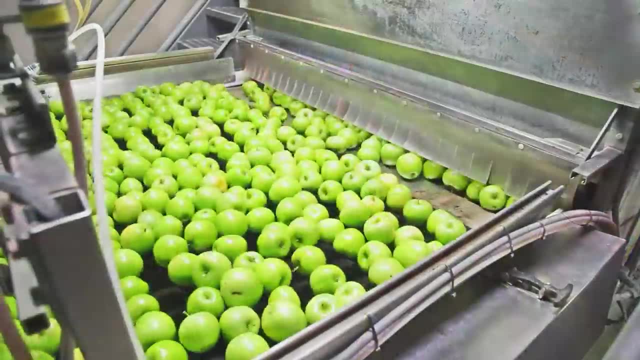 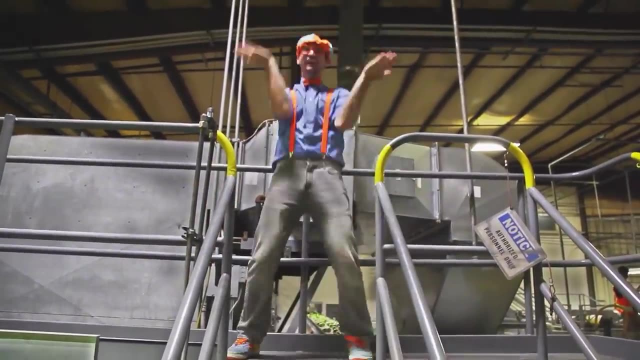 They get sorted by the ones that look really tasty to eat and ones that don't look tasty. They get sorted by the ones that look really tasty to eat and ones that don't look tasty to eat, And remember the not-so-tasty-looking apples. 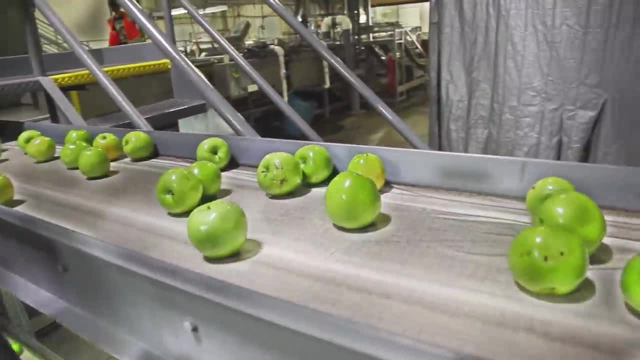 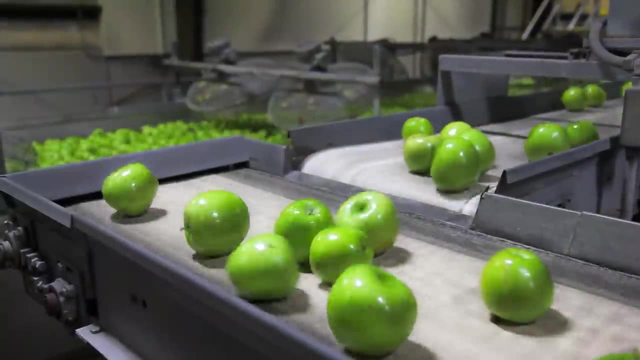 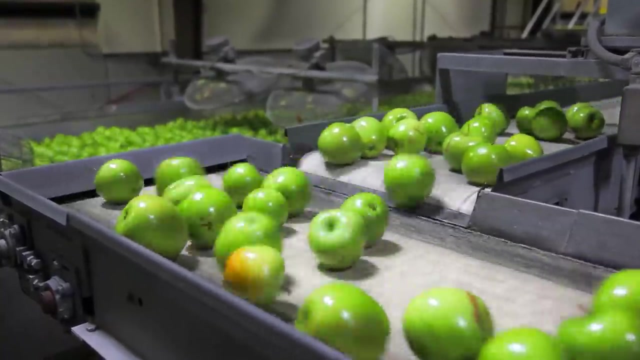 Yeah, these are them. They get to go up some fun apple escalators And then they get to go down some radical apple conveyor belts on their journey to make some tasty apples- apple pie. But we're not done there yet. Every tasty looking apple gets a sticker. 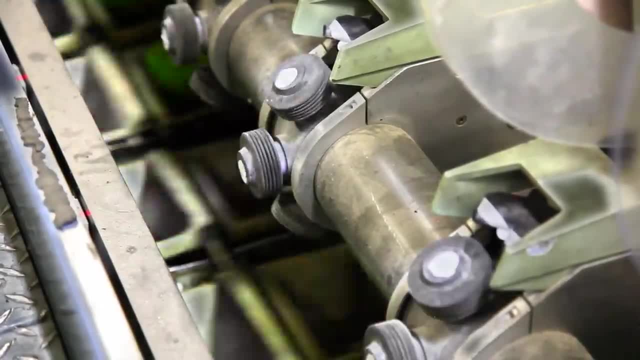 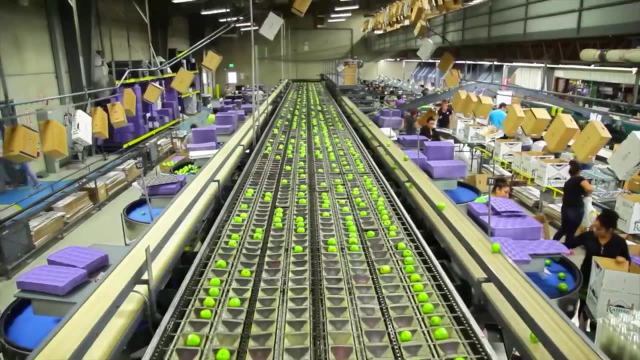 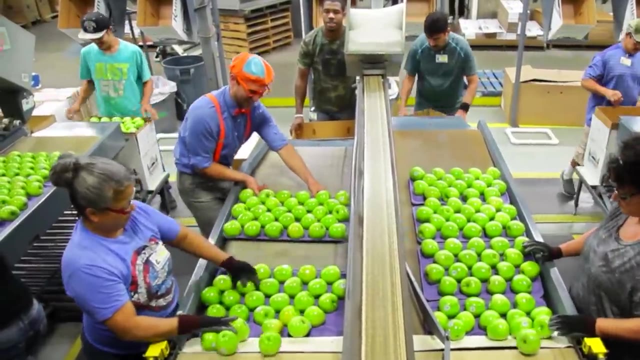 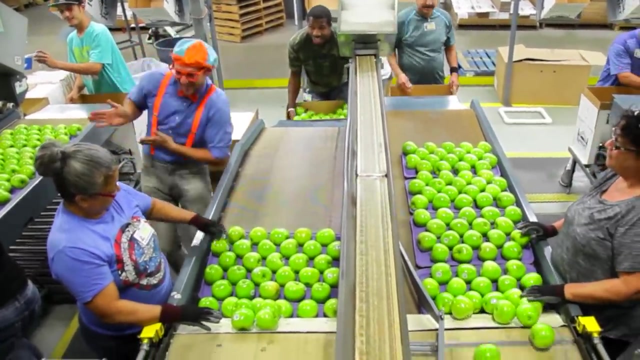 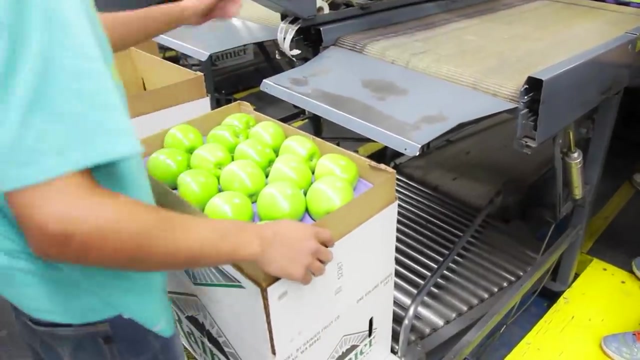 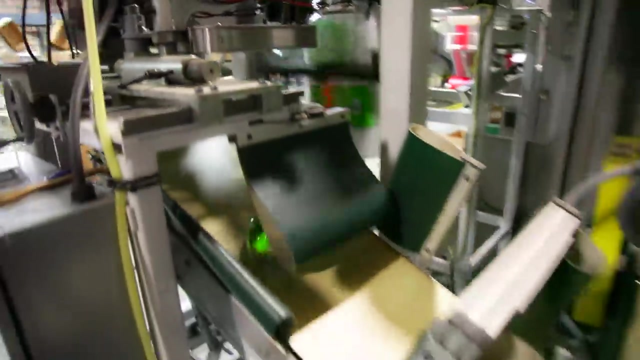 This is the sticker machine, And once every single apple has its very own sticker, they get put on what I like to call apple beds. And then the next step is that those apple beds get put inside of cardboard boxes, And some get put inside plastic bags. 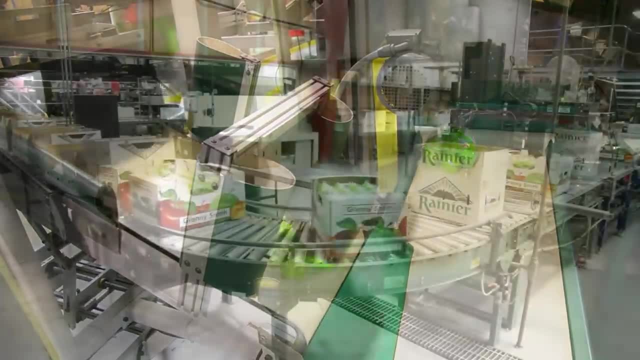 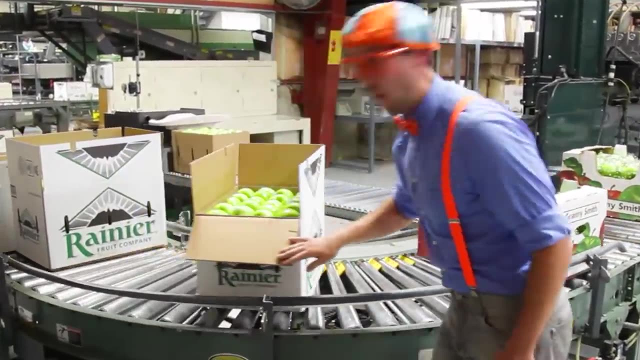 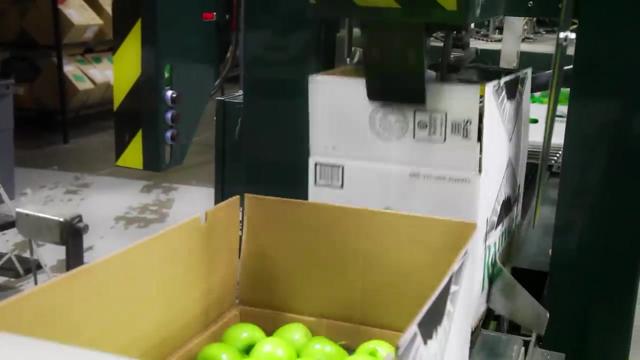 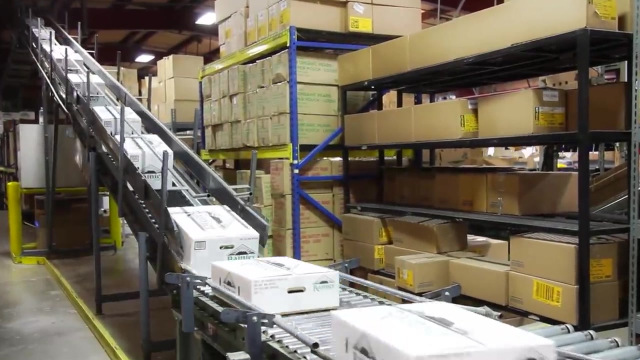 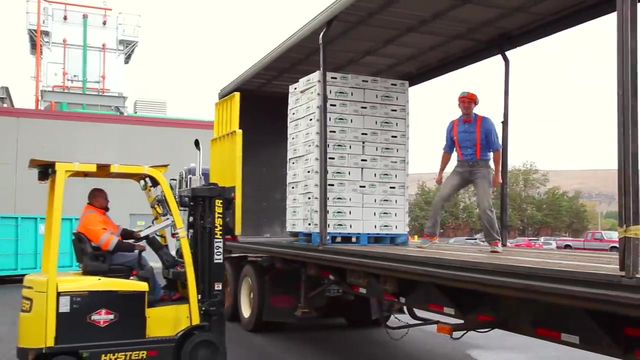 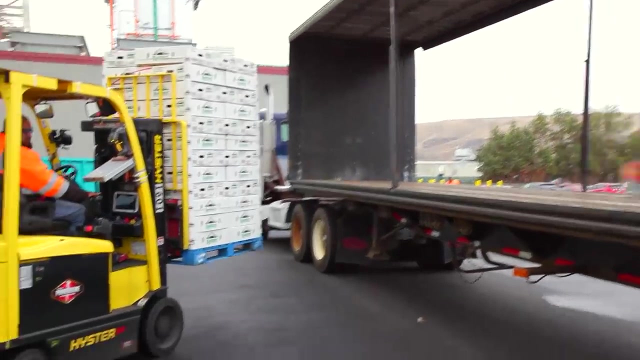 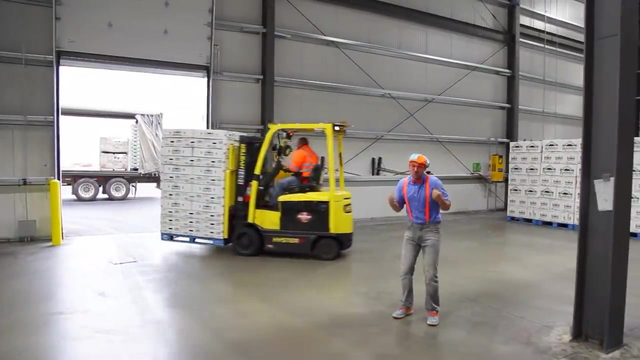 Oh, looks like some of these boxes need their tops closed. Now that the apples are all clean and packaged up, we've got to store them in a giant refrigerator and wait for the trucks. Grrr, We're inside the giant refrigerator now. 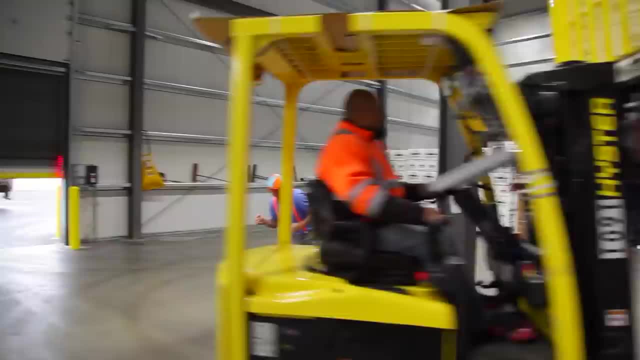 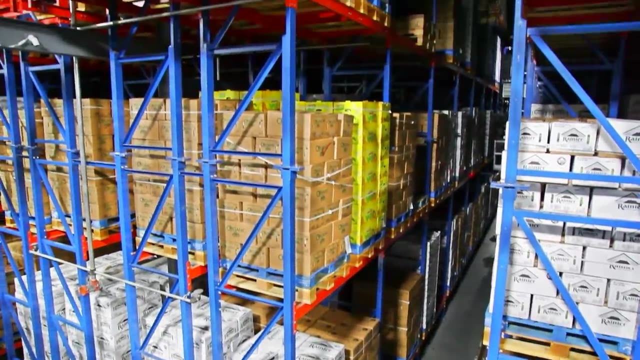 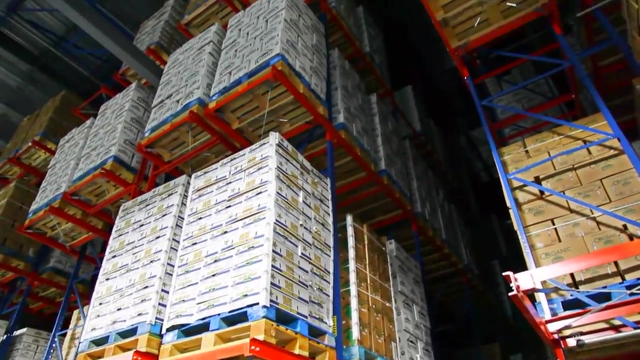 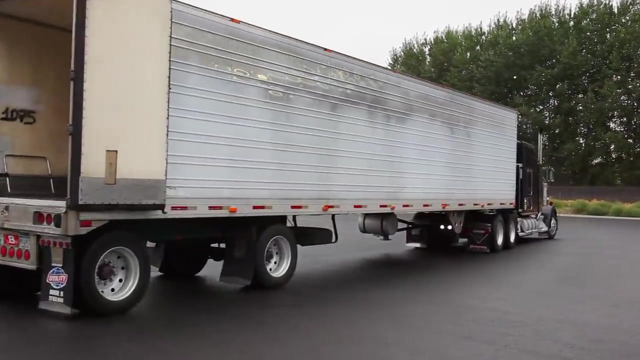 It is very cold in here. This is where all of the apples get stored. Wow, Look at how many apples there are. That's a really tall storage building. Yippee, The semi-truck is backing up to the building so it can be loaded up with a bunch. 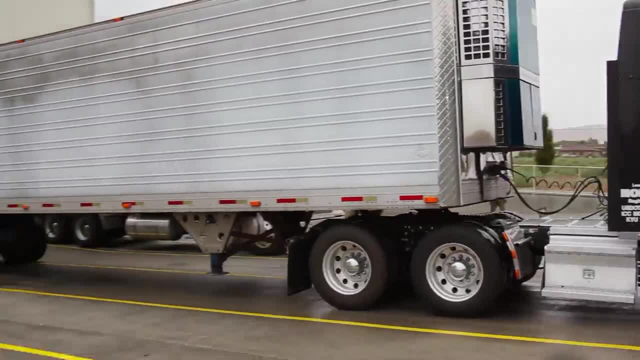 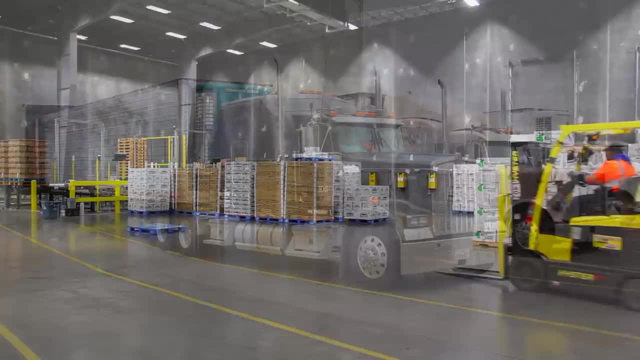 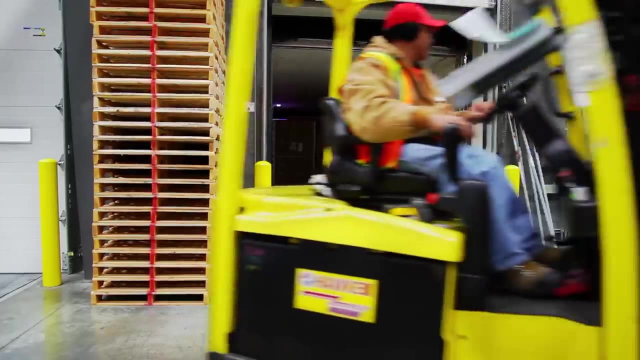 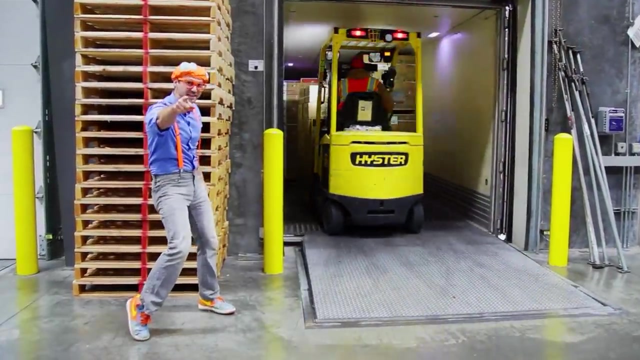 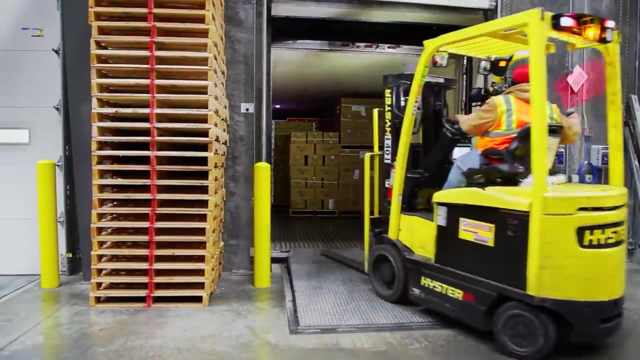 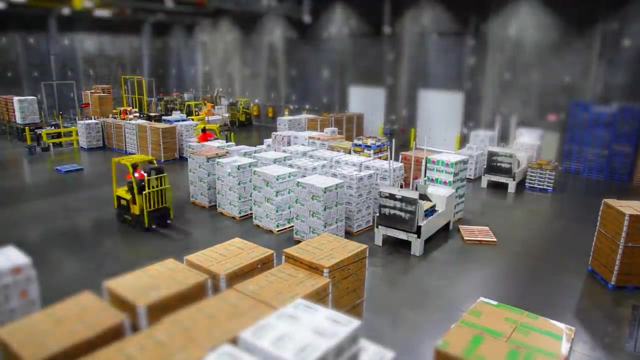 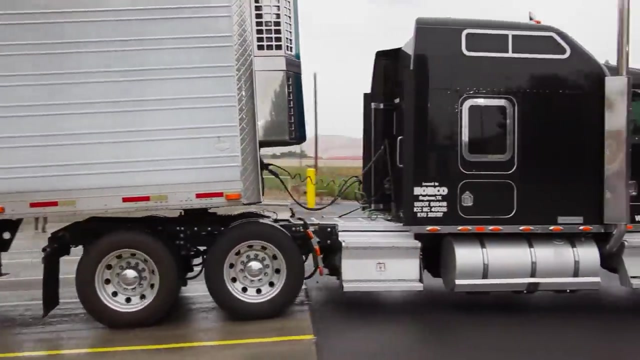 of fresh apples. The apples are almost ready for you to eat. We're currently loading them into the back of the semi-truck. Alright forklifts, Just a little bit more apples. Now that the semi-truck is all full of apples, it's going to deliver them to the grocery. 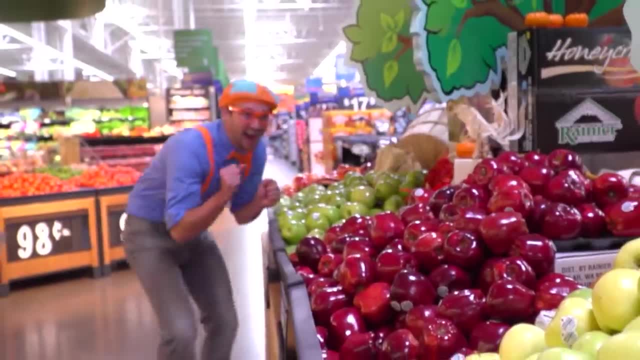 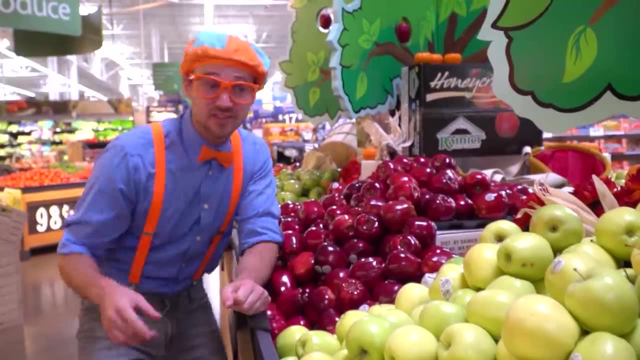 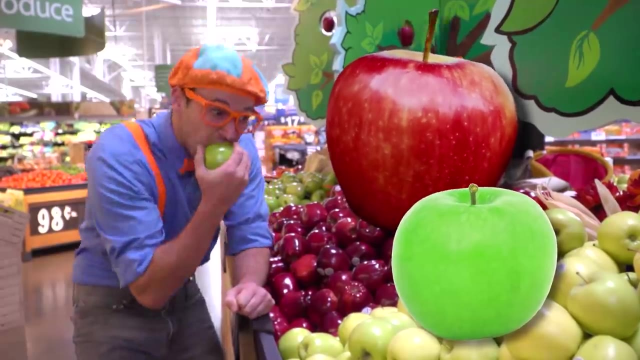 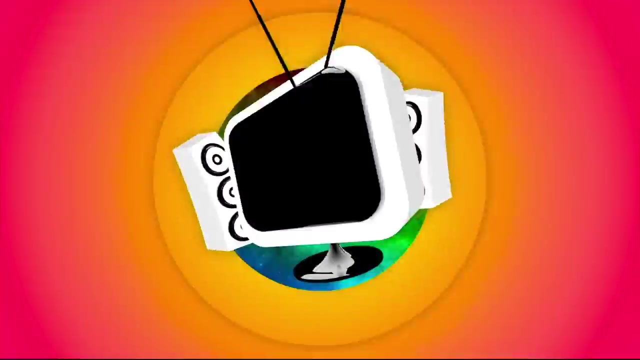 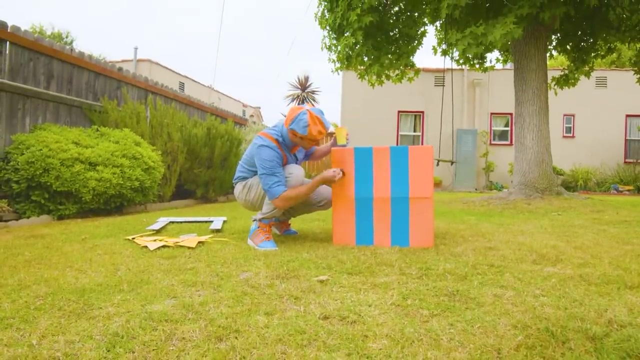 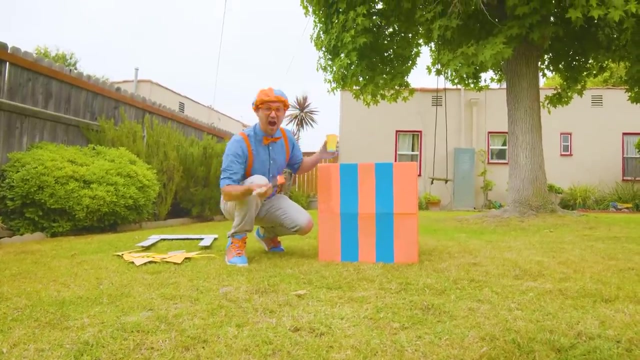 stores. Ooh, it was sure fun seeing how apples get to the grocery store with you And remember an apple a day keeps the doctor away. So much to learn about. It'll make you want to shout Blippi. Oh, hey, It's me Blippi. Do you see what I'm doing? I'm painting. Yeah, I'm actually. 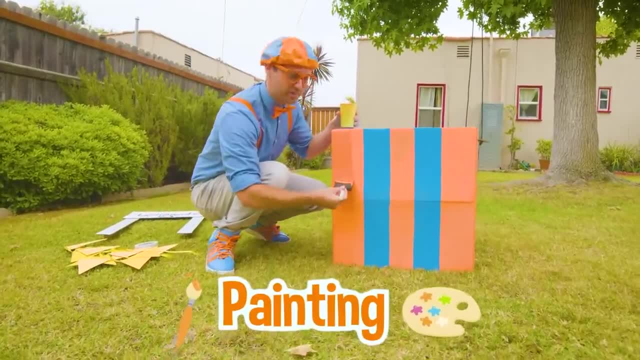 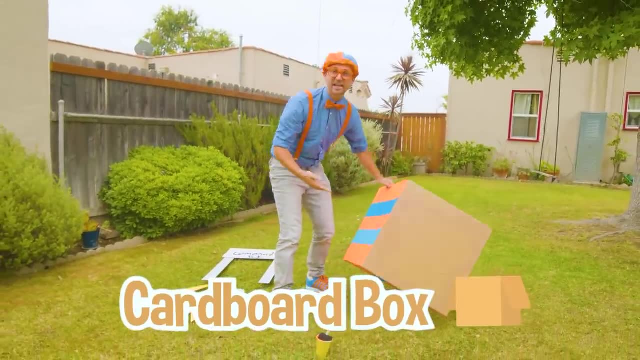 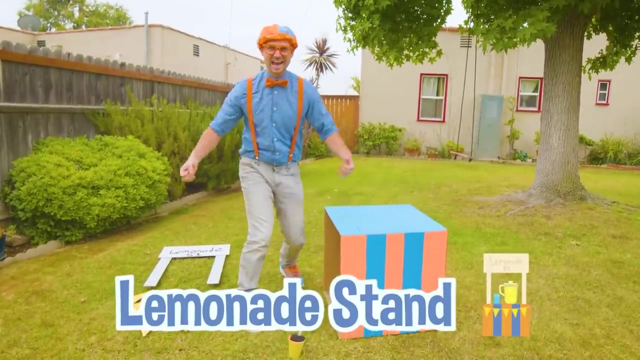 painting just a regular cardboard box. Check it out, See. I took this cardboard box and I'm painting it. Do you know what I'm painting and making? I'm actually going to make a lemonade stand. Yeah, I love lemonade, It's so yummy. But 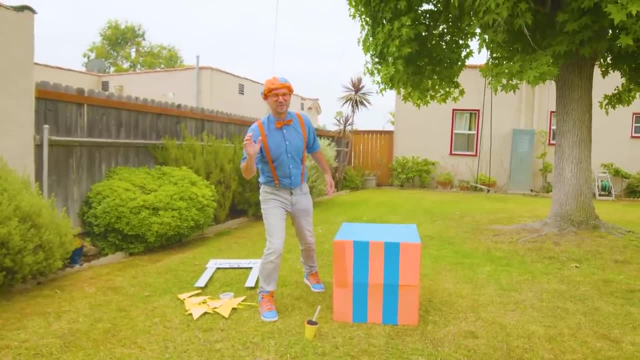 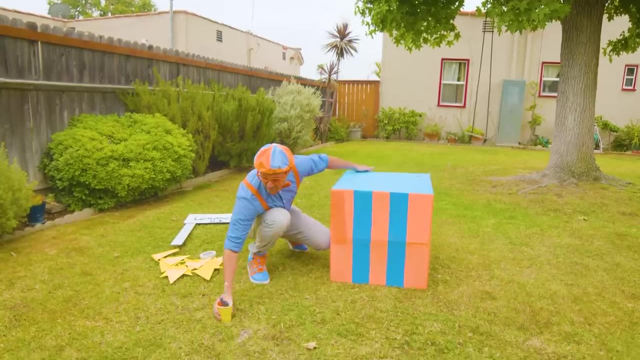 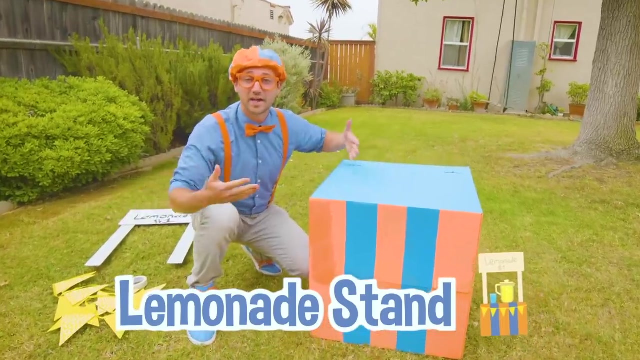 a lemonade stand isn't used just to drink your own lemonade It's, so then you can sell lemonade to others, Yeah, So the first thing that you have to do is make a very good-looking lemonade stand, so then everyone will want to come try your lemonade. So, now that it's all painted, I 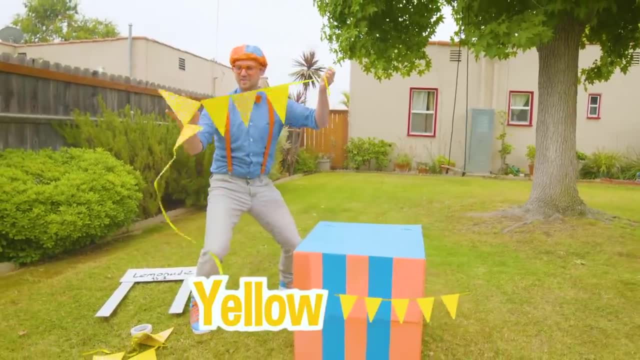 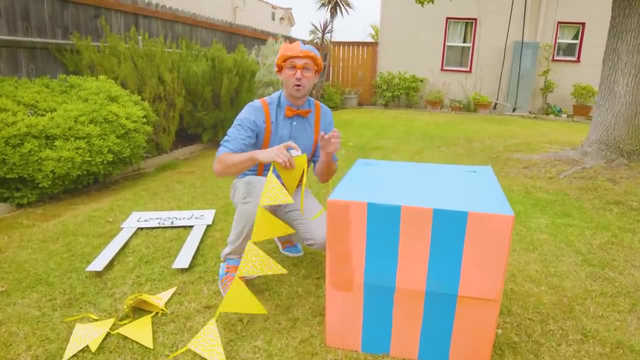 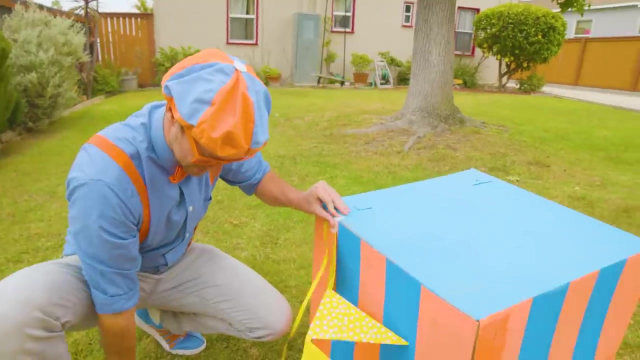 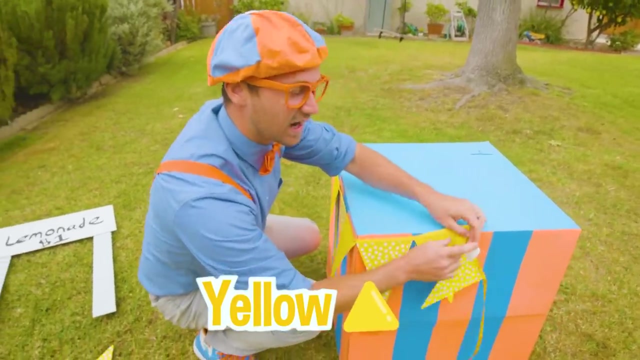 have these yellow triangle ribbons And if I put them on here on the top, it will spark some more customers. Okay, Let's put some tape right here. There we go. Wow, All right, You see these yellow triangles. Yeah, What is the color yellow that? 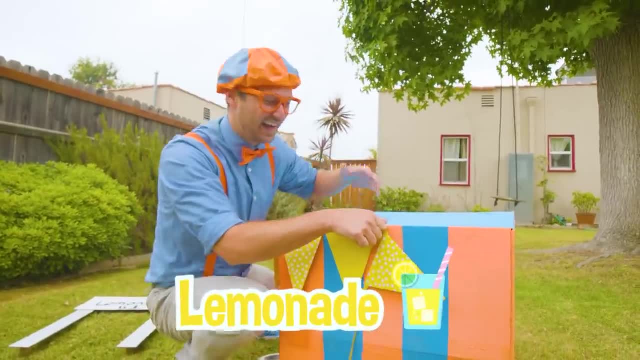 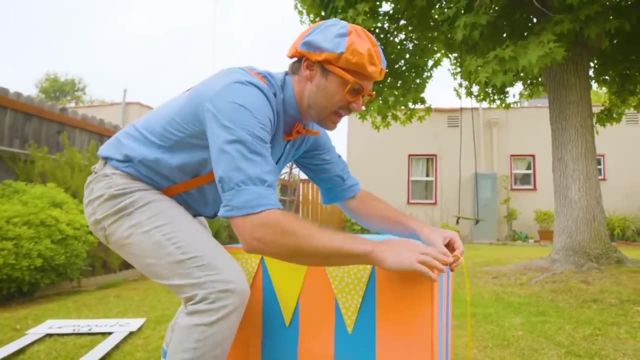 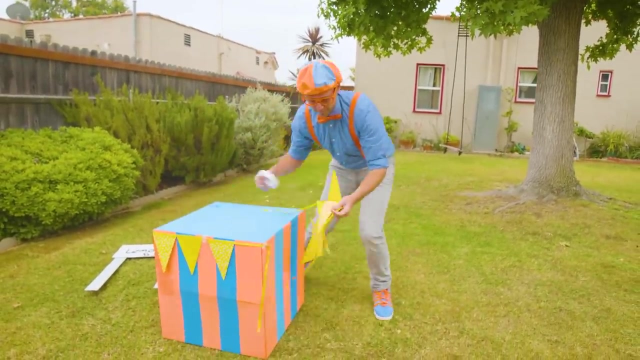 you can think of Lemonade Also. the sun is the color yellow. Okay, Here we go. Then we actually have a little bit more of this. Wow, Have you ever tried lemonade before? Yeah, Maybe, Yeah, Let's try it. 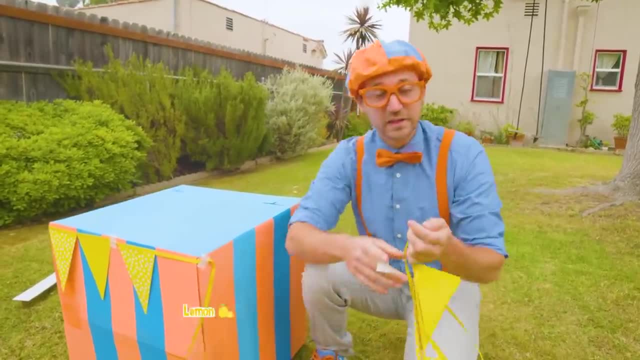 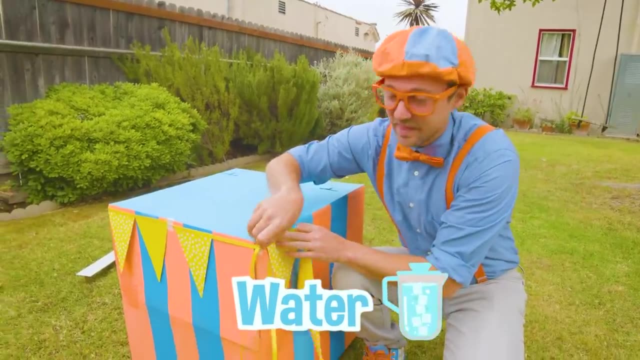 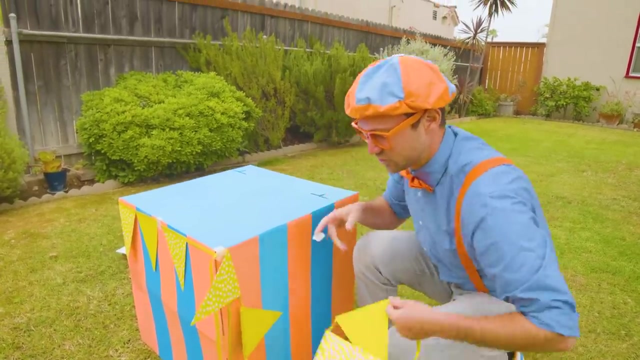 I don't know Definitely. What do you think? It really looks pretty good. It looks like a really tasty. It's weird because if you just eat a normal lemon it's really sour, But if you add a lot of water and then some sugar it'll sweeten it right up and make a nice 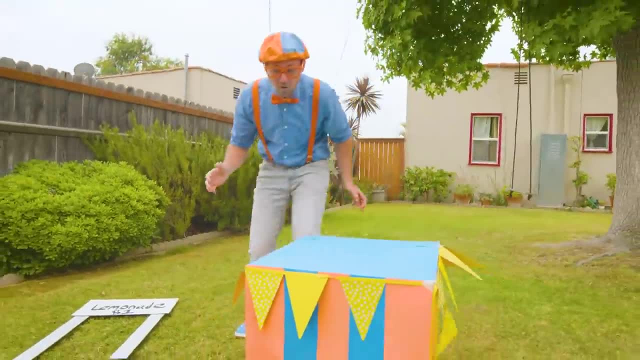 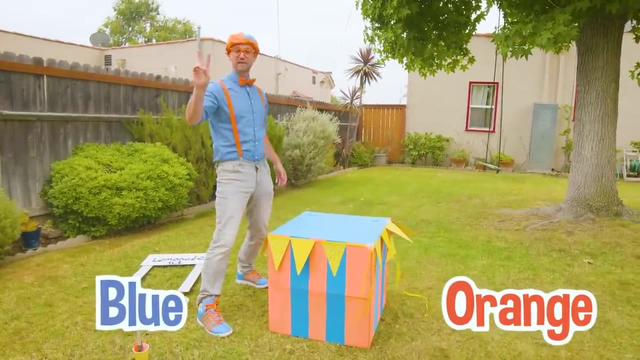 refreshing drink. Okay, How about, right there? Whoa, It looks so good. All right, we have our lemonade stand. blue, red, green and purple. Let's give it a shot. and orange- my two favorite colors. we added the yellow banners to bring in. 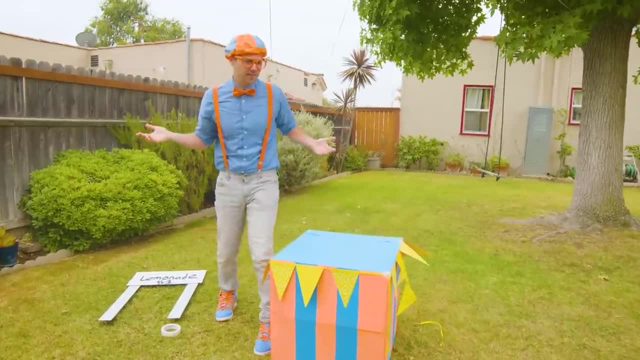 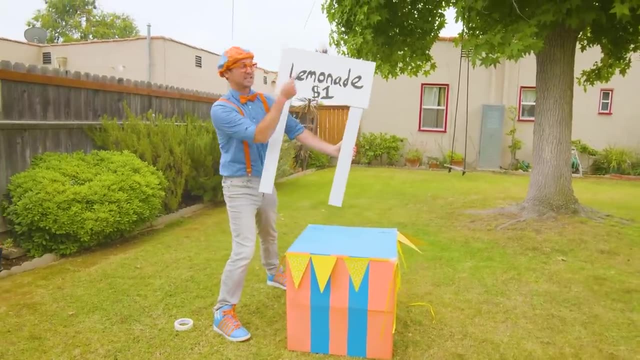 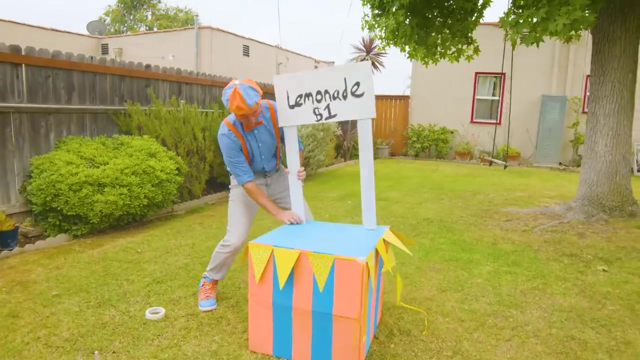 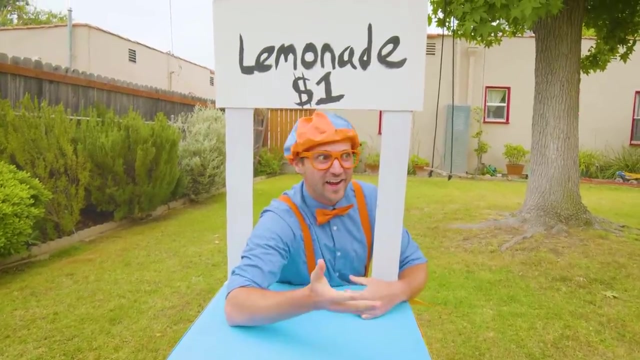 more customers, but all these customers are gonna be like: what's Blippi doing? so we need to tell them what we're doing. we're gonna be selling lemonade one dollar, so let's put this right here. perfect, how does this look? can you tell what I'm here for? yeah, to sell lemonade. all right, now that we built the stand. 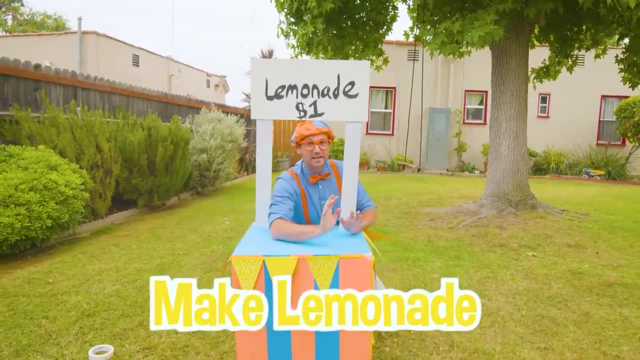 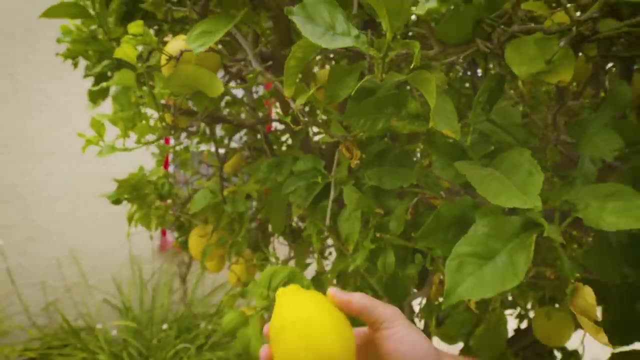 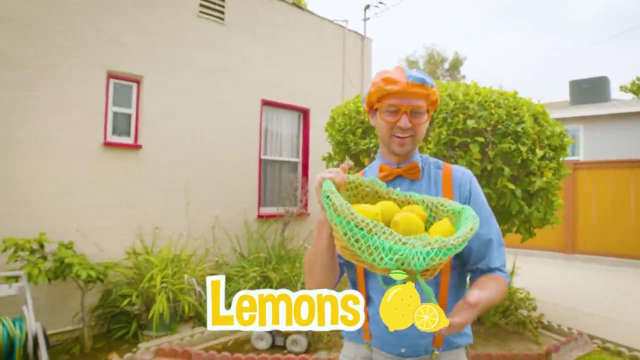 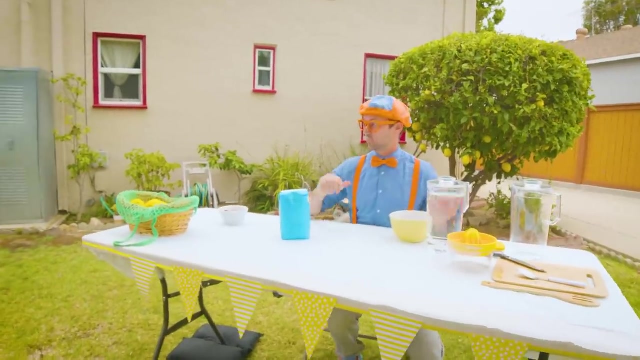 now we need to make some lemonade and then we can sell it. yeah, let's go. yeah, the first ingredient to lemonade is lemons. there we go, so great that our friend has their very own lemon tree. that definitely saves us a lot of money when we calculate how much this lemonade cost us to make. okay, all right. 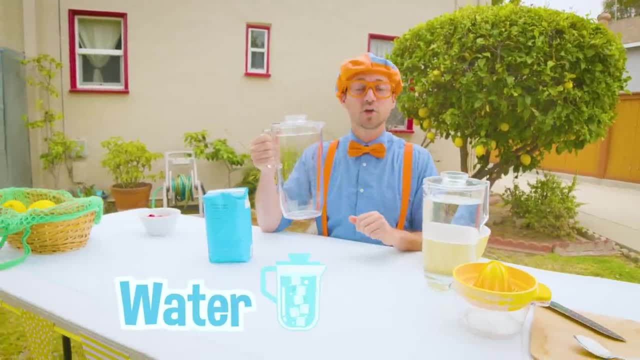 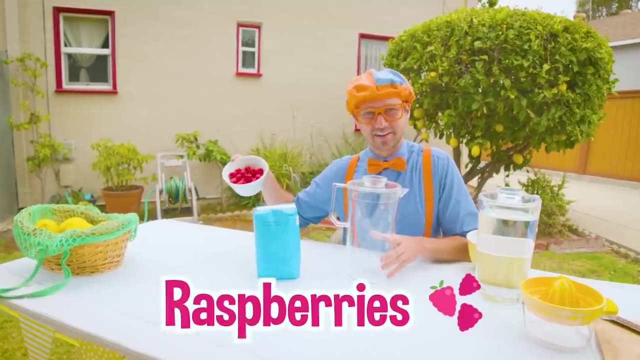 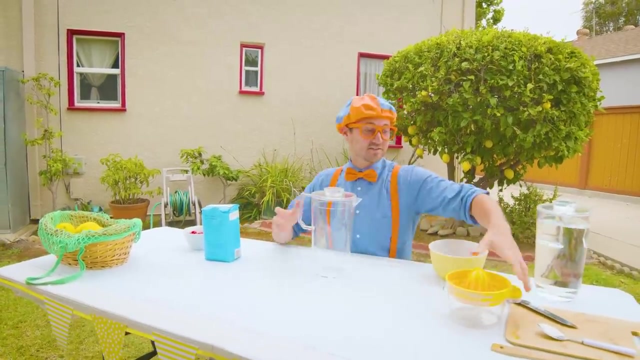 see this picture. we're gonna put a lot of water, sugar, lemons and we're gonna spice it up with a little bit of raspberries to make raspberry lemonade. so the first thing that we need to do is to grab our lemons. yeah, right and only. 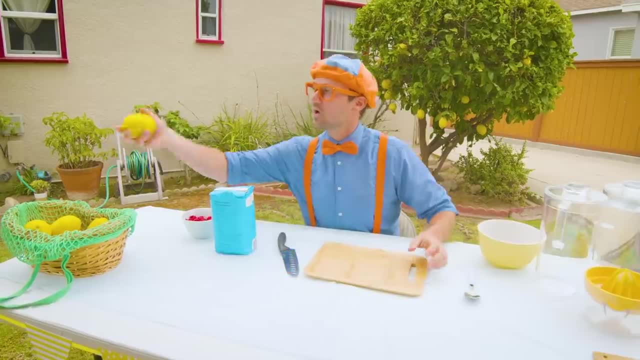 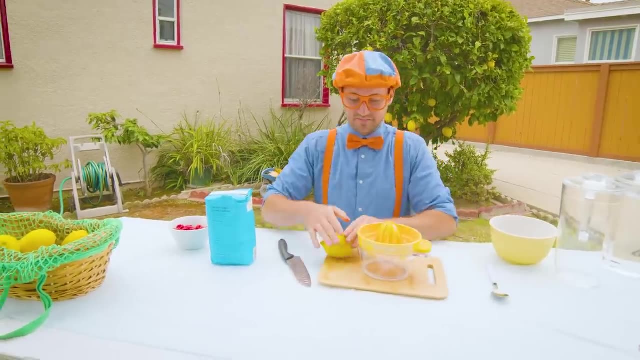 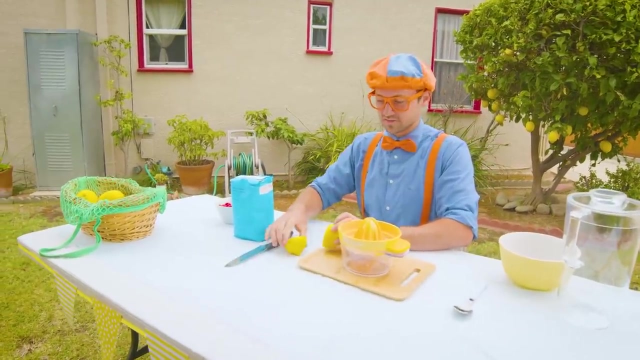 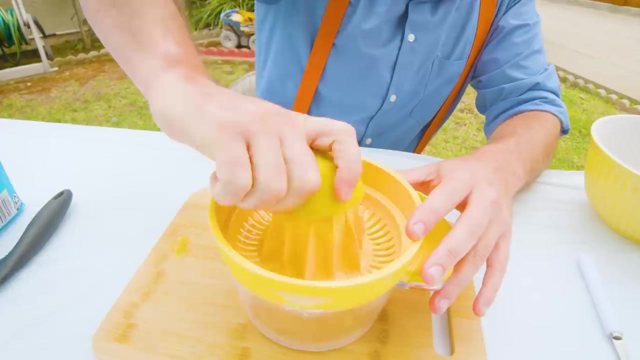 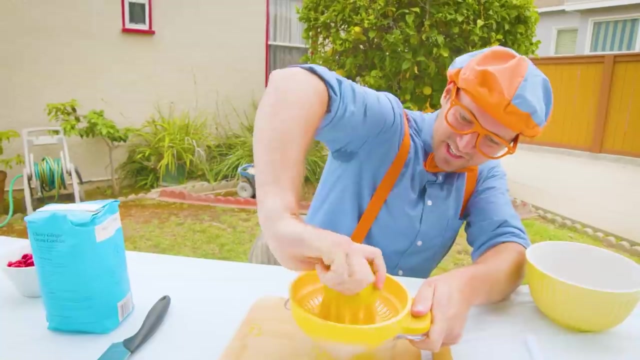 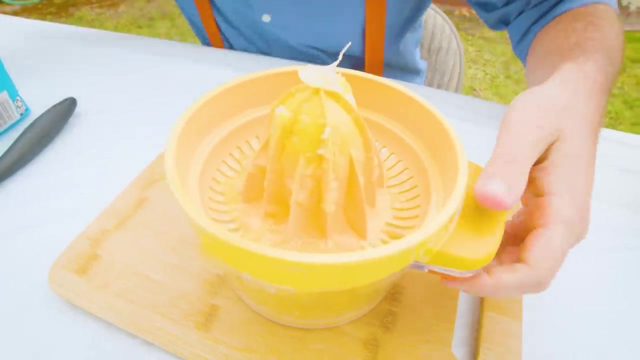 grown-ups should use a knife. so we're going to first take a lemon, we're gonna cut it in half and use this device to squeeze out all of the juice, just like this ready. Wow, yeah, do you see all that lemon juice down there? okay, let's do another. 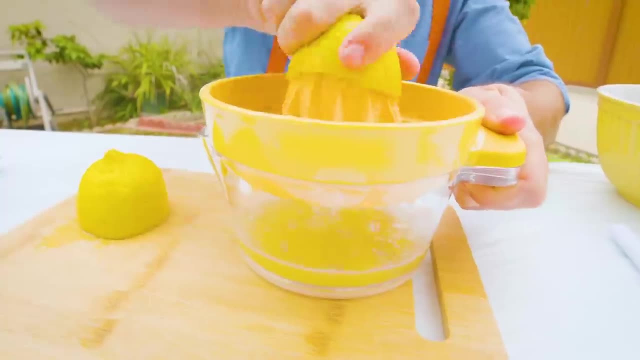 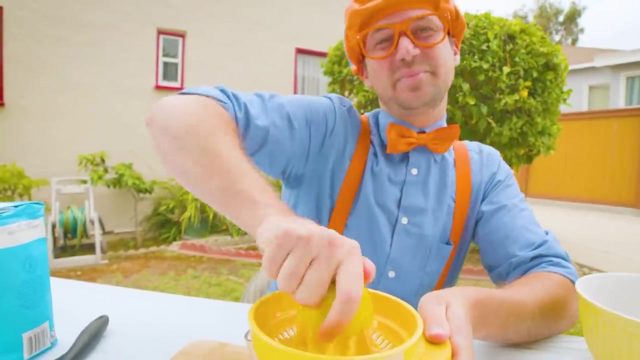 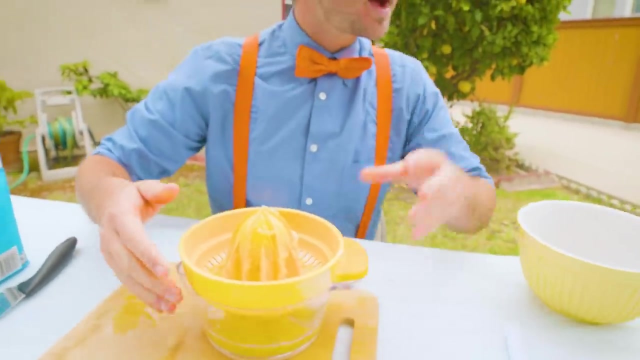 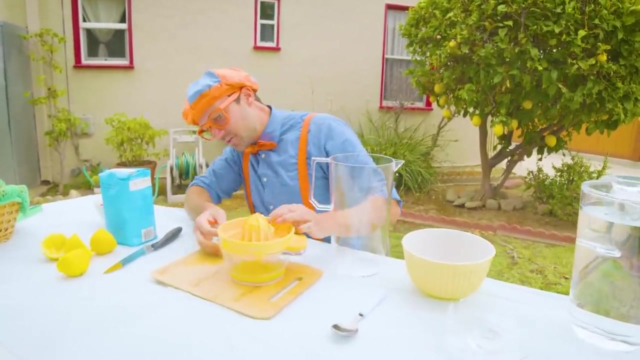 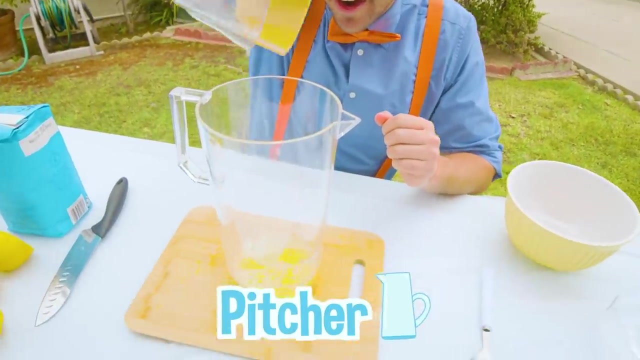 there we go. whoa, this thing is just pressing out all of the juice. it looks so yummy. I bet it'd be really sour though. all right, I think that is plenty of lemon juice for our lemonade, all right. so we need to now pour this in our giant pitcher. there we go. all right, it has a. 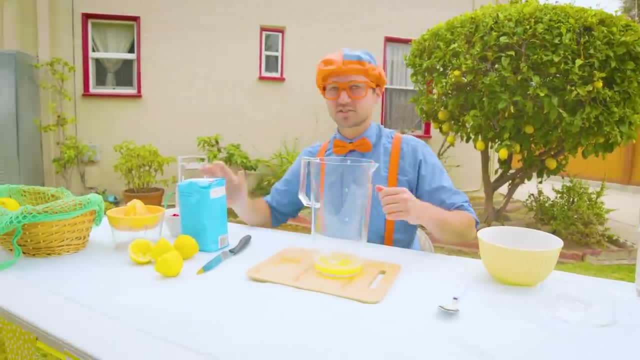 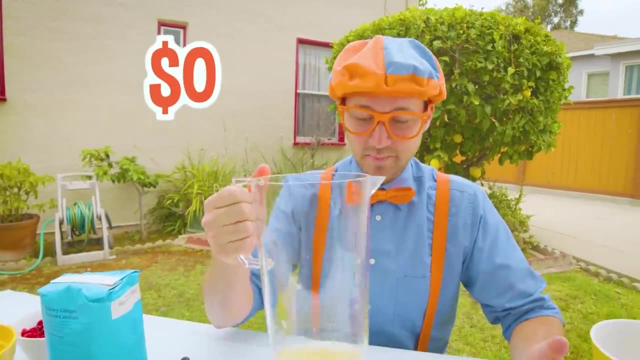 little bit of pulp, but that's okay. okay, so the lemons were free, so we're gonna pour it in our large jar. So that's a lot. So the lemons were free, So this cost us zero dollars to make. we're right on track, okay. the next thing let's add: 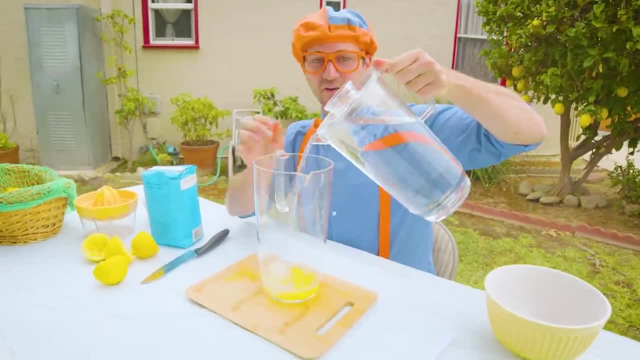 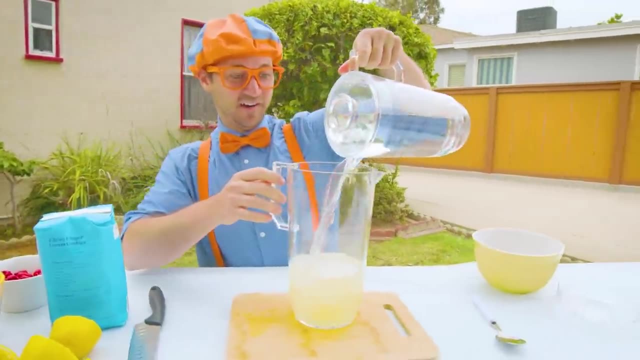 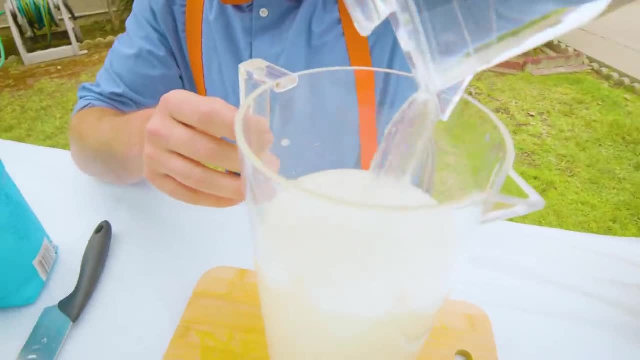 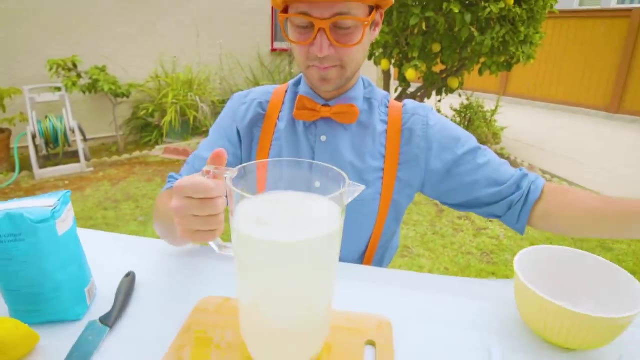 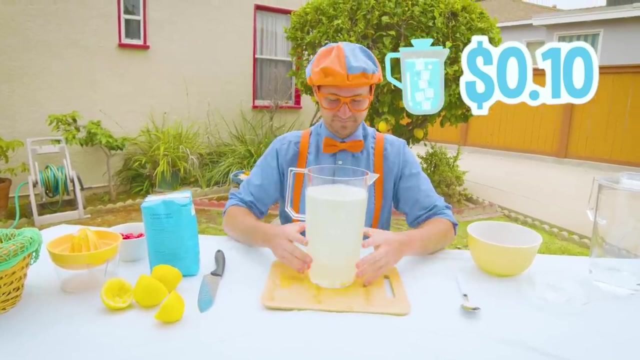 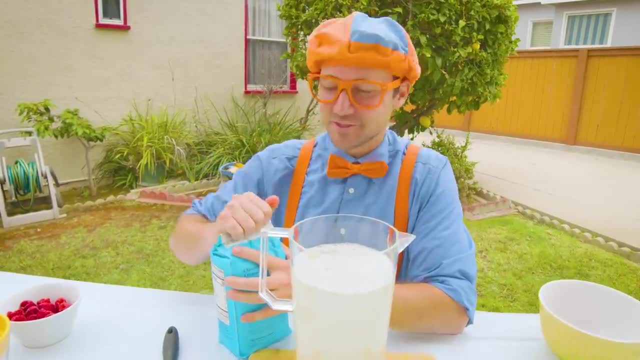 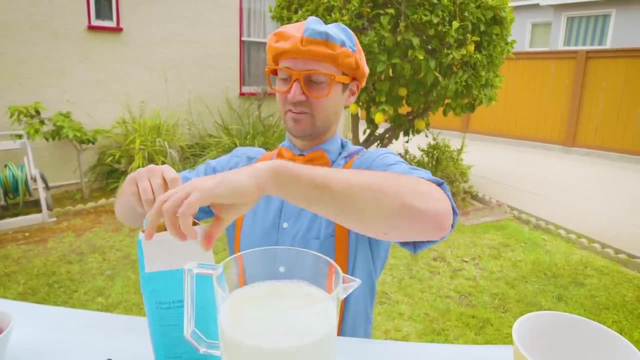 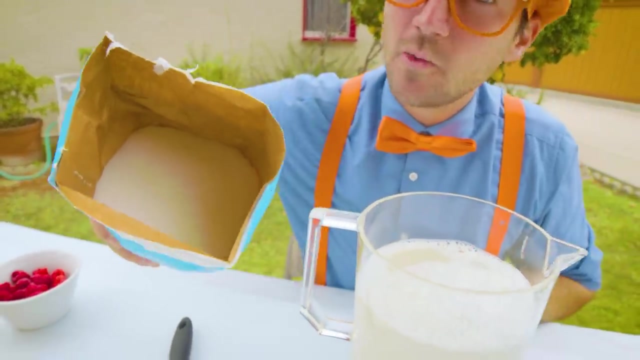 Because this is basically just like watered-down lemon juice, which would be really tart and sour. So what we have right here is sugar. Yeah, That's a really tasty ingredient. You don't want to eat too much sugar, though. 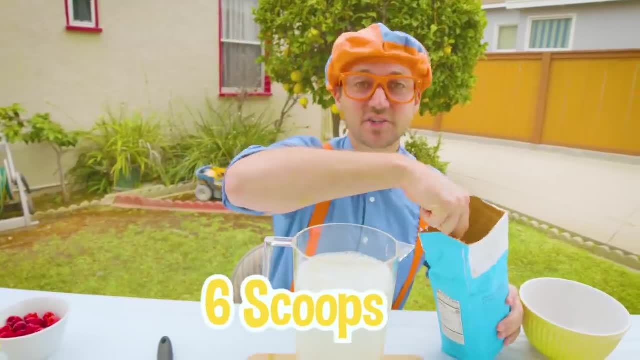 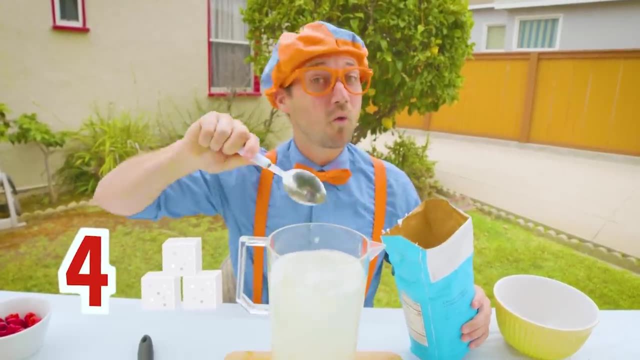 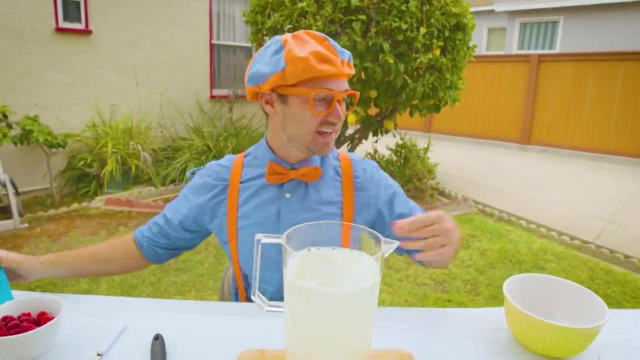 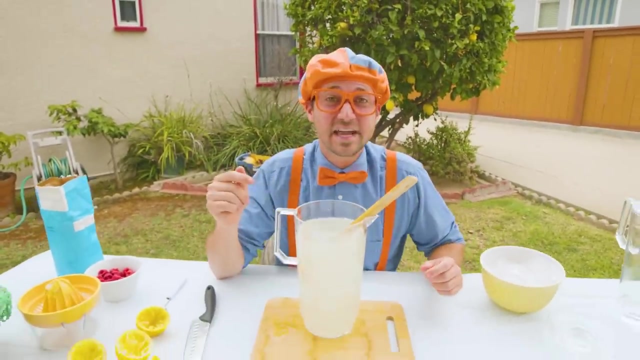 But for the lemonade we're going to add six scoops Ready. One, Two, Three, Four, Five, Six. There we go. Let's put that aside. Here we go. Whoo-hoo-hoo, This lemonade is complete. 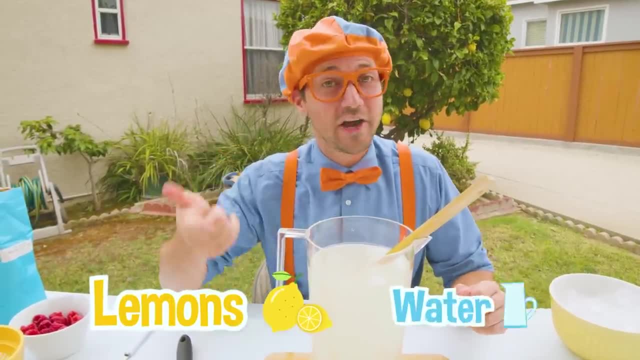 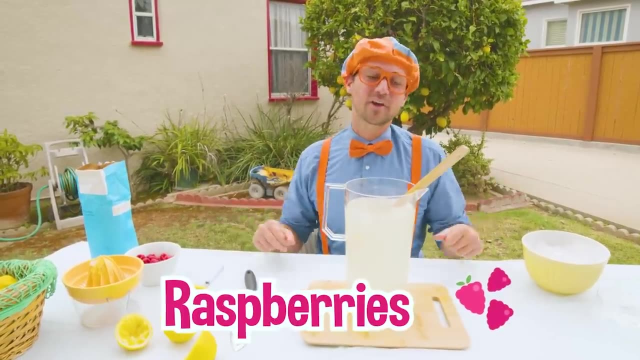 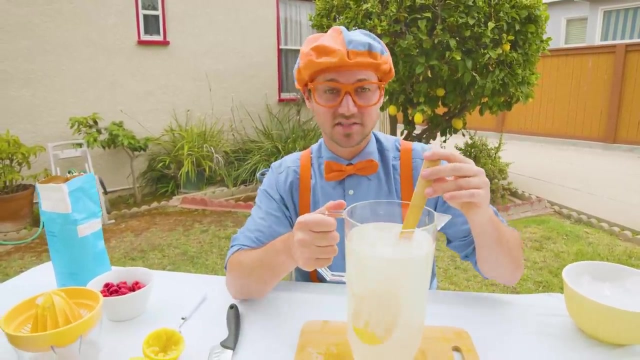 All you really need to make lemonade are lemons, water and sugar, But we have that extra ingredient from earlier. remember Raspberries? Yeah, we're going to make raspberry lemonade, But before we add those, let's calculate how much this lemonade has cost us thus far. 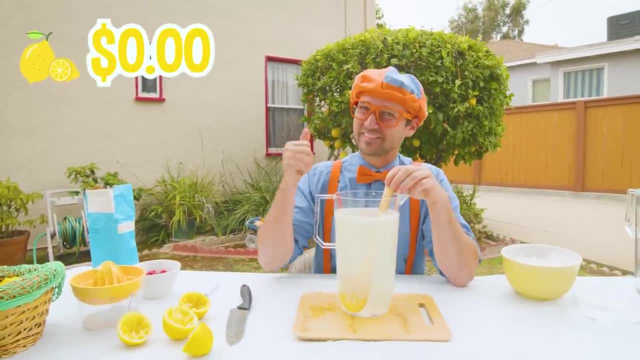 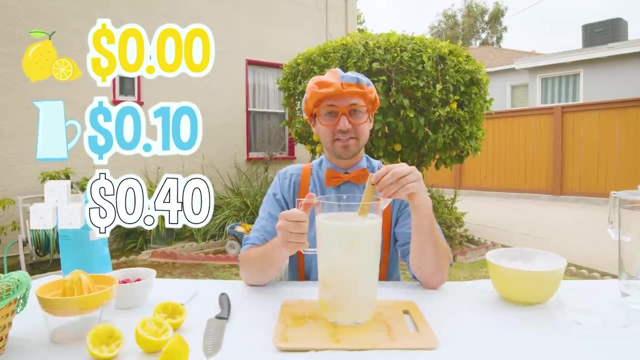 Well, the lemons were free because we have a great friend, Ha-ha. The water was 10 cents and then the sugar was 40 cents, So right now we're at 50 cents for this whole pitcher. Whoa. 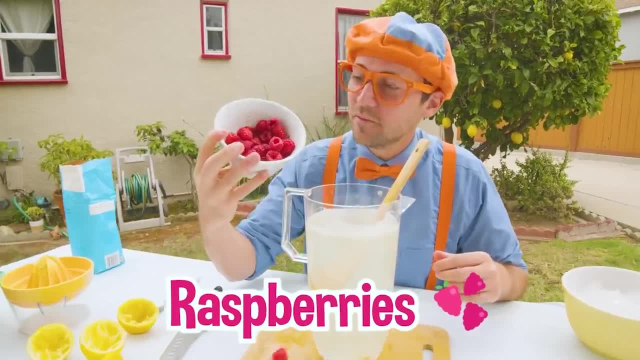 All right, Now we can add our raspberries. Whoo, Oh-ho-ho, Oh-ho-ho. That silly one fell out. I'm not going to touch it, I'm going to just use these Ready. 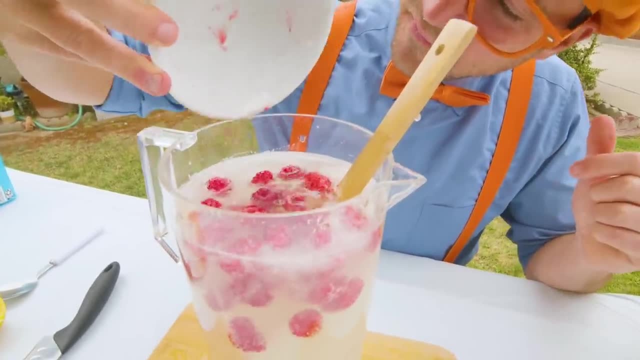 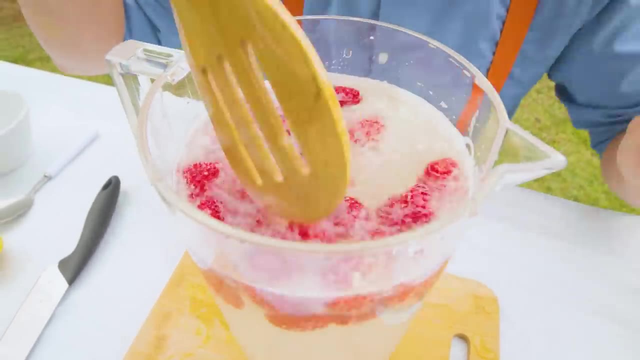 Here we go. Whoa, Looks like they float. Whoa, Oh-ho-ho, Raspberry lemonade, Ha-ha. Okay, So now our total cost. let's calculate. So earlier it was 50 cents. 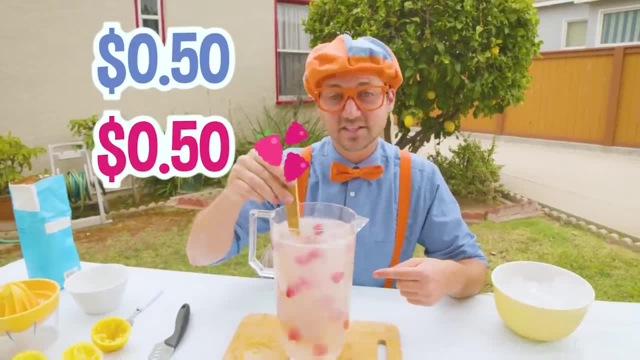 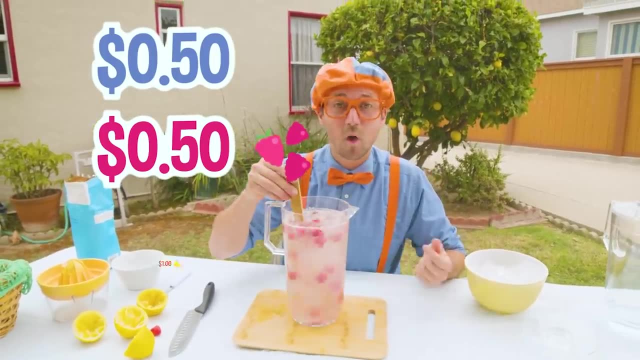 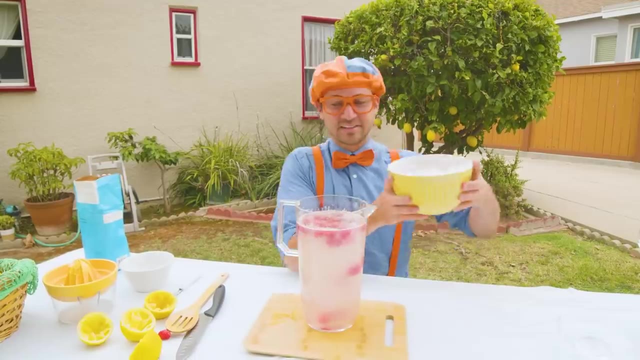 And these raspberries cost me 50 cents from the grocery store. So 50 cents plus 50 cents is $1.. Wow, This whole pitcher cost us $1.. All right, Let's put in some ice Whoa-ho-ho-ho, to chill it down, so then we can go and sell it. 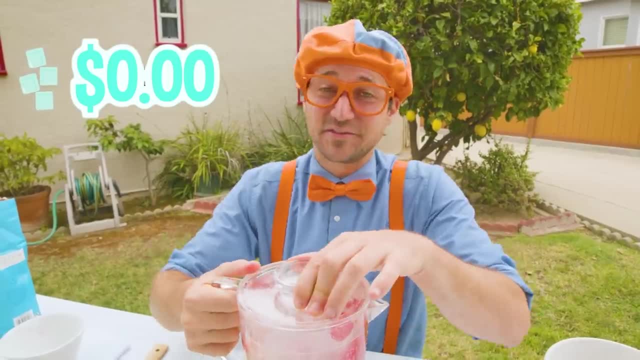 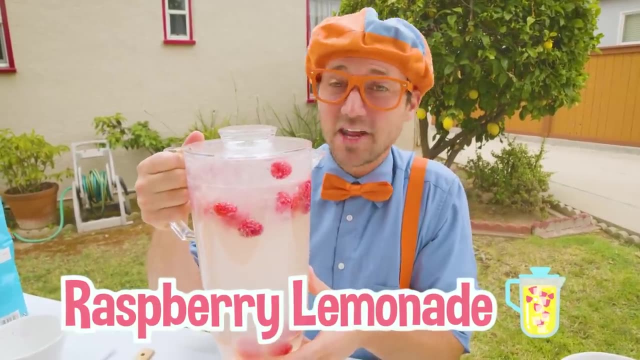 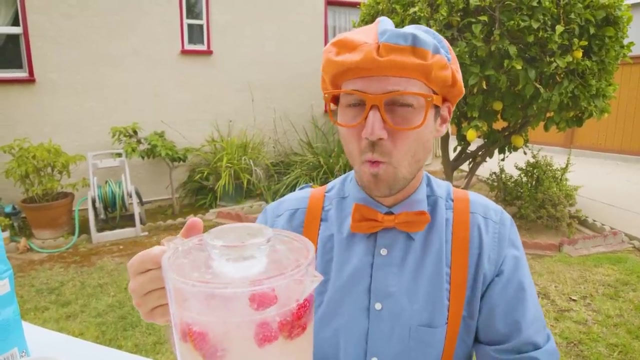 The ice was free because our friend also has a freezer full of ice. So now that we have nice cold lemonade, raspberry lemonade, we can go and sell it. I think there's about eight cups in here And our cost is $1.. 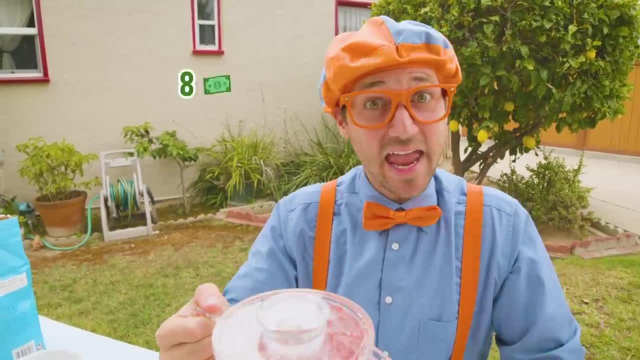 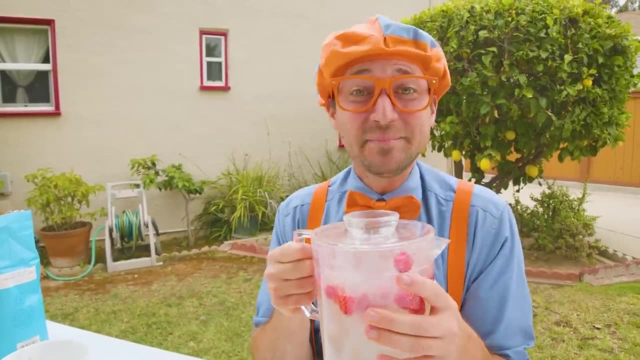 So eight cups. if we sell them for $1, would be $8.. $8.. Oh, And if we minus $1, that's $7.. Whoa, We're going to make $7.. Let's go, Whoa. 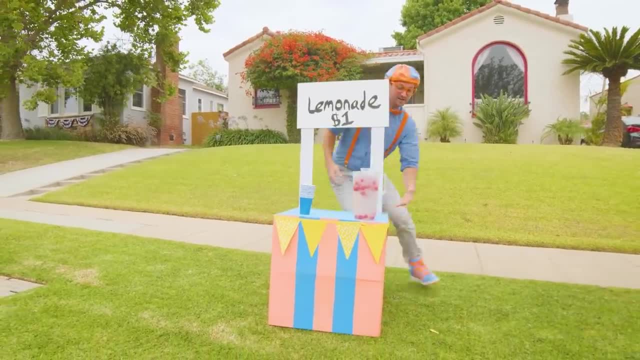 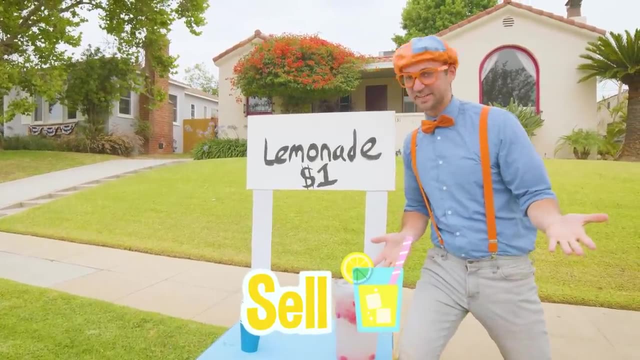 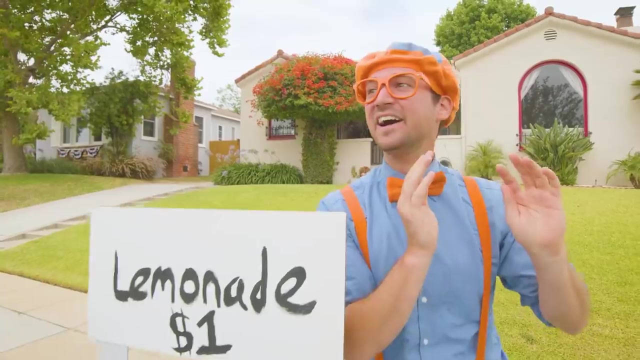 We did it. We built this amazing lemonade stand. We made some tasty lemonade. Yeah, Now it's time to sell some lemonade. Here we go: Lemonade, Lemonade. Who wants some lemonade? I'd love some lemonade. 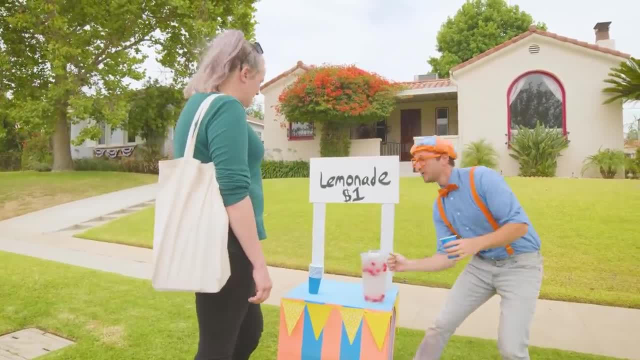 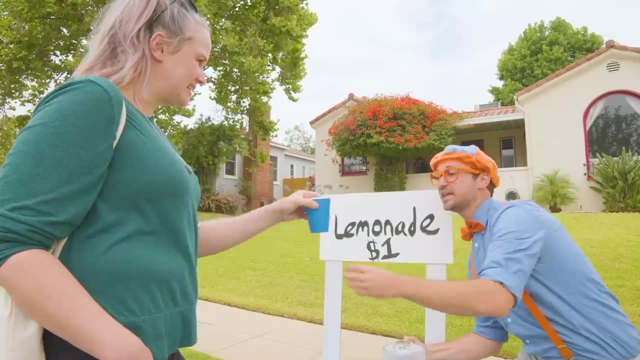 Oh Okay, What are you doing today? Good, I'm a little thirsty, Oh really. Well, it looks like I might have something just for you. Oh fantastic, How much is it? It is $1.. $1.. 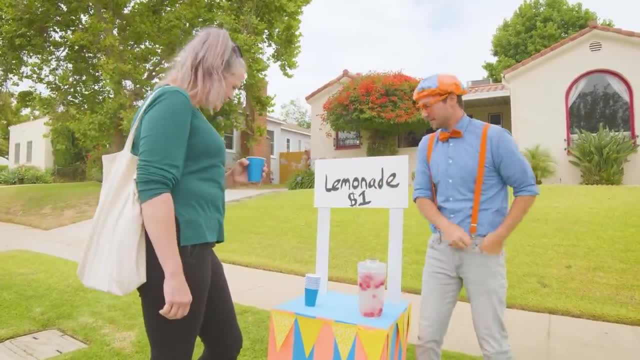 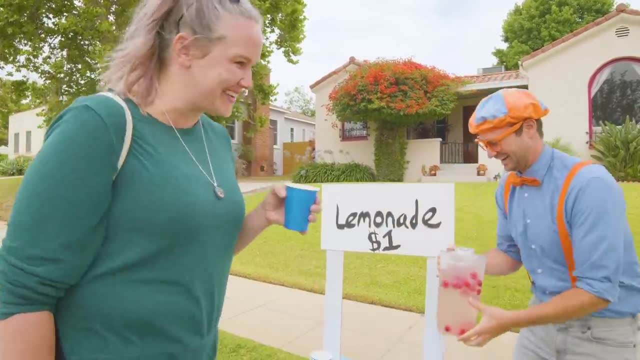 I got that right here, Amazing, Thank you. What kind is this? This is not normal lemonade, It is raspberry lemonade, My favorite. I can't wait to try. Thank you All right, See you later. Bye. 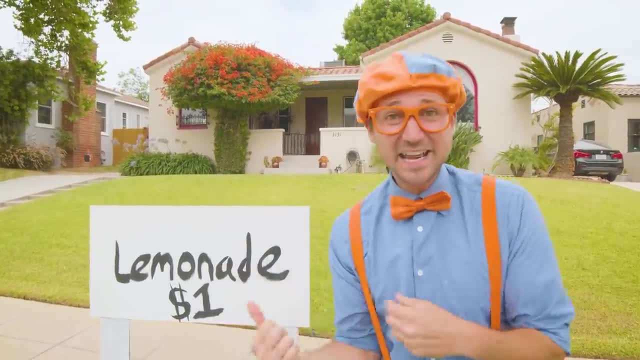 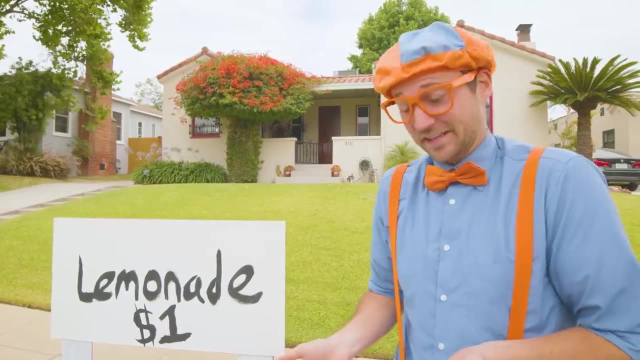 Did you see that You and I just made our very first lemonade sale? Good job. Well, this has been so much fun learning about business, how to make lemonade with you, and having fun along the way. Well, time to sell some more lemonade. 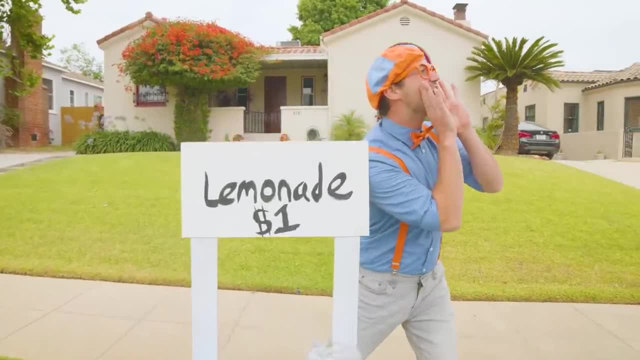 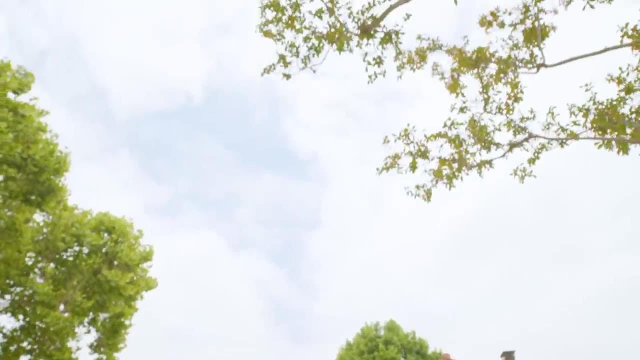 Lemonade, Lemonade. Who wants some lemonade? Yeah, So much to learn about. It'll make you want to shout Blippi. Oh hey, It's me Blippi, And I was just digging. I was just digging. 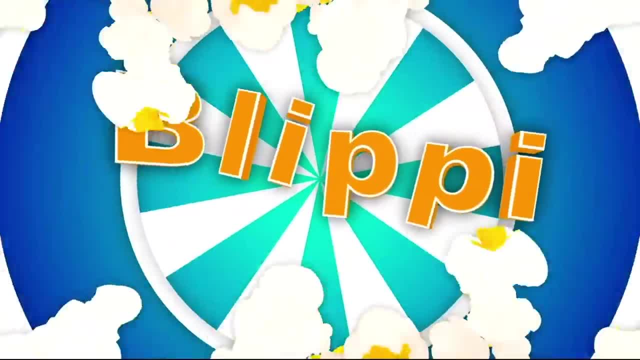 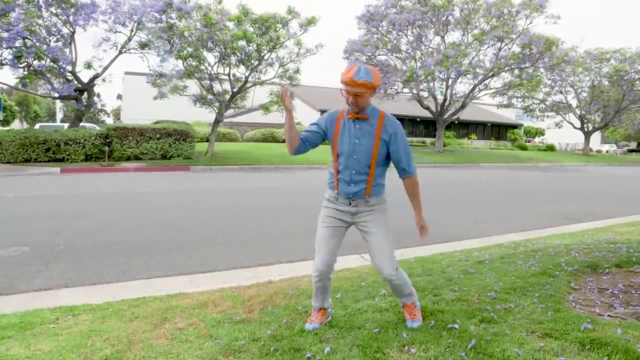 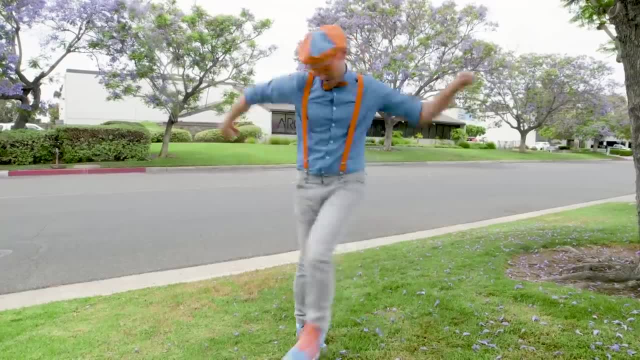 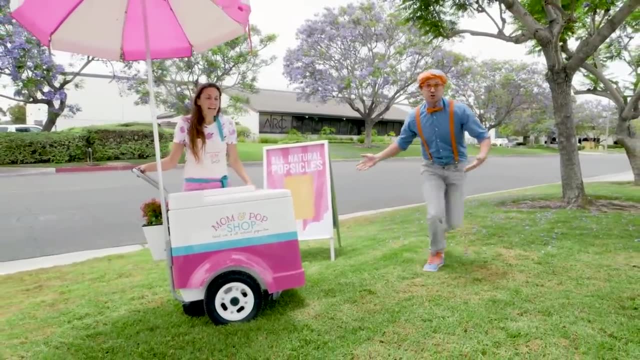 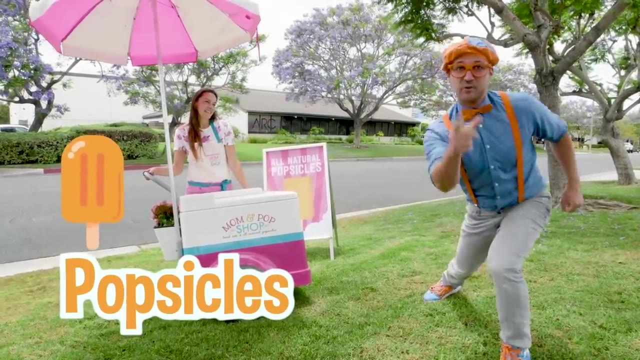 Well, no time for breaks when you're dancing. Do you see that? Whoa, It's a popsicle cart and I love popsicles. I think you and I should get a popsicle. Let's go. Hey Hi, Blippi. 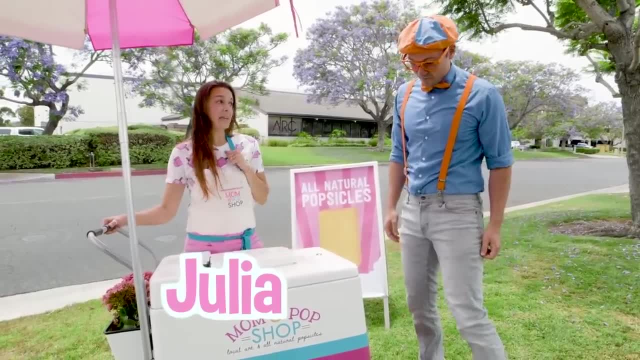 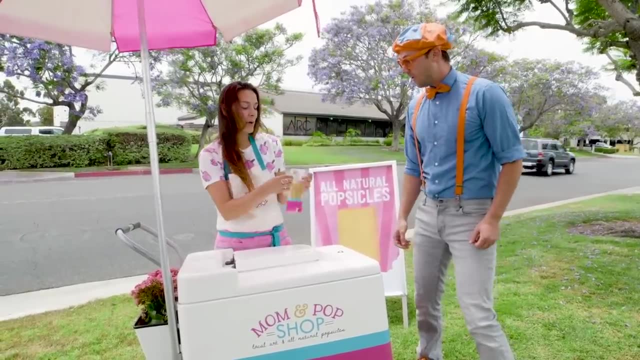 How are you your name? I'm Julia. Would you like a handmade popsicle? Yeah, I love popsicles. What flavor do you have? This is cha-cha-cha. It's mango, pineapple and chia seed. That sounds so yummy. 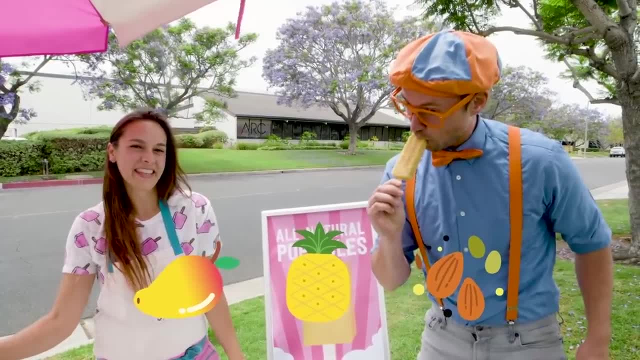 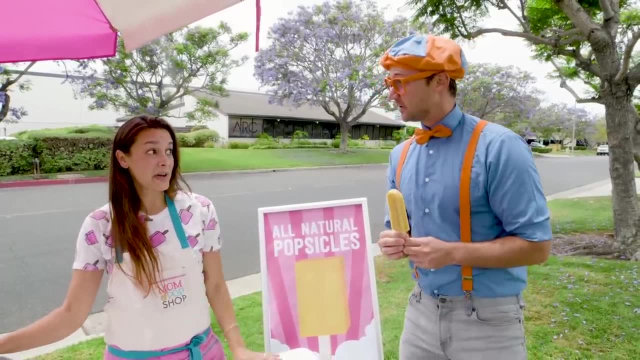 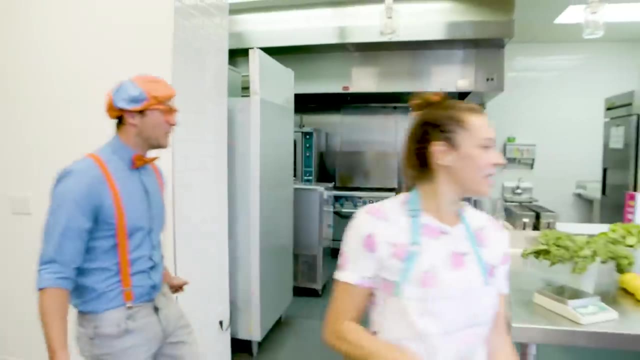 Mango, pineapple and chia seeds. That is so yummy. Yay, glad you like it. Do you want to come see how they're made? Yeah, that would be so much fun. Let's go. Welcome to my kitchen. 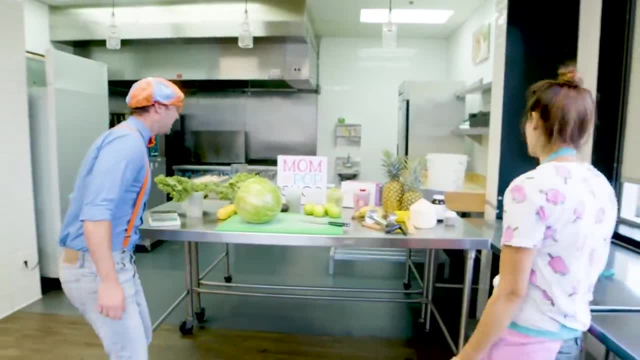 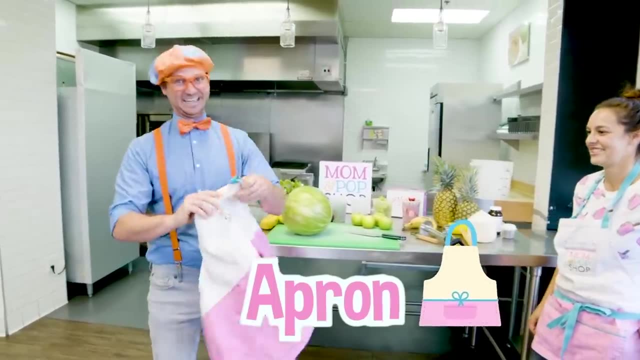 Wow, look at this place, It's so cool. Thanks. Now, first thing, you need to gear up. Check it out. This is an apron. Here we go, Wow, Okay. well, what do we have here? 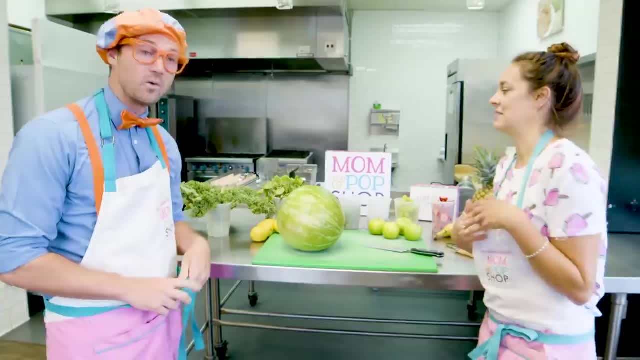 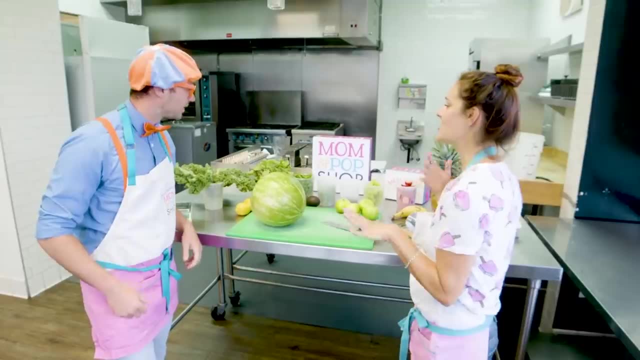 So these are all the ingredients we use to make our popsicles. Oh, it looks like a bunch of fruit and vegetables. Yep, you got it. We actually use a lot of superfoods in our popsicles, So you'll see. 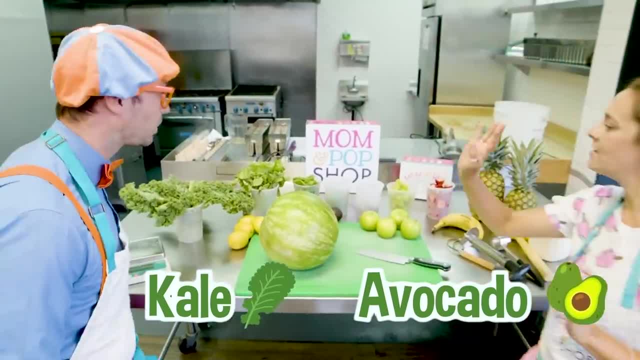 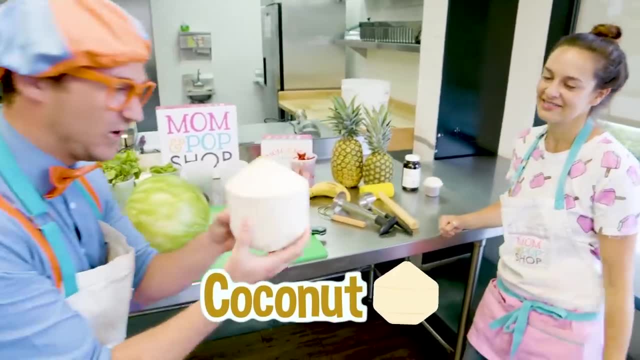 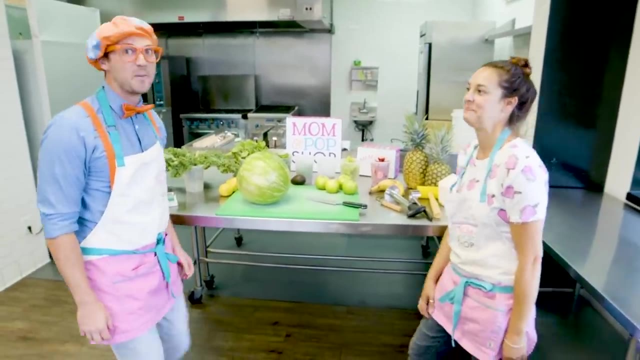 kale and avocado and spinach and chia seeds. What's this? This is a coconut. Wow, that's cool. A coconut Cool. Well, what flavor are we making? I thought we could make Popeye. Popeye, Yeah, All right. Guess why I call it Popeye? Um, I don't know Why. 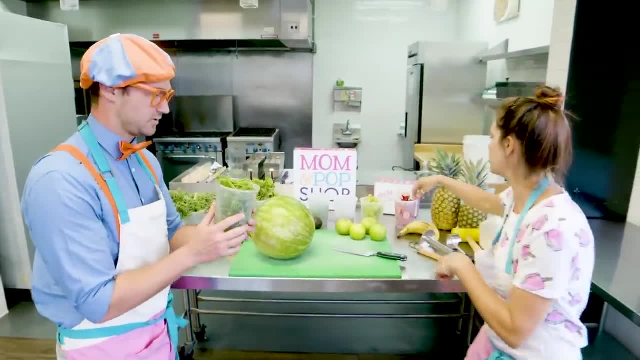 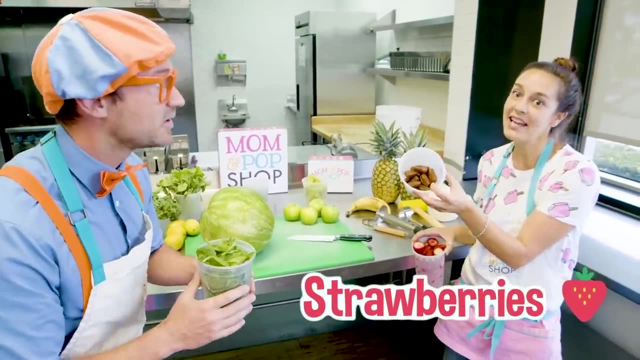 I use spinach. Okay, So here we go. Hold the spinach. I was making a batch earlier, so I thought we could just add to it. Okay, So here's some spinach and what do you have? Strawberries, Strawberries. And to sweeten it, we use dates. Oh, dates, All right, Come on back. 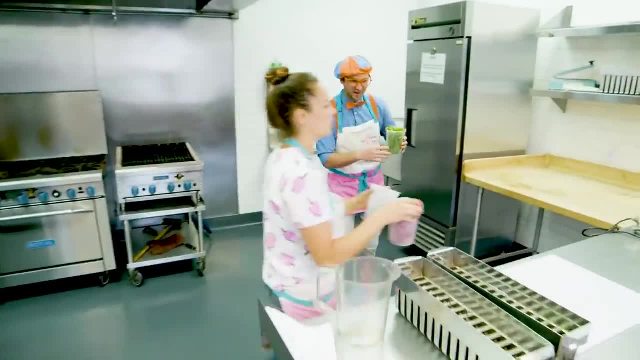 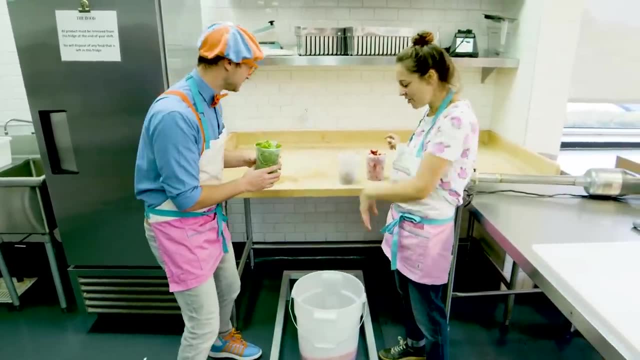 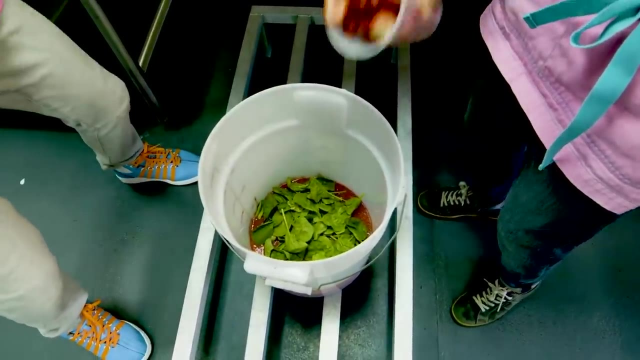 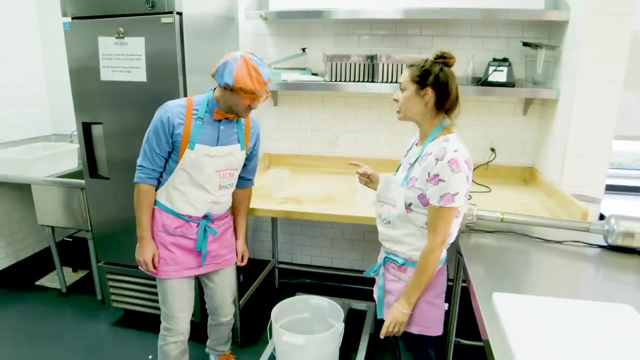 Okay. So here's the batch I was working on earlier. Oh, look at it. All right, That looks yummy. Go ahead, Let's add it in. Okay, Bye-bye spinach. And then here are some strawberries- Ooh, And dates. Yum. Now, what might be different about? 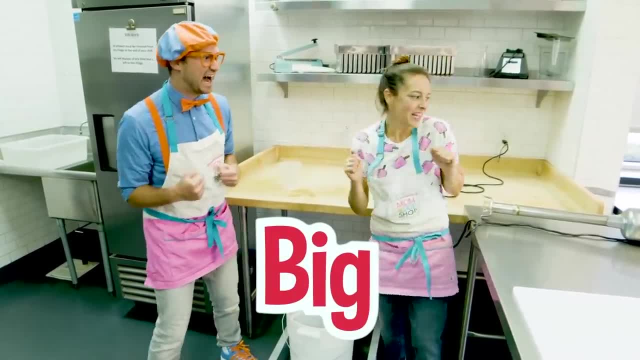 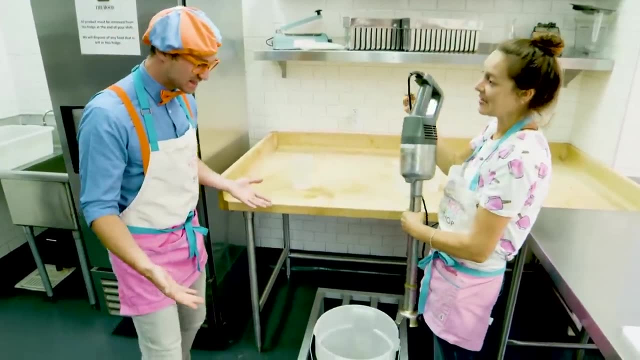 your kitchen is. we have some big equipment we use here. Really, I'm excited. Whoa, look at that. That thing is massive. What does that thing do? This is our immersion blender. Wow, So you put it in. Whoa, You hit the button. 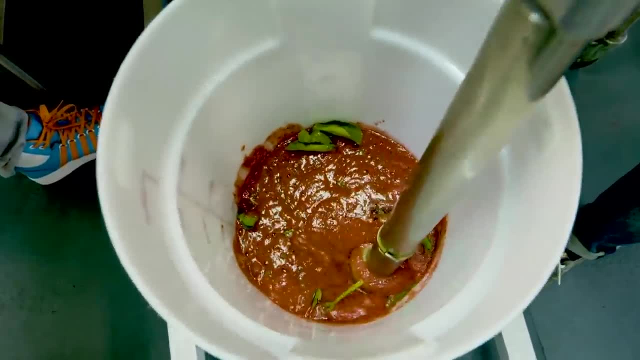 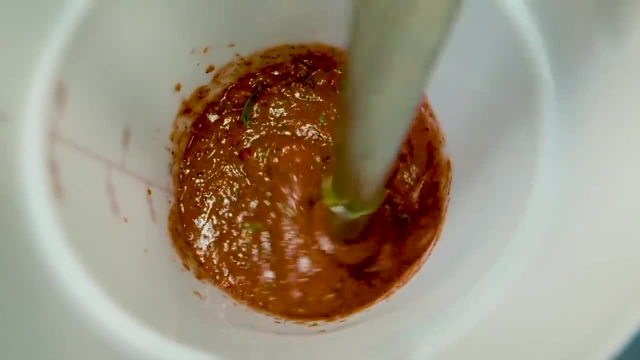 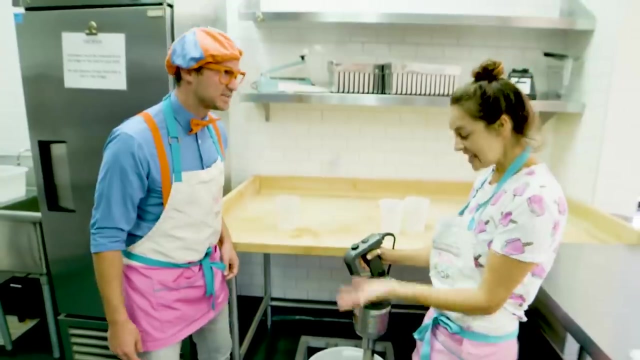 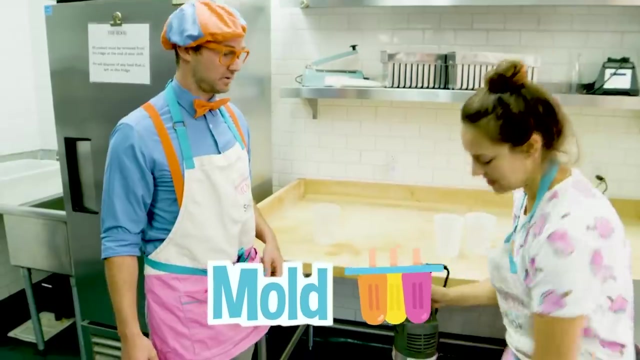 Whoa, Whoa, There you go. So that just blends it up into a liquid. It sure does. Wow, That looks so yummy. Well now, what do we do? Now we're going to put it in our mold, Okay, 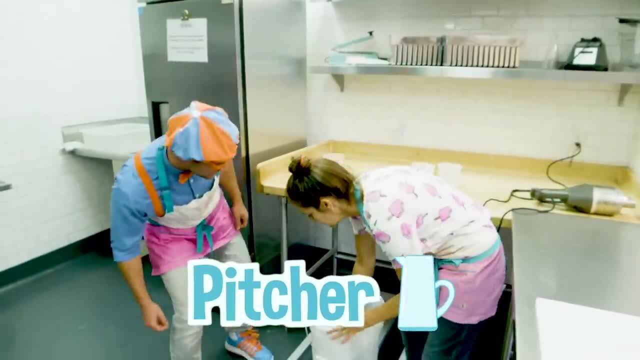 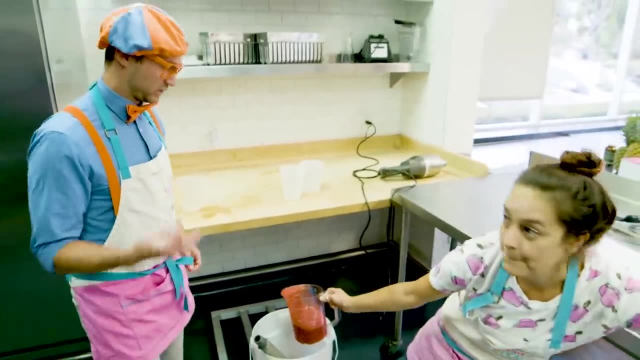 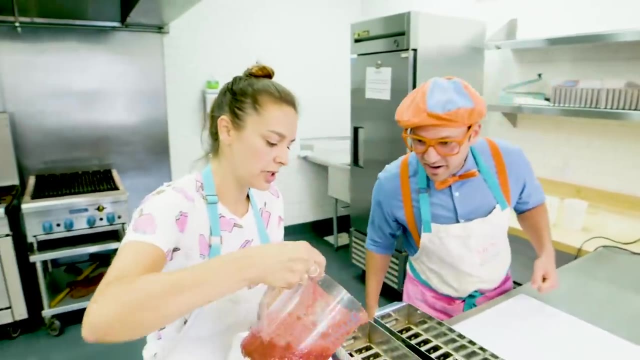 And I'm going to get my trusty pitcher. Ooh, What? So it's basically three ingredients all blended up to make one yummy tasting liquid. So now what we're going to do is we're going to pour it in. 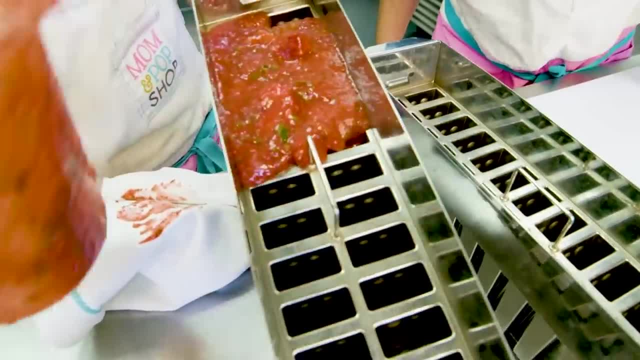 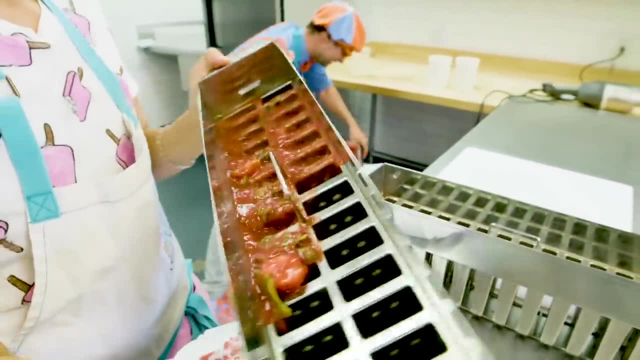 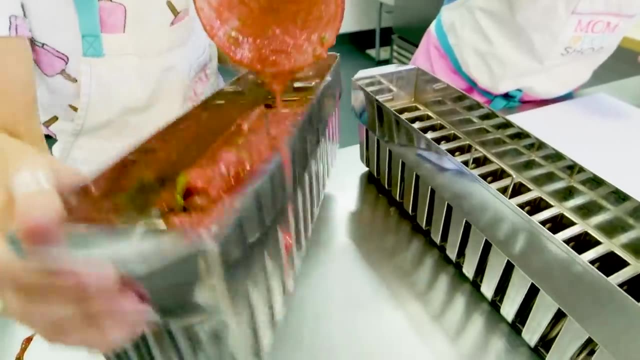 Oh, And then you kind of just have to feed it through, Shake it around. Yeah, May I, Of course. Okay, Here's some more. Whoa, We got some chunky ones in there. That's okay, There's some more. 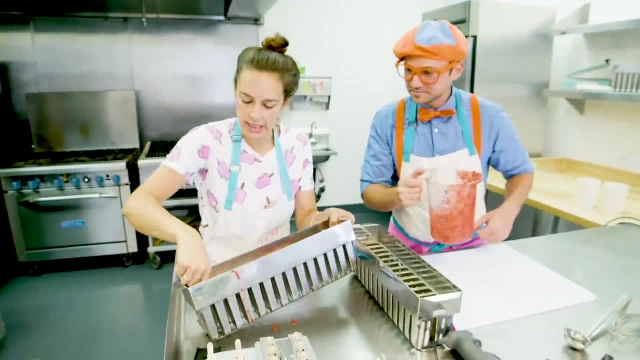 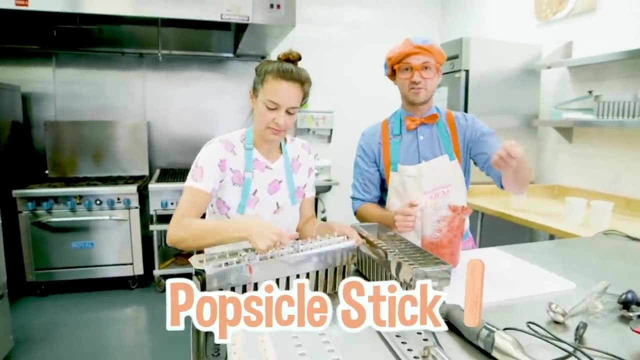 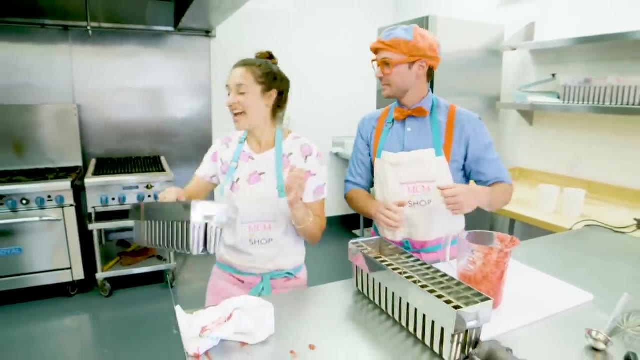 Okay, And then next, what we need to do is: Let's get some more chunky ones out. We'll just put in our sticks, Ooh, Yeah, like a popsicle stick. Have you ever eaten a popsicle and you hold onto the piece of wood? Yeah, That's what we just put in there. That's what makes. 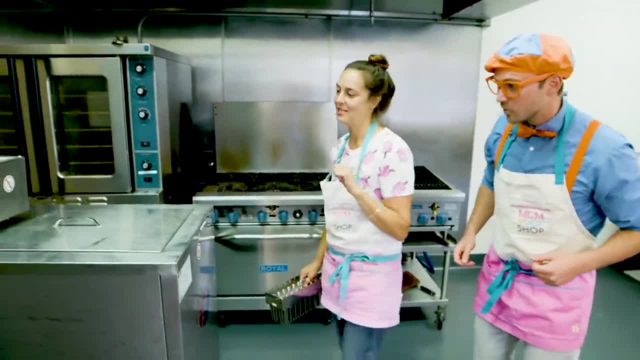 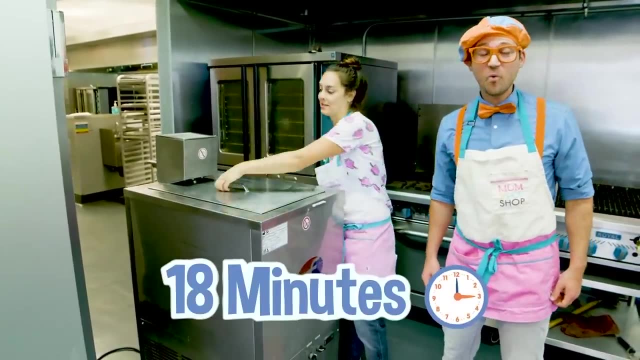 them so handy. Okay, And now we put it into our extra special popsicle machine. Whoa, Whoa. what does this thing do? It makes it super cold. It freezes a Popsicle in 18 minutes. Wow, I'm so excited. 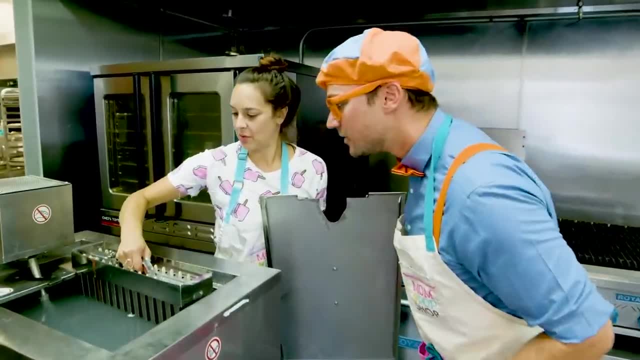 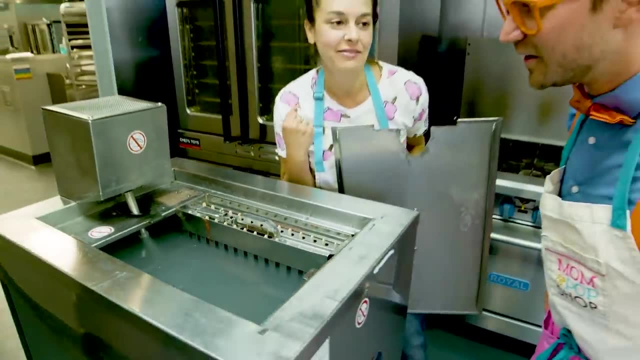 I sure do love Popsicles. Hey, check it out. Let's put it in: Whoa. so is that just really cold in there? Yes, it's actually made out of a special Popsicle freezing liquid. Whoa, all right. 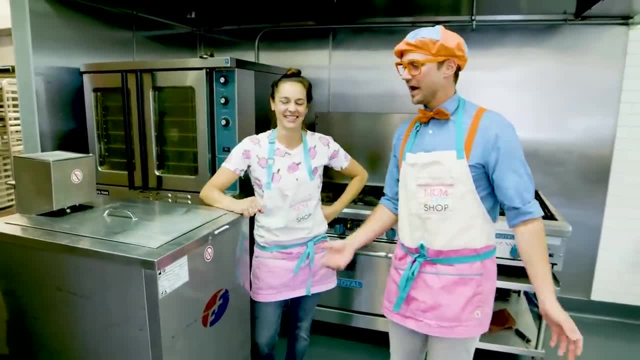 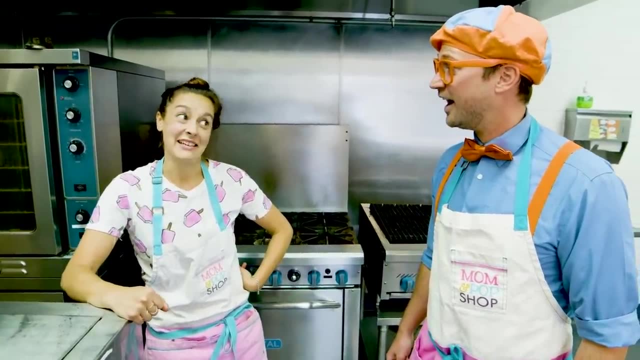 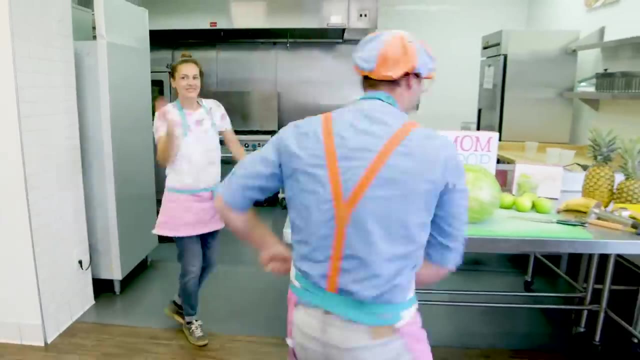 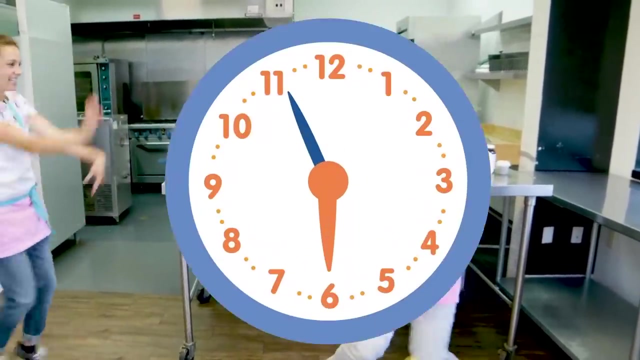 I can't tell you all my secrets, Maybe for later. Well now, what do we do? Well, usually when I wait for Popsicles to freeze, I like to dance. Okay, let's go. Woo-hoo, Whoa. does that mean it's done? 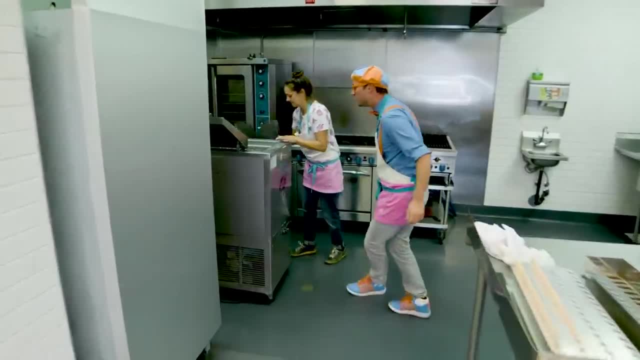 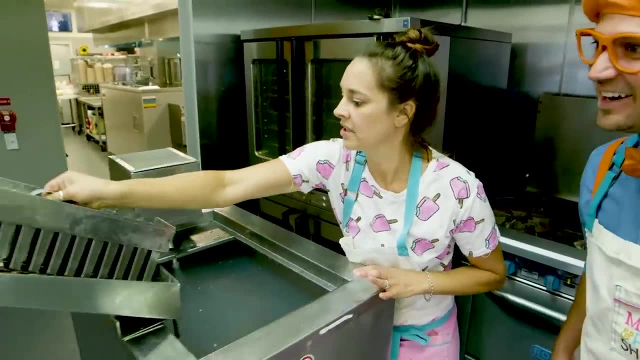 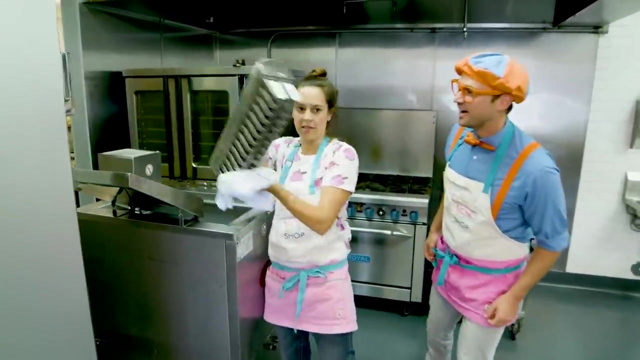 Sure does. Oh, All right, let's shake off that good Popsicle liquid. Okay, Let it dry. All right, I'm going to grab this towel so we don't slip on it. That'll make a fun dance move. 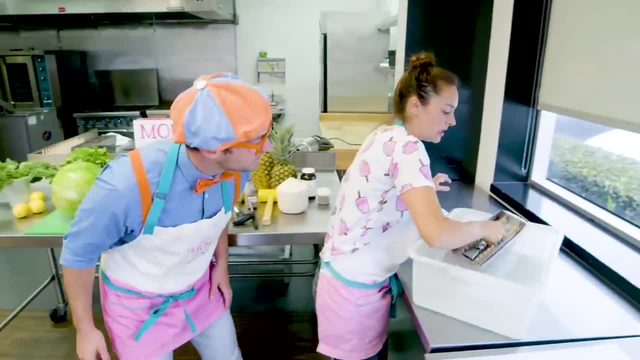 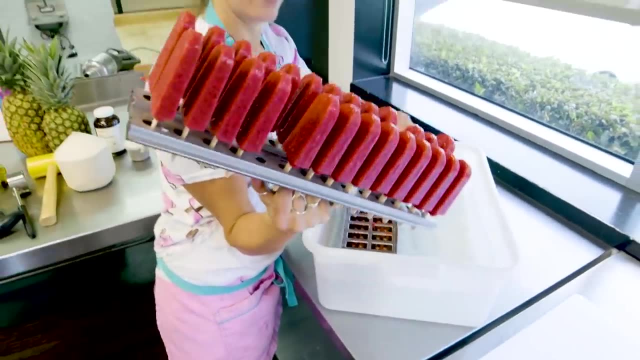 Yeah, We have to put it in the liquid. Okay, and what does that do? It kind of softens it up, so it comes right out. Oh, lost one. There they are. Those look so yummy, I am so excited. 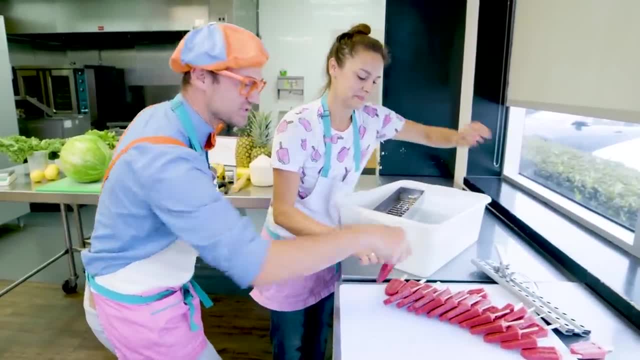 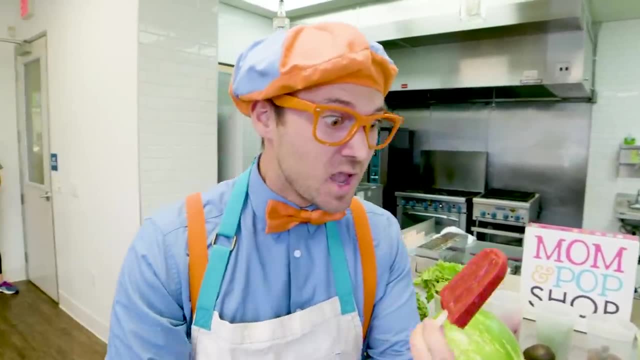 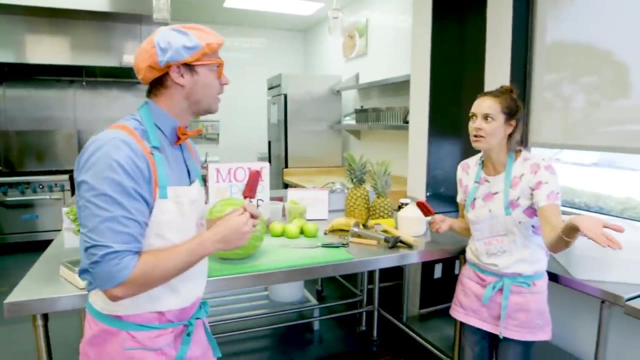 Go ahead, try one. Okay, how about this one? Wow, Yum, That is so yummy Yum. That reminds me I got to go back out and sell more Popsicles, Okay, well, Do you think you could watch the kitchen for me? 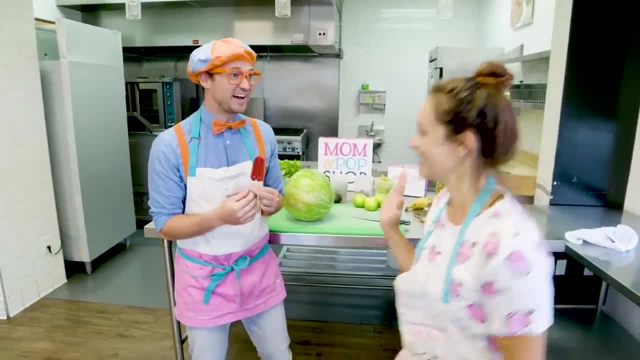 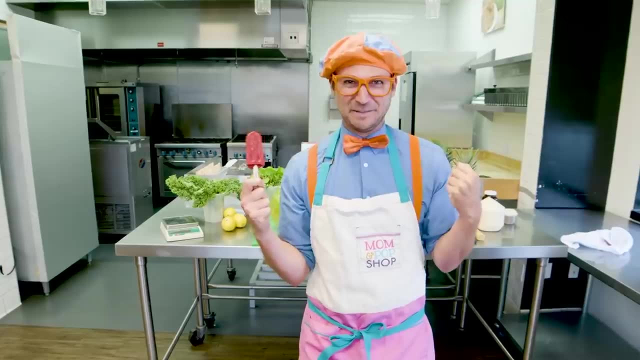 Feel free to make your own flavor. Make our own flavor. That sounds like fun. See you, Blippi. Thanks for showing us around, No problem, Did you hear that You and I are going to make our very own Blippi flavor? 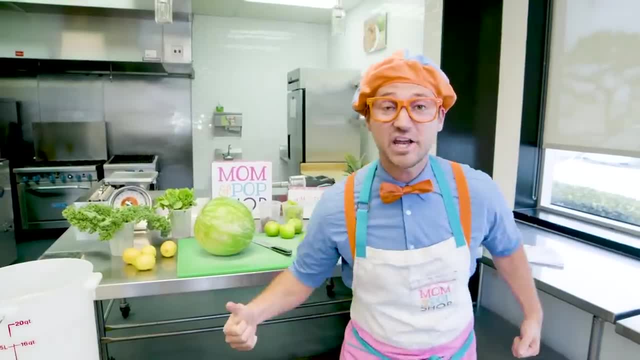 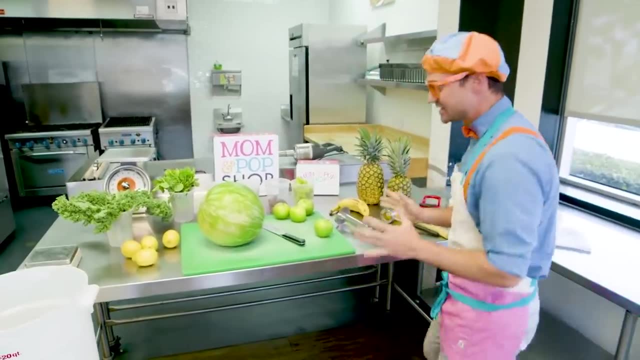 Let's do this. Did you hear that? All right, You and I are going to make our very own flavor, And I am so excited. All right, Let's see what we have to work with. All right, You know what kind of fruit this is right. 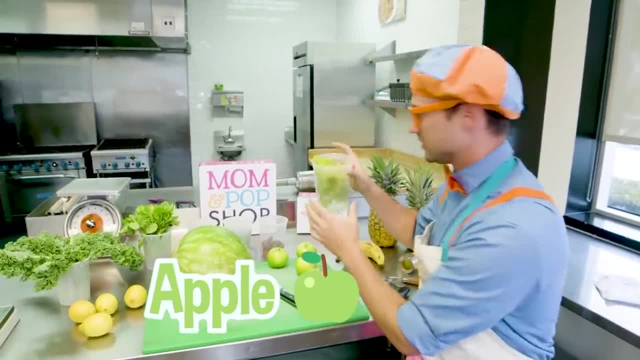 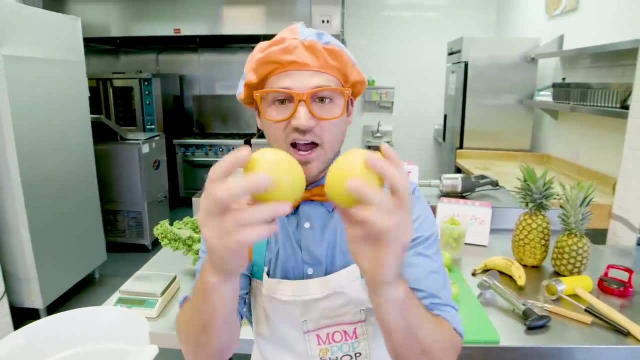 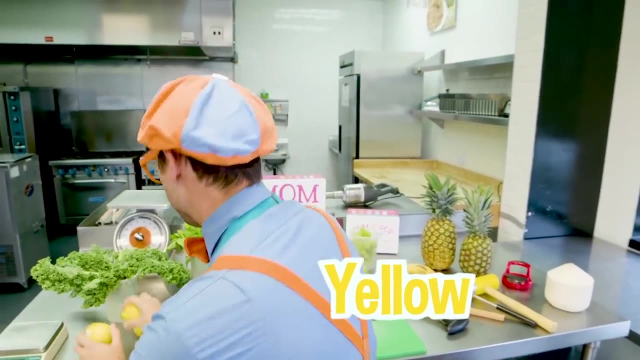 Yeah, This is an apple. Okay, Looks like we have some grapes. Yum, Yum, Ooh. What are these? Check these out. Yeah, These are lemons. Lemons are the color yellow, Wow. And then we have some greens over here. 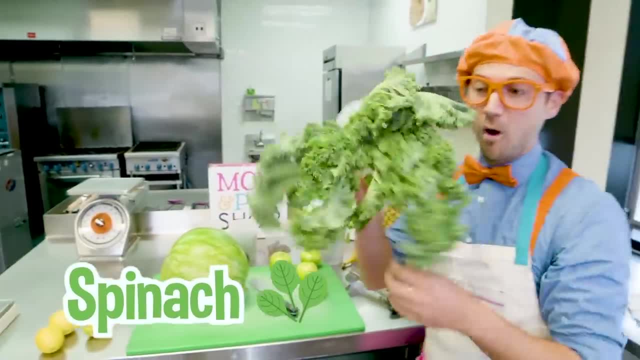 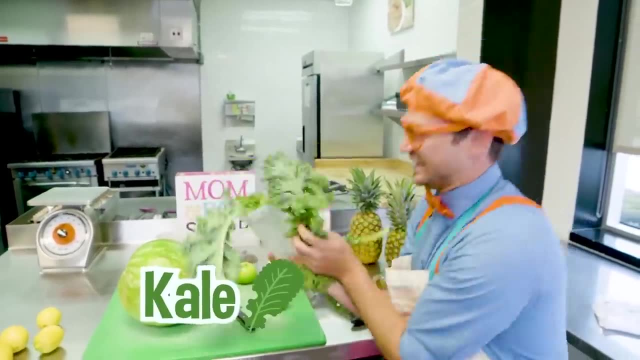 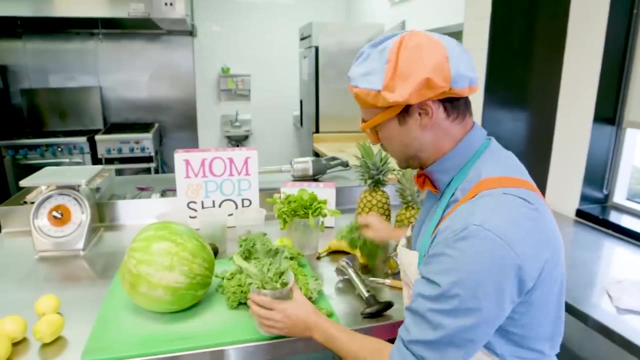 Whoa Spinach, Wow Whoa, Hello, It's like hair. Whoa Oh, This is kale, And kale is really yummy And it doesn't like containers. That's silly. Okay, Let's put these back in here, so then we can continue to see what type of fruits and vegetables. 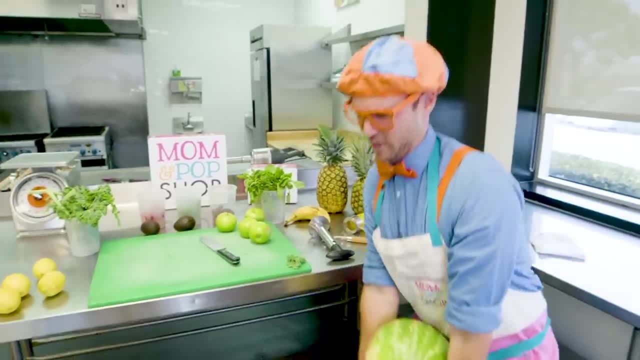 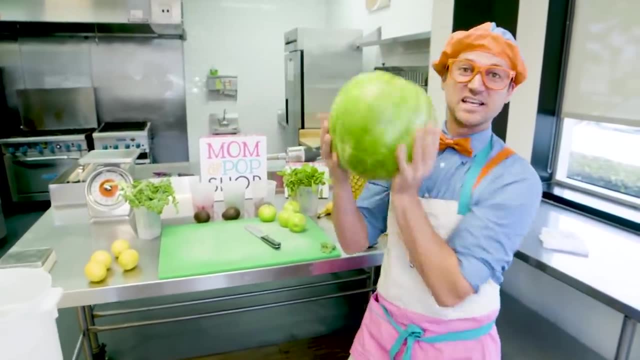 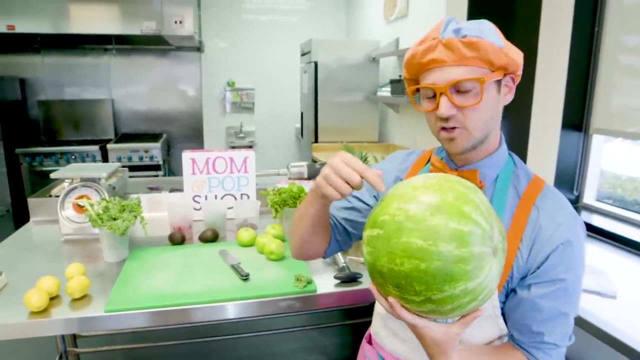 we have like this: Whoa, This is so heavy, Whoa, Whoa. Yeah, This is a watermelon, and watermelons are so big and yummy. Do you know what color is on the inside of the watermelon? Yeah, 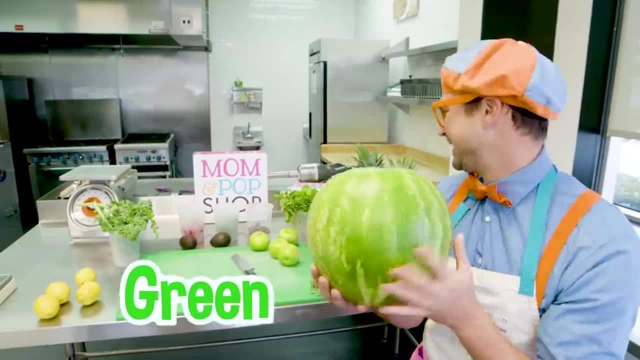 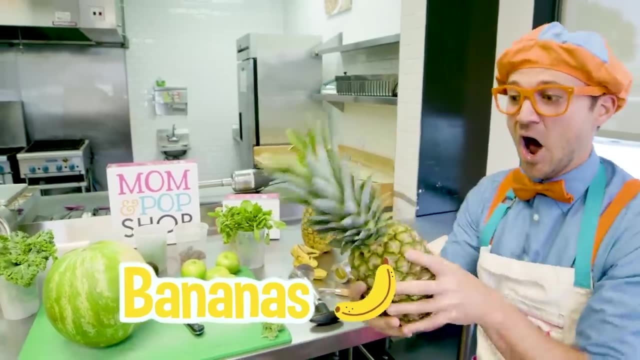 Red, Yeah Red, And the outside is green. Okay, Just a couple more Bananas And pineapple Yum. Okay, So you can see, we have this big bucket right here and we need to put a lot of the ingredients. 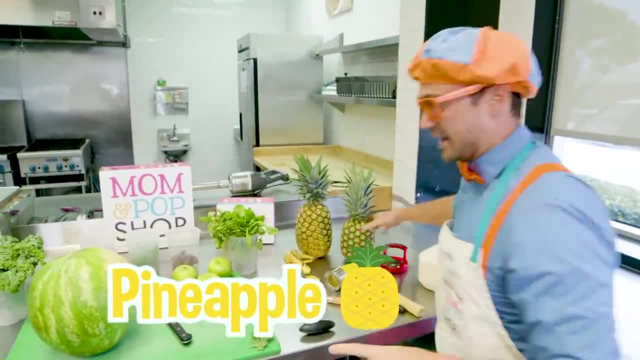 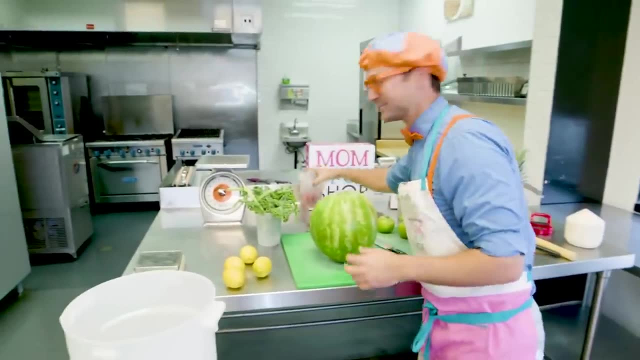 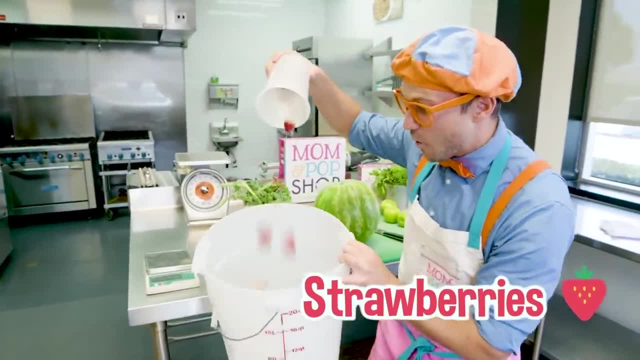 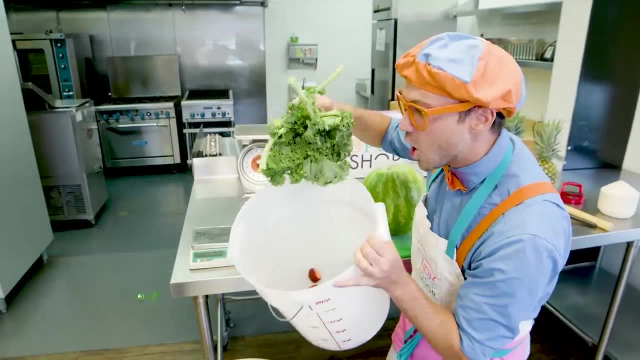 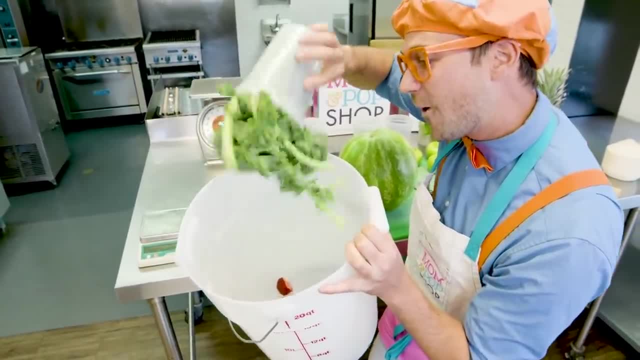 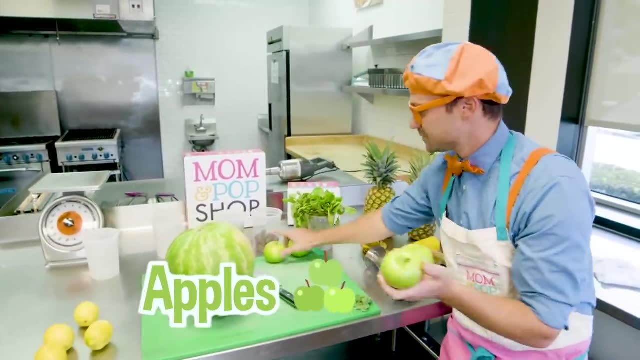 Woohoo, Woohoo, Woohoo, Woohoo, Woohoo, Woohoo, Woohoo. You're doing so good. Oh, Apples- Okay, We could put the whole apple in there, but I think we should probably slice it. 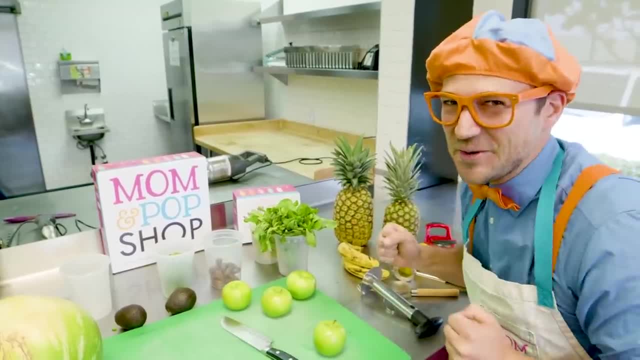 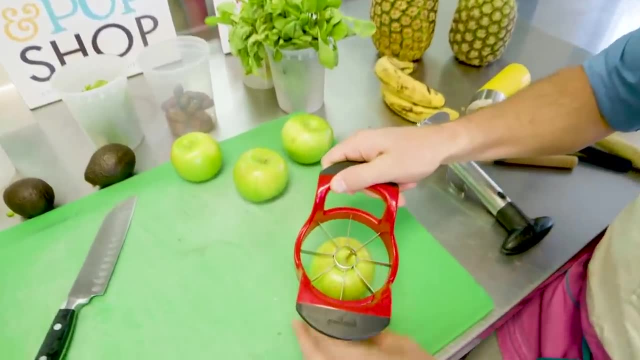 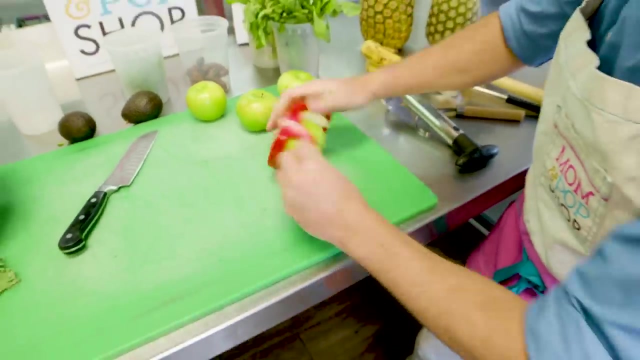 Have you ever had a slice of an apple? They're so yummy. Okay, Here is our red apple slicer. Then put it right in the center, just like that, and then you push down. Whoa, Look at that, That is awesome. 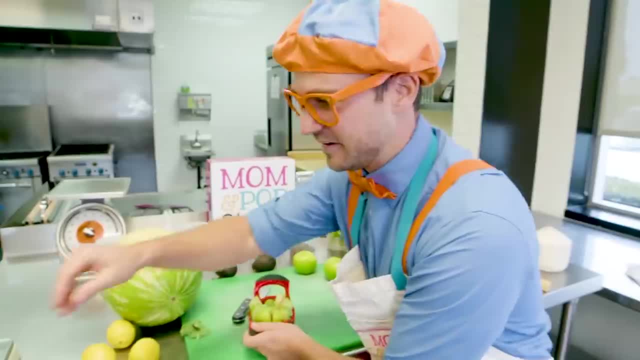 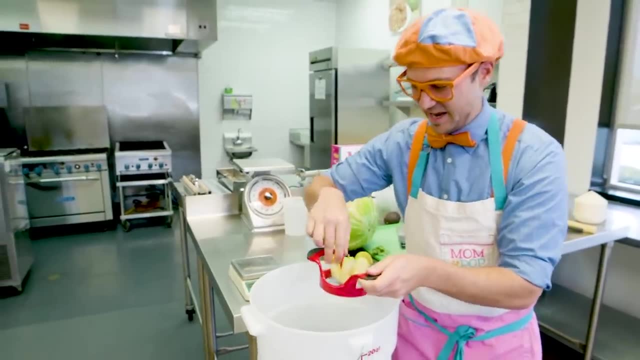 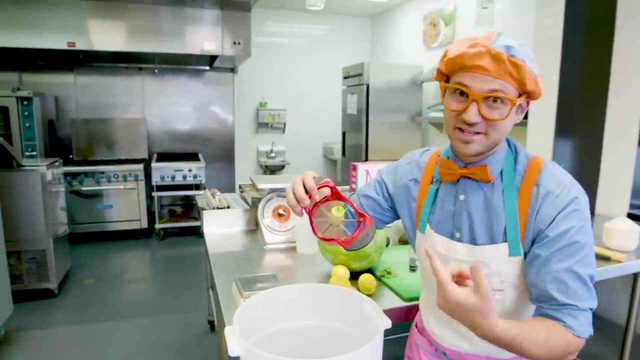 Slice the apples, so then you pull them out and then you can put them right in our big bucket. Wow, And you keep the core. whoop, you keep the core, which is the center out of it, because there's a lot of seeds in there. 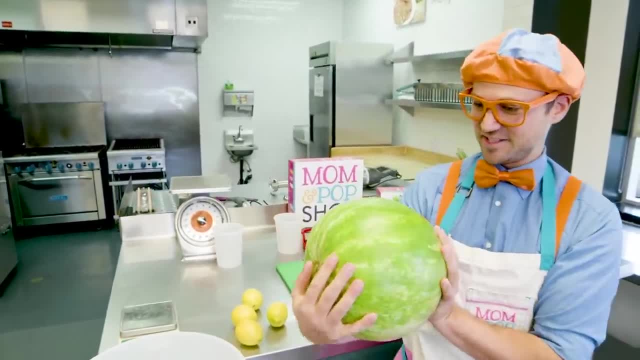 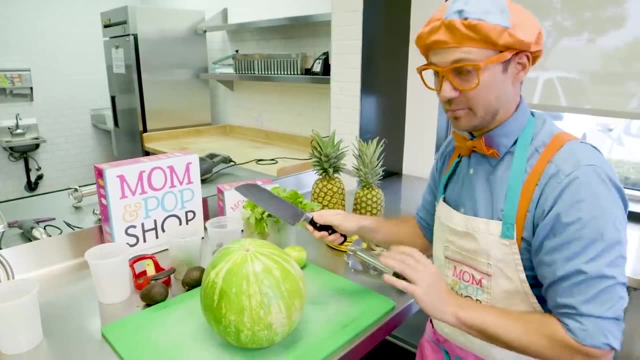 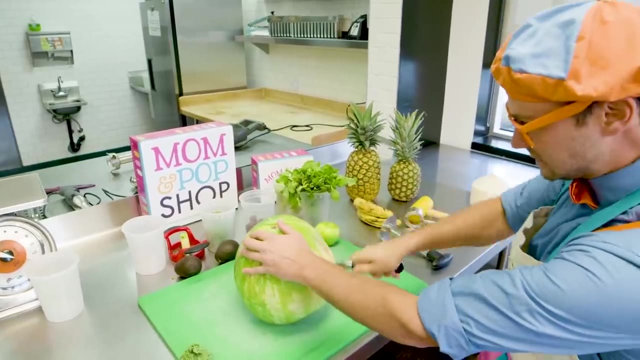 Oh, Speaking of seeds, watermelons have seeds. Okay, Let's cut open the watermelon. Whoa, I'm going to be very careful because I'm a grownup- with this knife Ready. Okay, Here we go. Chop it in half, just like that. 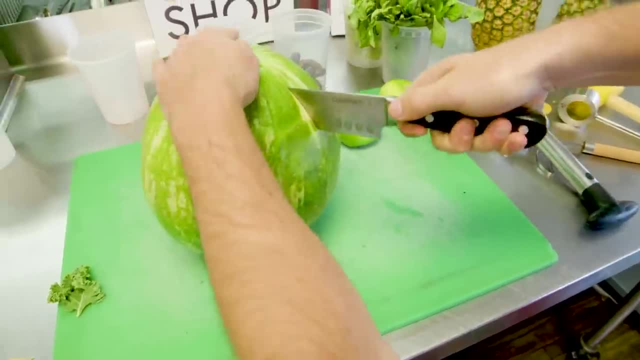 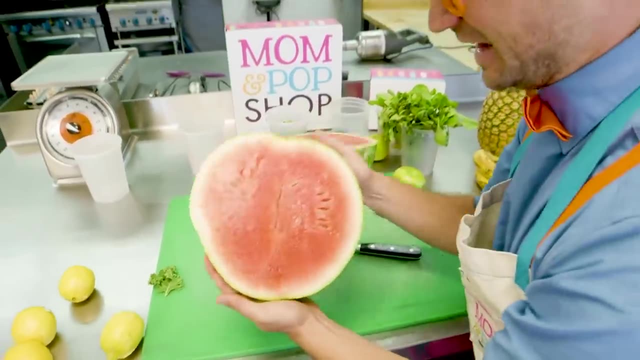 Flip it around. Whoa, Okay, There we go, There we go. Wow, Look at that, That looks so yummy. Our popsicles are going to be so yummy. Okay, I have an idea. Here we go, All right. 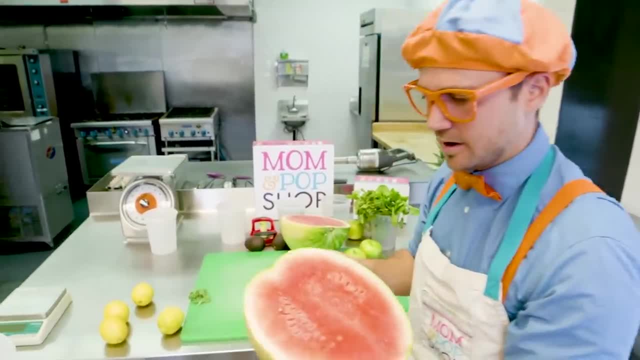 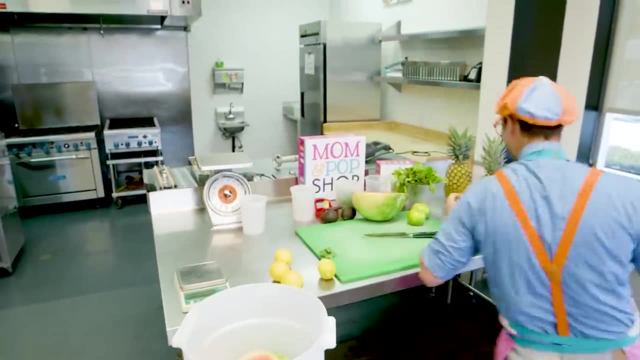 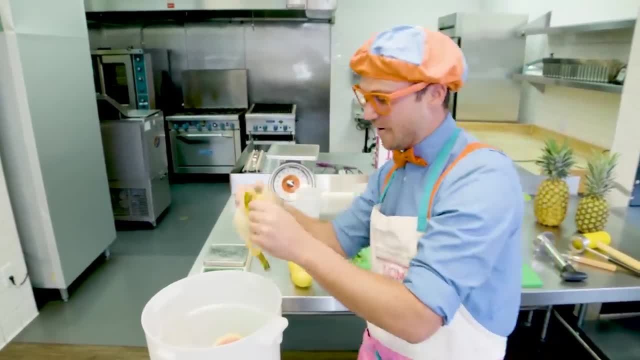 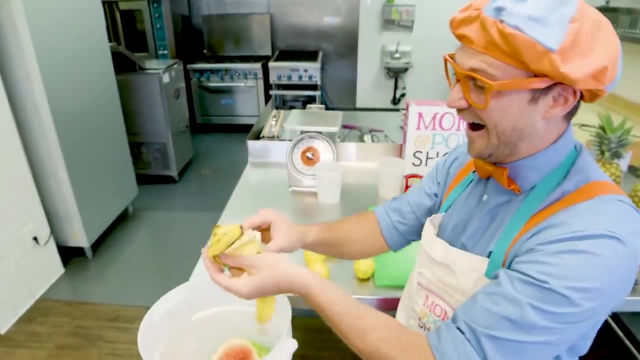 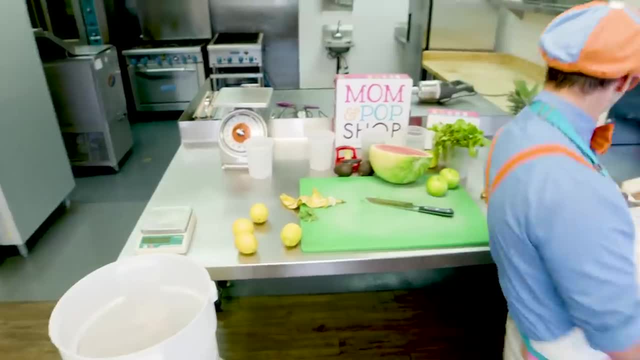 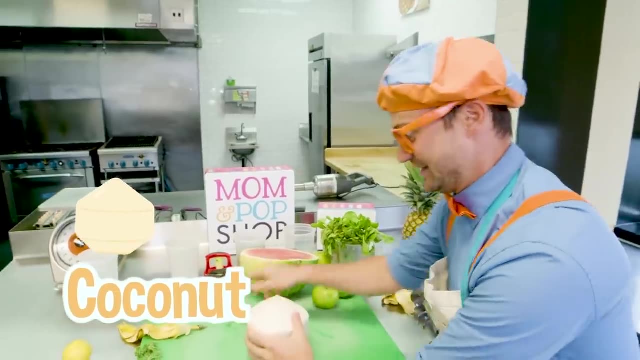 Yum, Look at it. Is that looking tasty? Or does that look tasty? Whoa, And remember we learned what fruit this is? Yeah, the coconut. All right, These are a little tricky to open, but it's worth the trouble, so let's take the coconut. 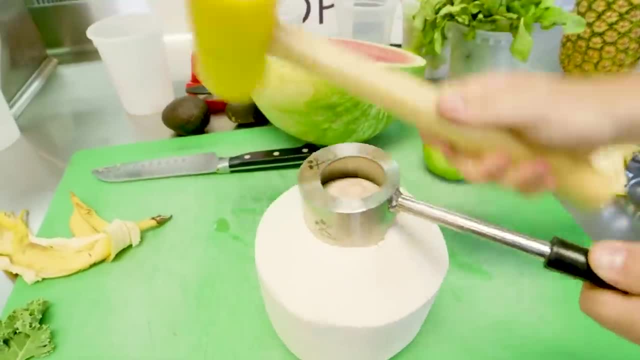 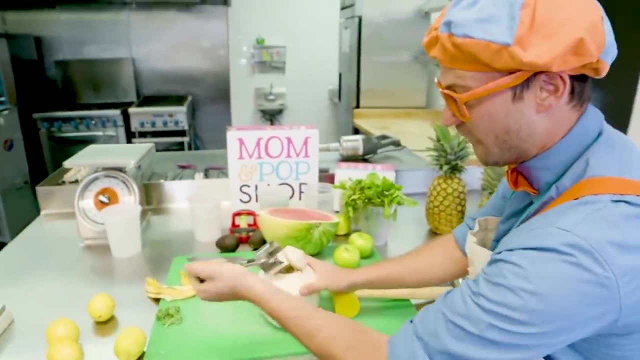 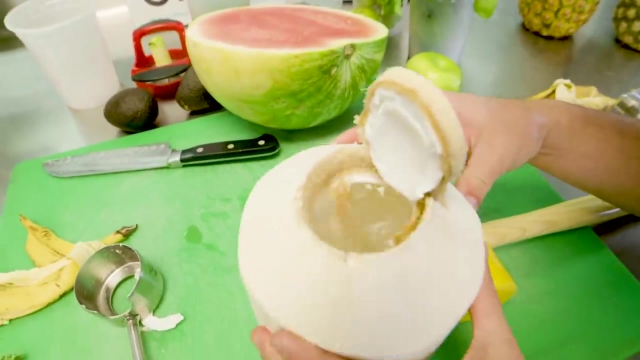 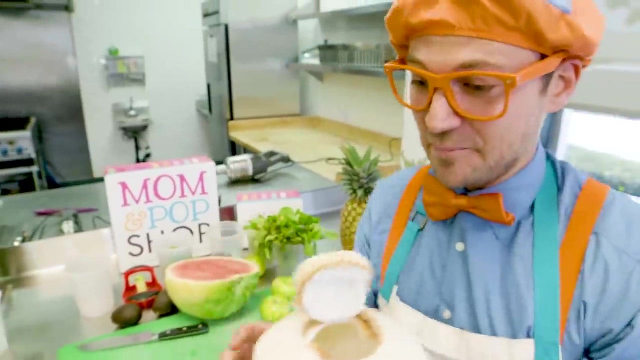 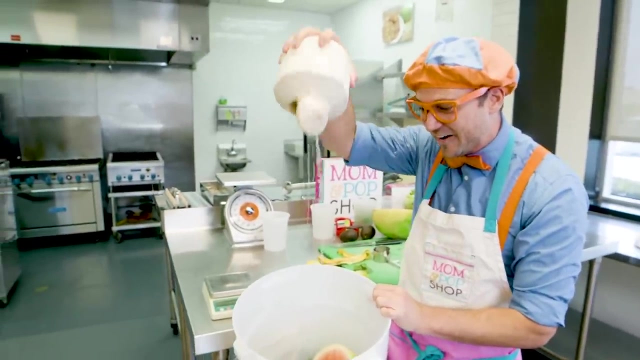 opener. Okay, Wow, we did it. look at that. wow, wow, look at all that liquid. I just want to drink it all up. oh, okay, we'll put that in the bucket for the popsicles. whoa, yum, okay, use this little. 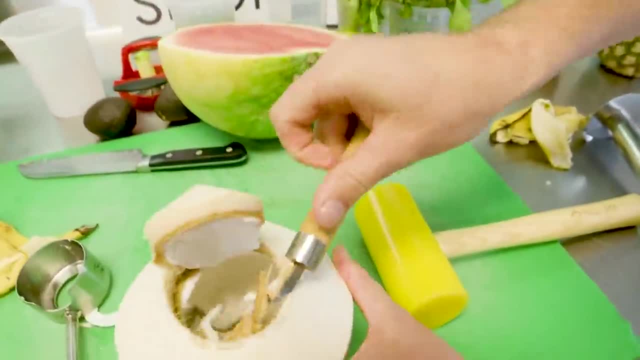 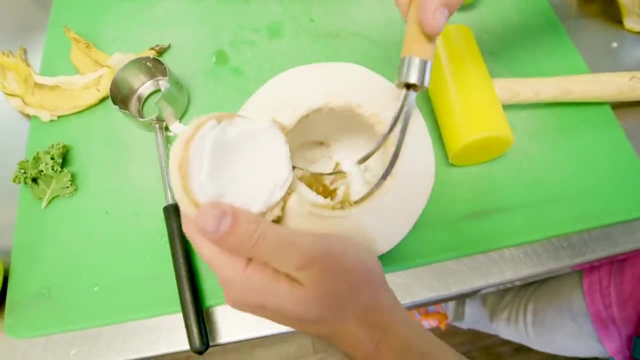 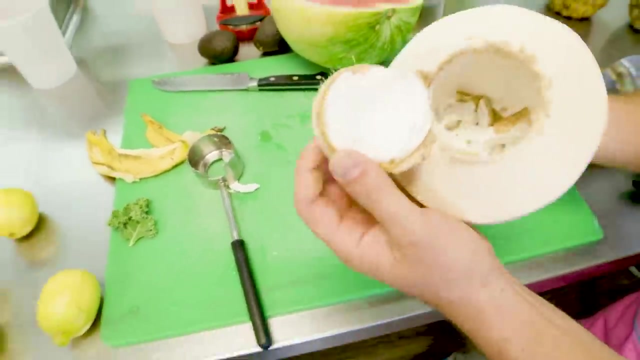 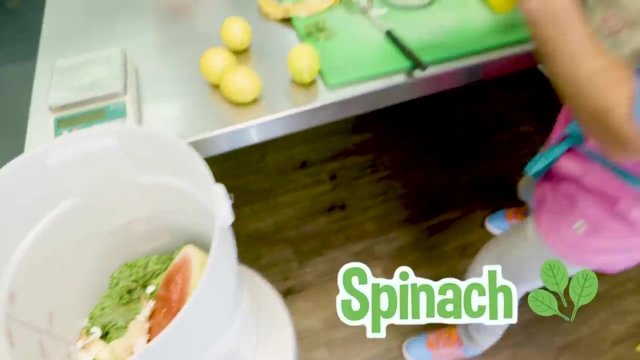 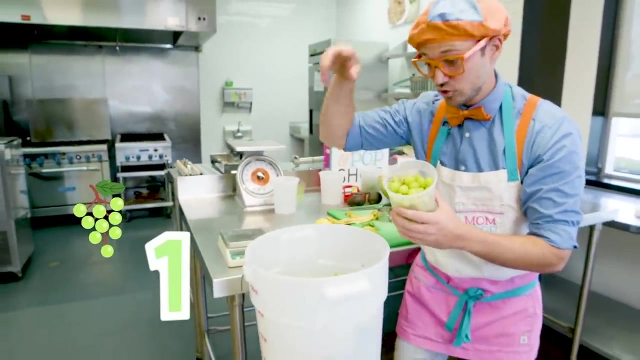 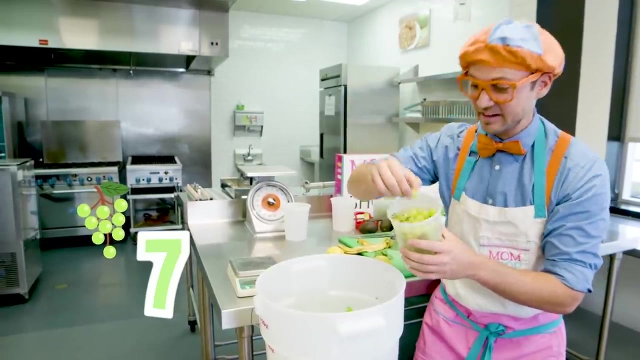 coconut device and pull out some of the coconut meat. yeah, right in there, oh, yummy, there we go. all right, perfect, let's bring it right over here, yum, all right. oh, spinach, right here, woohoo. and then we have a bunch of grapes. we'll do one, two, three, four, five, six, seven, eight. 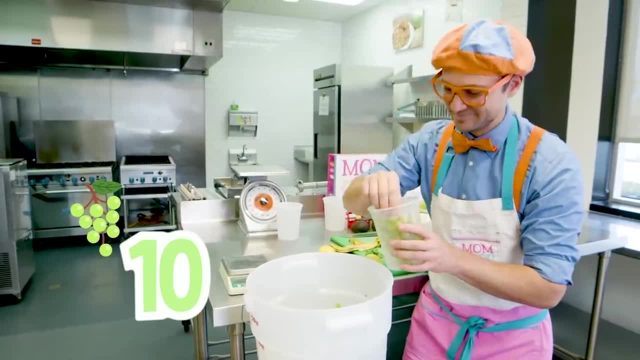 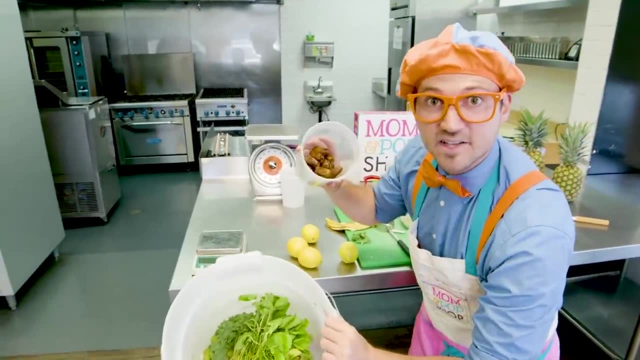 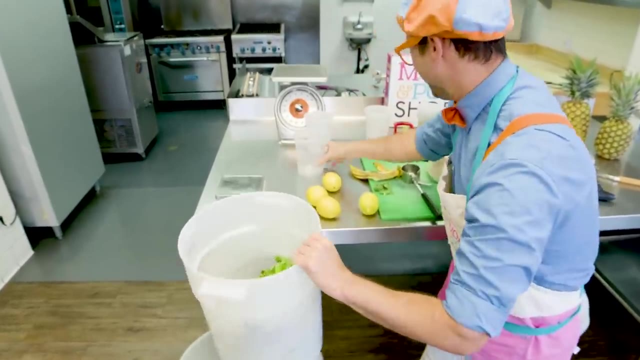 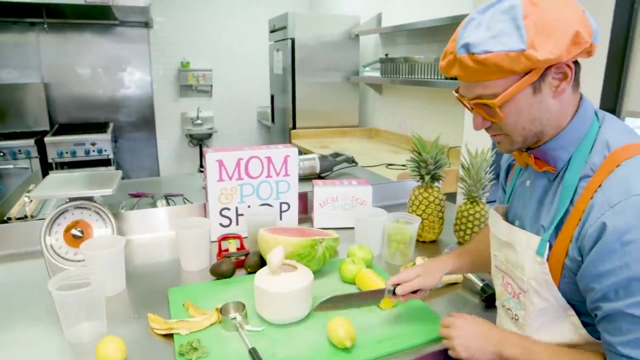 nine, ten, ten, eleven grapes, all right. and then remember these. we used these earlier. these are dates. here we go. whoa, okay, can't forget about the lemons. we have so many types of fruits and 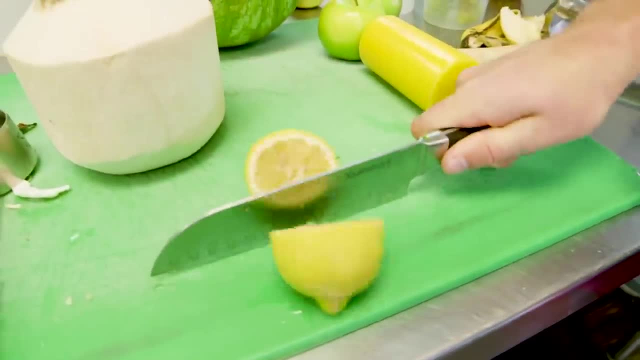 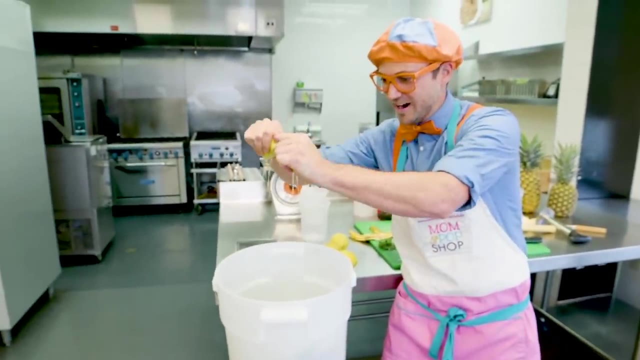 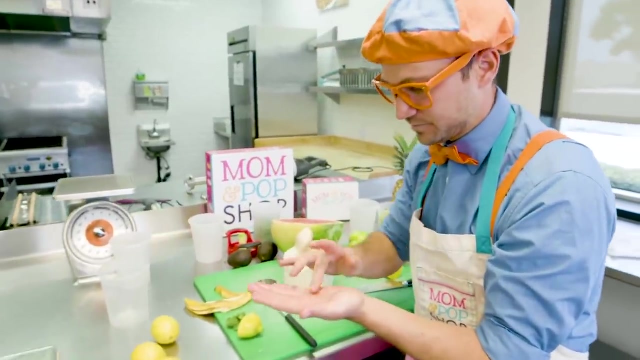 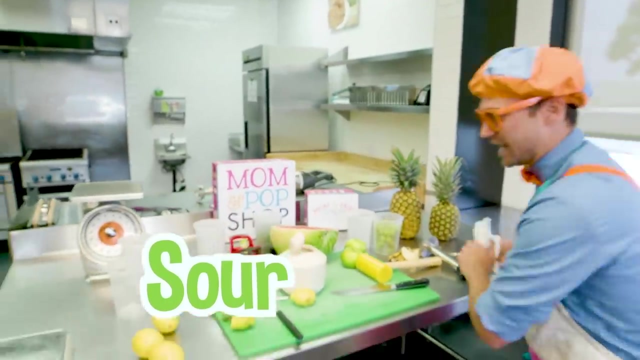 vegetables in here, here we go. wow, okay, let's take these and give a little squeeze. woohoo, have you ever tasted a lemon before? okay, let's try some. whoa, whoa, that's sour. okay, let's wash our hands. and then, last but not least, 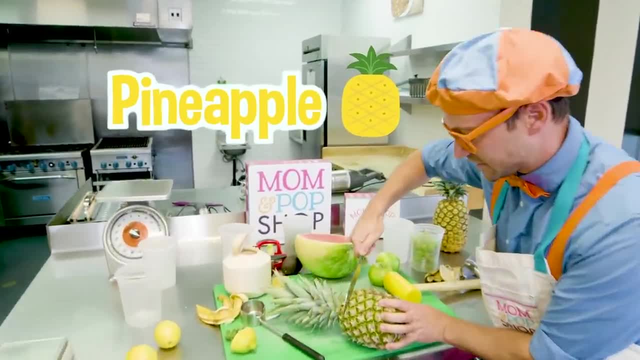 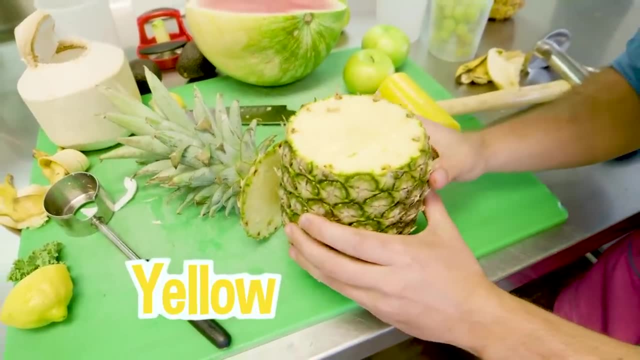 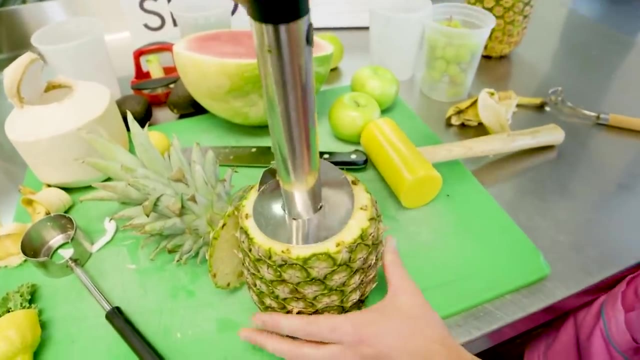 we have a pineapple. we cut the pineapple just like that and see that yellow that looks so yummy. so now admire what just came out of the pineapple. now we take this pineapple tool and put it right on touch and then give it a little twist. 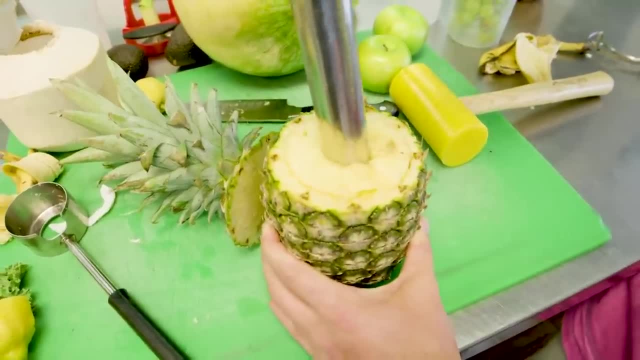 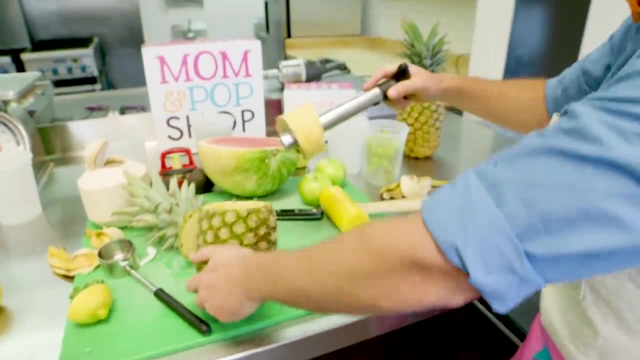 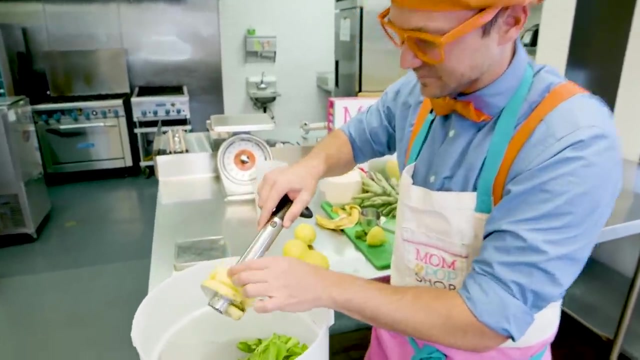 wow, look at that, and then you pull it out- whoa, check that out- and then take it off. just dip that in and then you're done. cool, Awesome, This looks really good, Just like this, and that's gonna give it some nice sweetness. 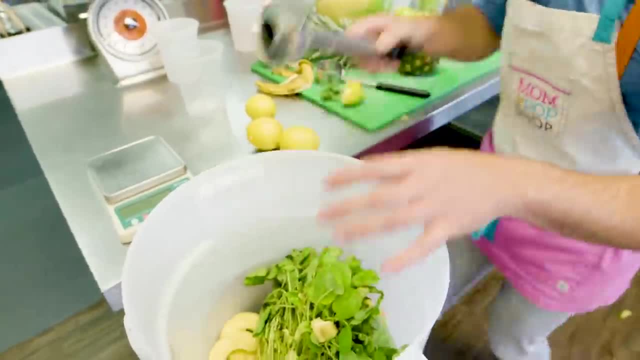 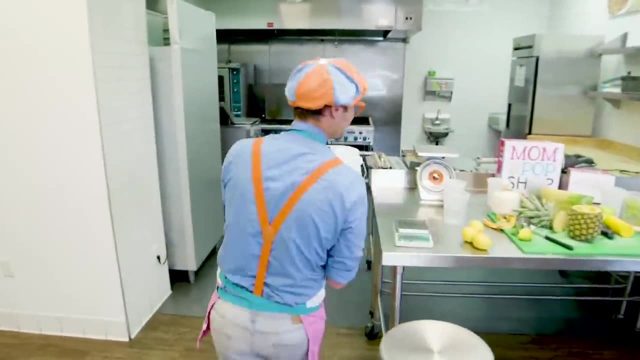 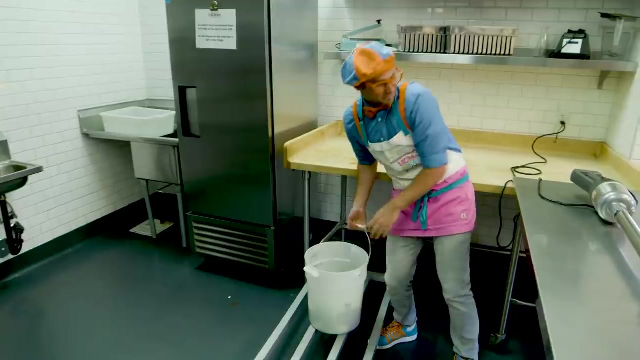 to these yummy popsicles. All right, I think that's plenty. Look at whoa, that's so heavy. Come on back here. Remember that next step that we do. Yeah, she taught us that you put the bucket right here. 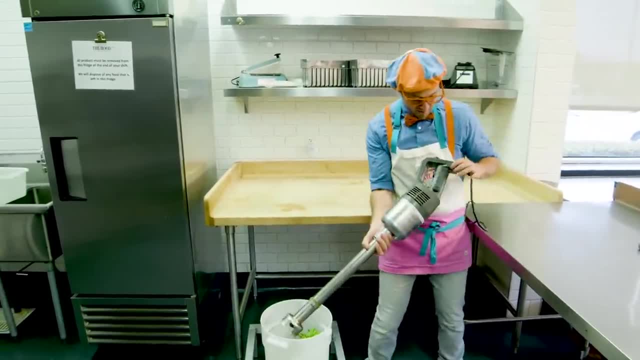 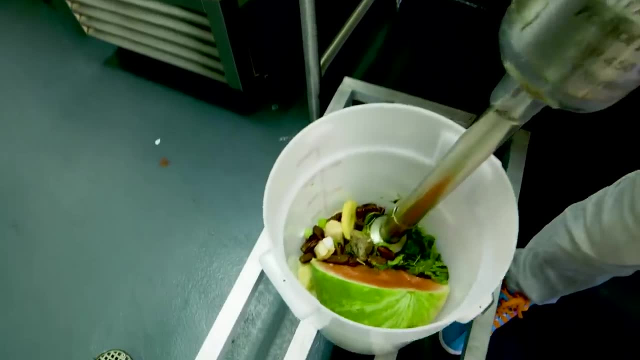 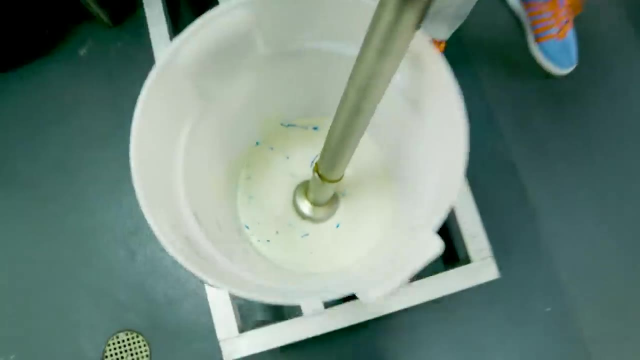 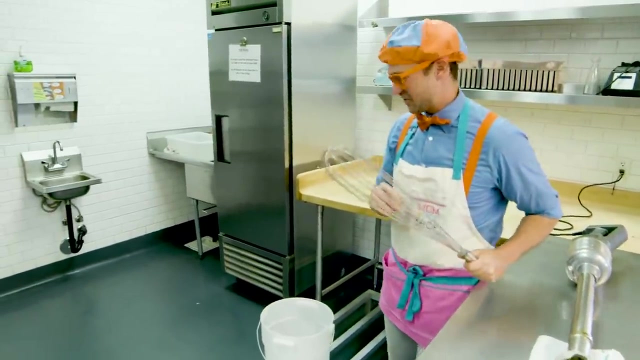 and take the big blender: whoa, Whoa, and we blend it up. Here we go. Whoa, All right, now it's all mixed up. Wait a second, though. we need the magic tool. This is a giant whisk, woohoo. 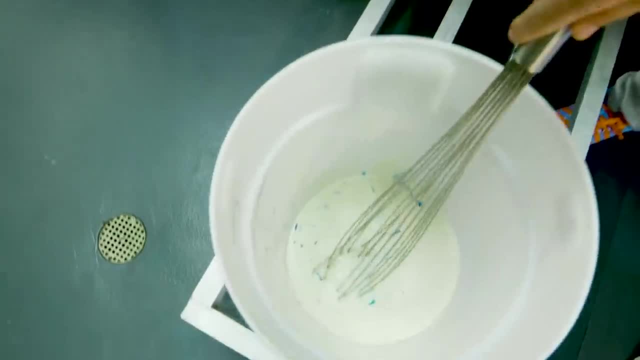 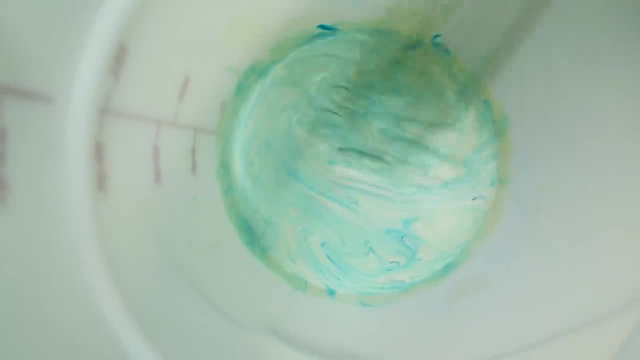 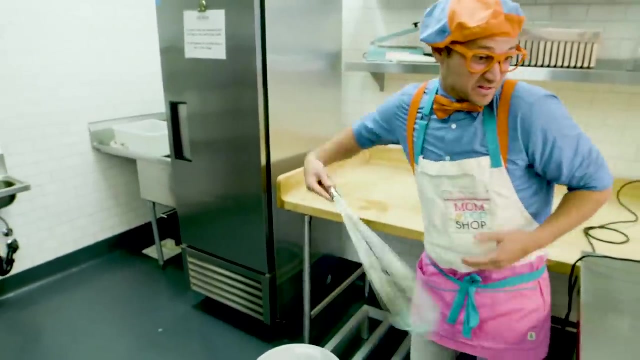 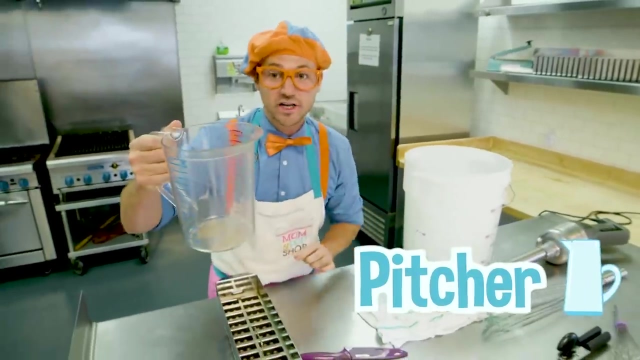 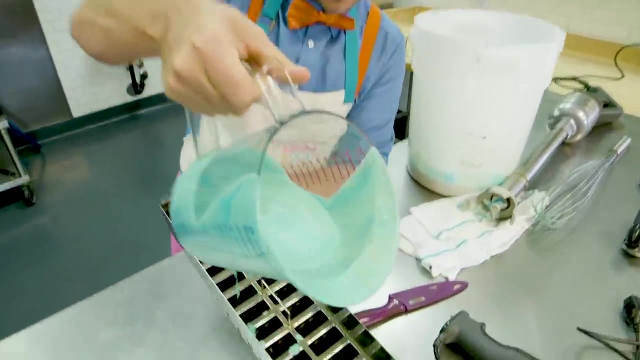 Check this out. All righty, it's adding some color. Okay, let's put this right over here and then we can bring this up and grab this pitcher. Remember from earlier: we need to scoop some out. Oh, I am so excited pour some in. 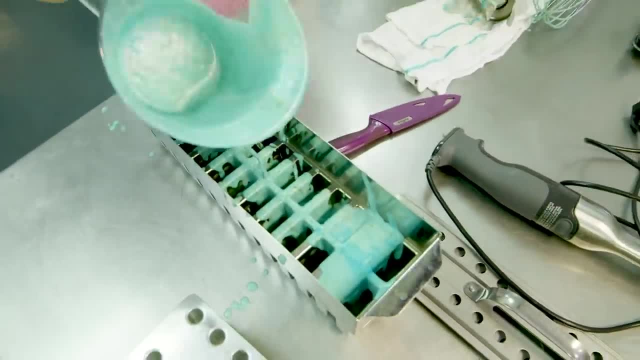 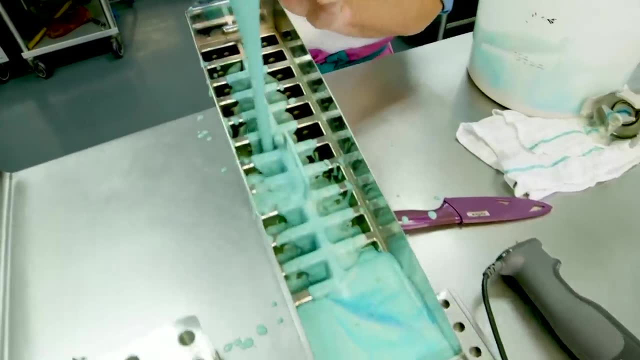 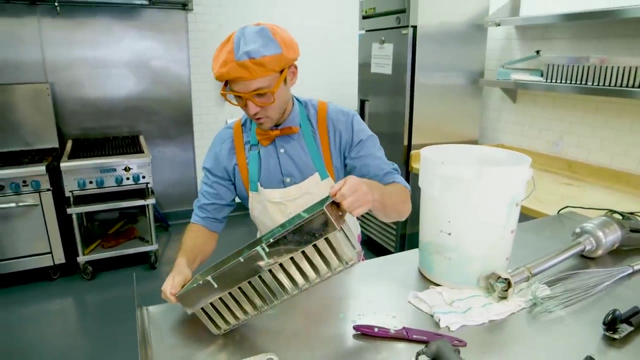 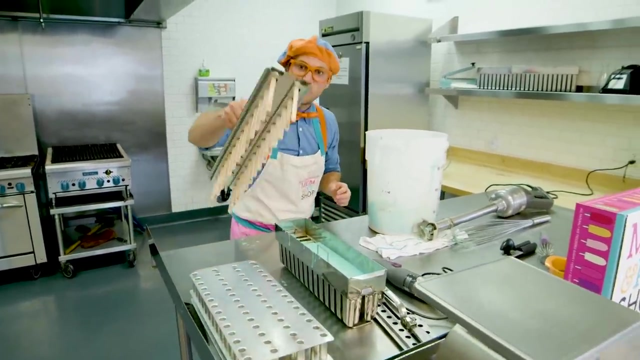 Let's grab another scoop. Okay, here we go. okay, whoa, All right, I think that's plenty, So let's give it a shake. okay, yes, These are gonna be so yummy. Then let's take these sticks, wow. 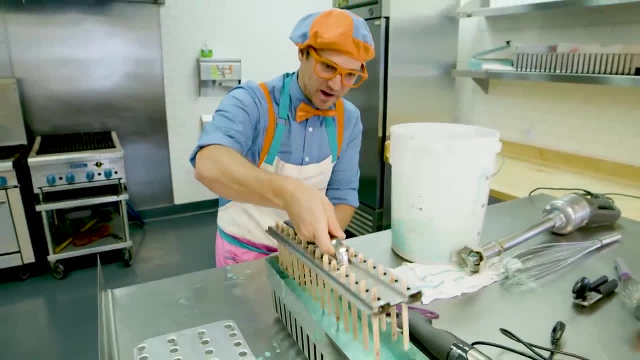 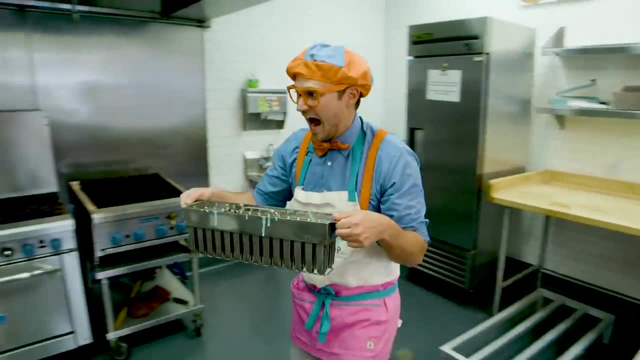 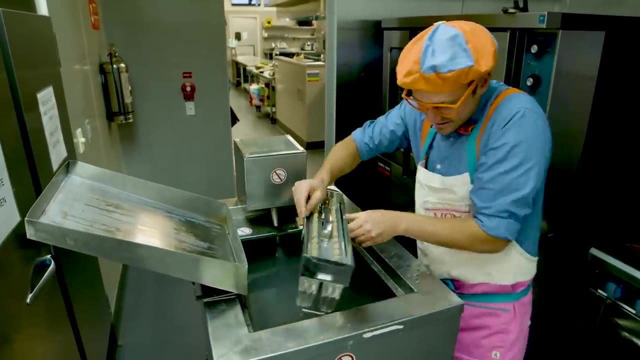 That's a lot of popsicle sticks, Ha ha, Put them right in there. oh perfect, Okay, now we need to bring it to the cooling station. Here we go, set it down. Woohoo, we did it. 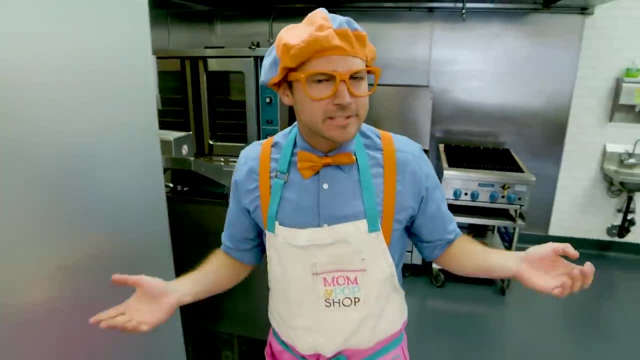 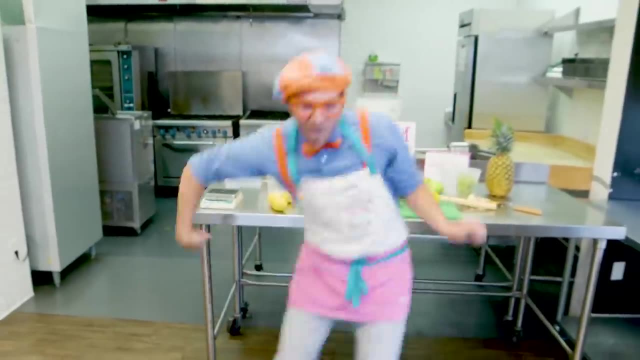 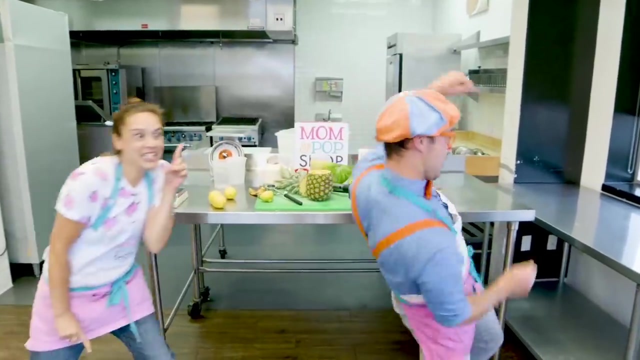 All right now. remember what we had to do earlier. It's gonna take a long time, So we get to dance while we wait. Here we go, Here we go, Here we go. Did I just hear a ding? Woohoo, you sure did. 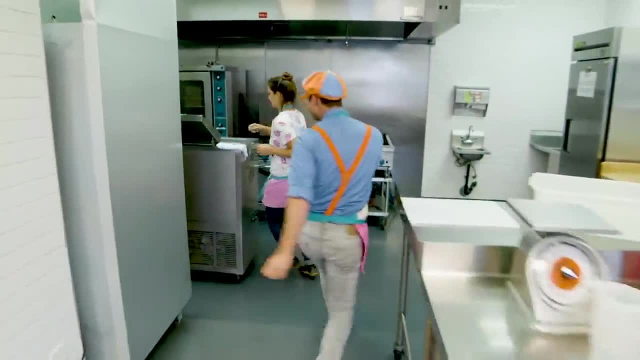 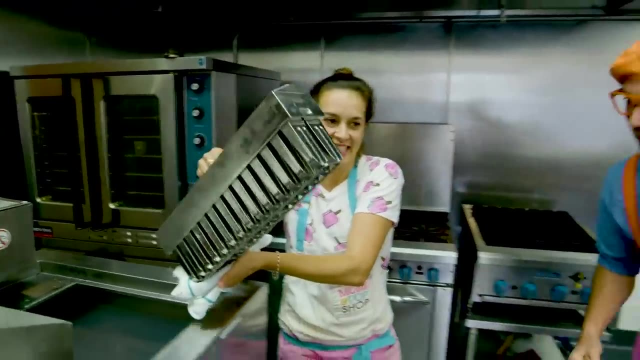 The popsicles must be ready. Let's check them out. Woohoo, All right. Whoa, I am so excited. Hey, we gotta drain them. I can't wait to see the ingredients you used. Oh, me too.